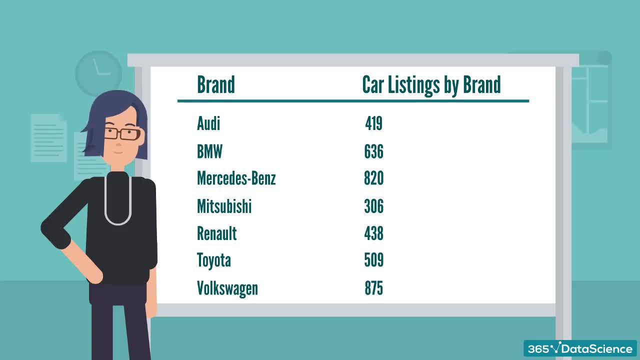 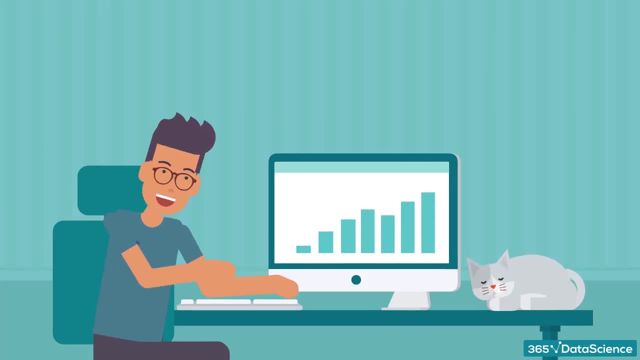 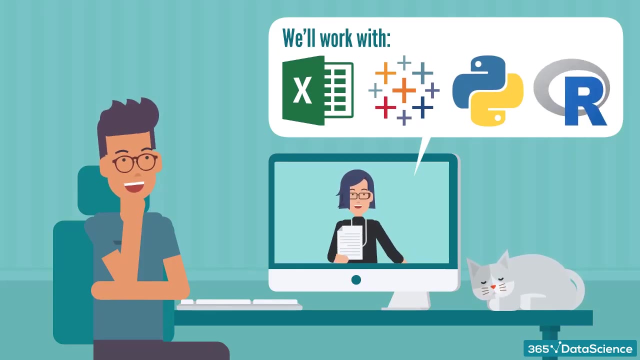 but extremely fitting for an introduction into charts. Rest assured that even if you're a beginner in the field, you'll quickly get used to creating and styling charts. We'll also discover the Excel Tableau, Python and R- built-in functionalities that help you create bar charts with ease. Exciting stuff Can't. 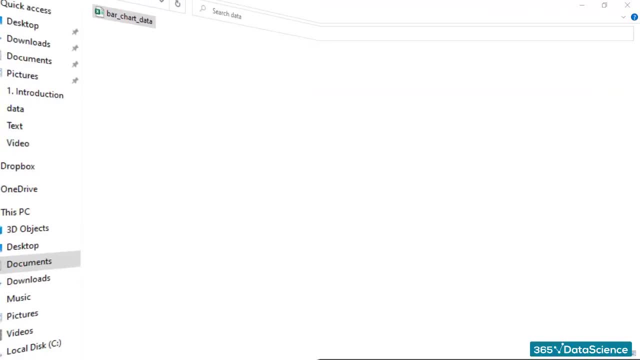 wait to kick off. Here we'll discover how to create and style our charts so they look professional and ready for any presentation. Without further ado. let's get started. We'll go ahead and open our Excel file called Bar Chart Data. 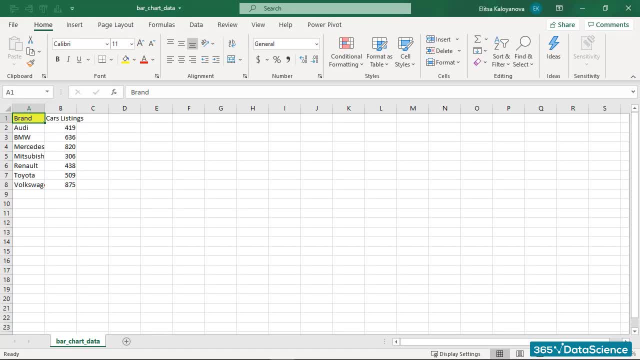 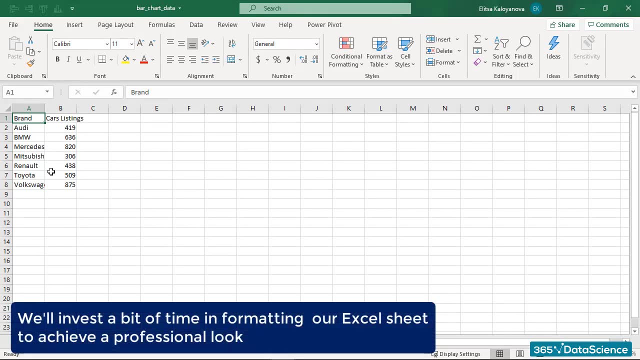 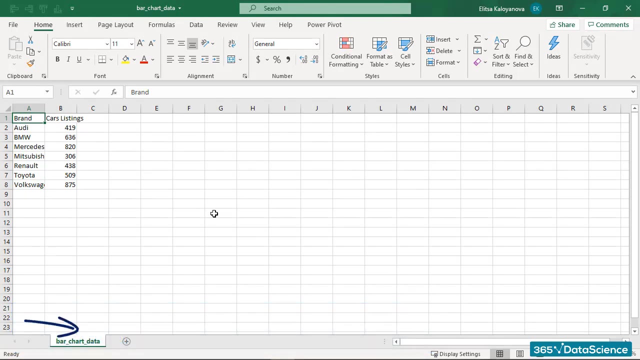 Our data contains the following two columns: Brand and Car Listings. Alright, We'll invest a bit of time in formatting our Excel sheet to achieve a professional look. We'll keep the raw data in this sheet and instead work on our graphic on a separate. 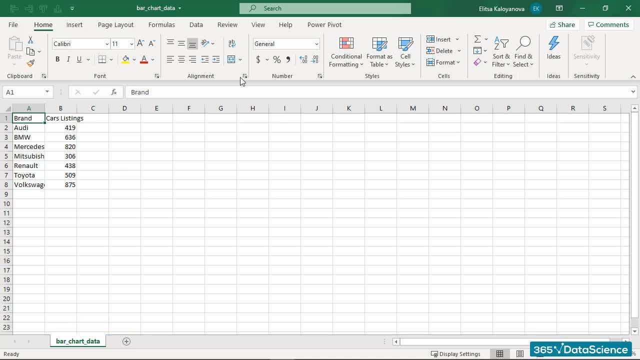 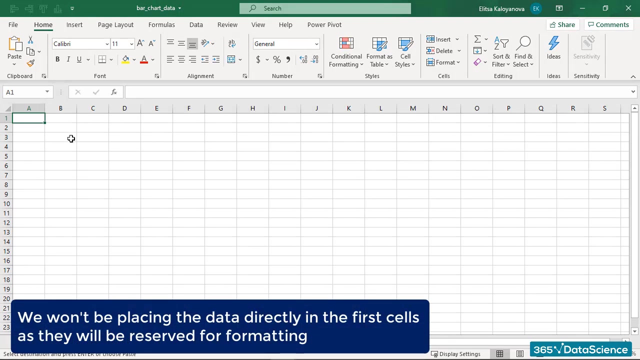 Excel sheet. Let's start by selecting any cell containing data. Then, by pressing Ctrl and A, we can grab all cells from the table. Let's copy them with Ctrl and C and place them onto a new sheet. We won't be placing the data directly into the first cells, as they will be reserved. 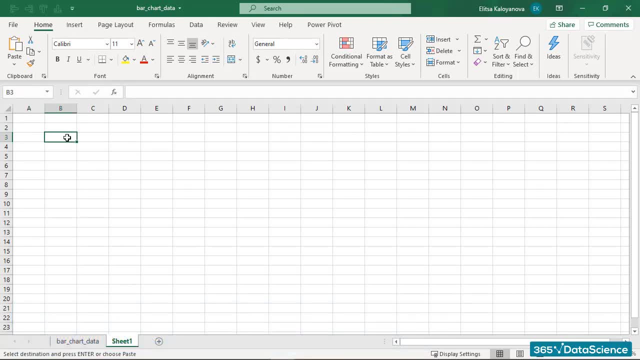 for formatting. Instead, let's select the cell B3 and right-click on it. From the drop-down menu, we choose the first Paste option. Alternatively, you can use the shortcut Ctrl and V to paste the data. So far, not much of a difference, but we're only just beginning. Let's remove the gridlines. 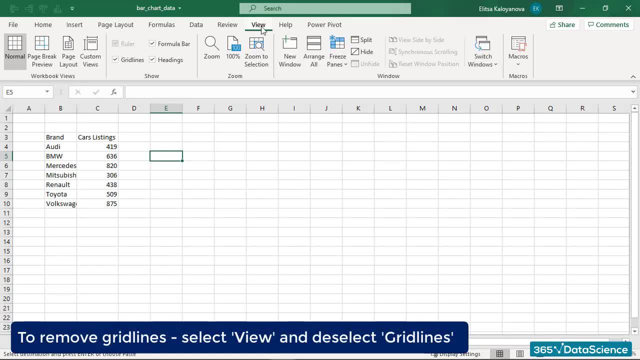 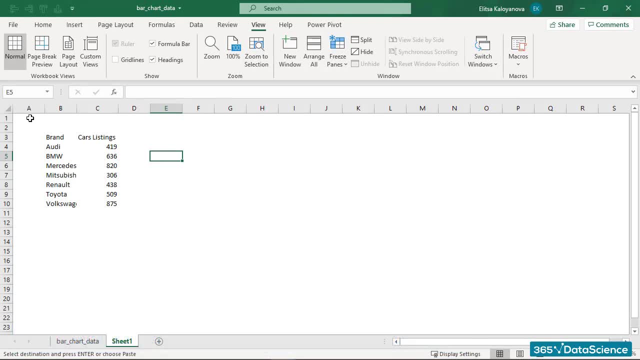 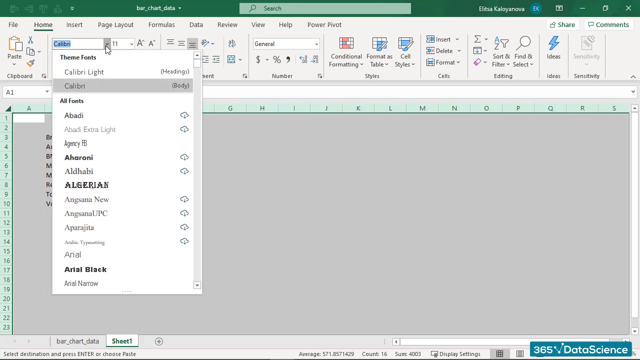 on this sheet. by selecting View, Let's also change the font and font size of our sheet. We'll click on A1 or any empty cell and then press Ctrl and A. This time all cells in our sheet have been selected. Now, from the Home section, we can change the font to Arial and reduce the font size to. 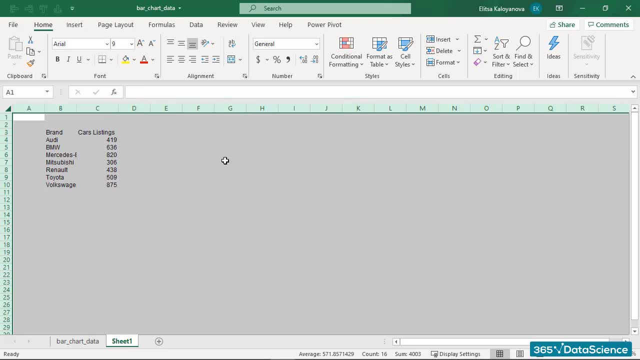 A1.. Okay, The next step is to make the column names more prominent compared to the original ones. We'll click on A1 and then press Ctrl and A. This time all cells in our sheet have been selected. Now from the Home section, we can. 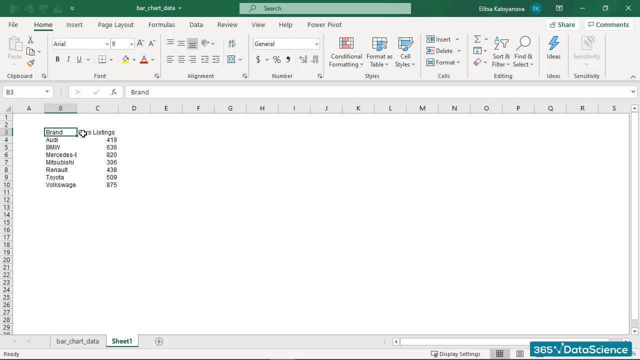 use the shortcut Ctrl and V to paste the data. Let's select cells B3 and C3 and bold them. We'll also click on the gridlines icon and select a thick bottom border. Cool, Let's reduce the width of the A column, as we don't require all that empty space. 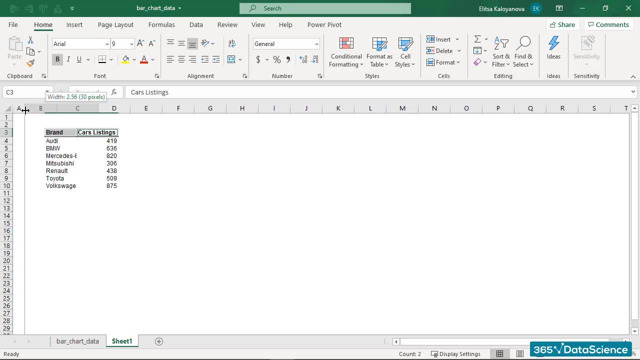 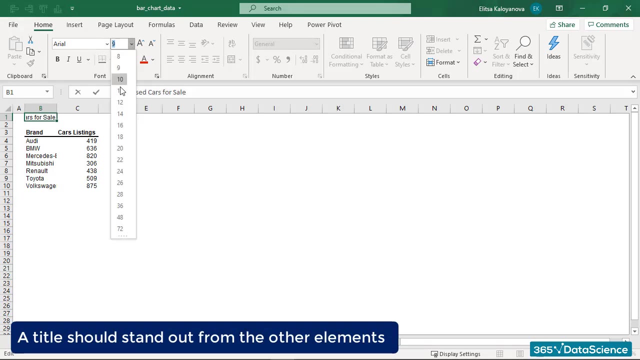 So let's make it around 30 pixels wide. In cell B1, we'll type in a title for our sheet which will be Used Column. Since this is a title, it should stand out from the other elements. We can increase its font size to 12 and bold it. 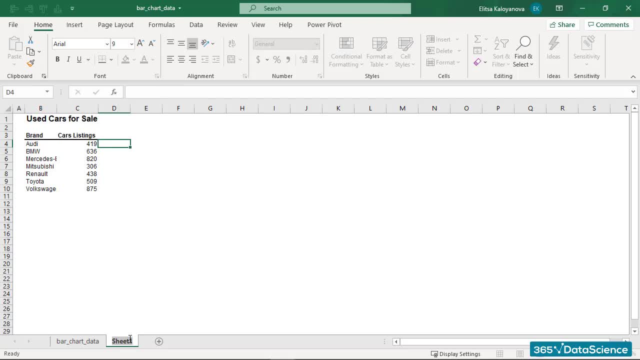 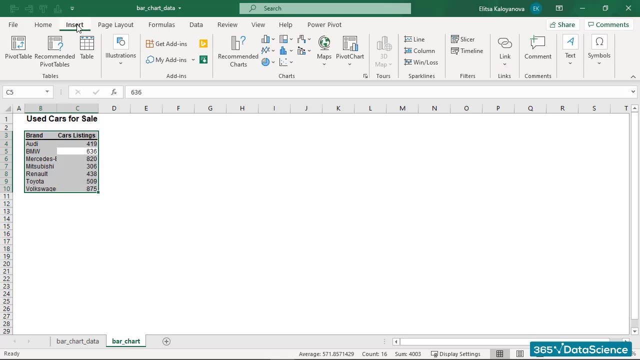 Lastly, let's rename the sheet itself to Bar Chart. Great, Now we can confidently begin creating the actual bar chart. Let's select both columns, Then go to the top ribbon in Excel and click on Insert. The Charts panel has a variety of charts we can use to display our data. 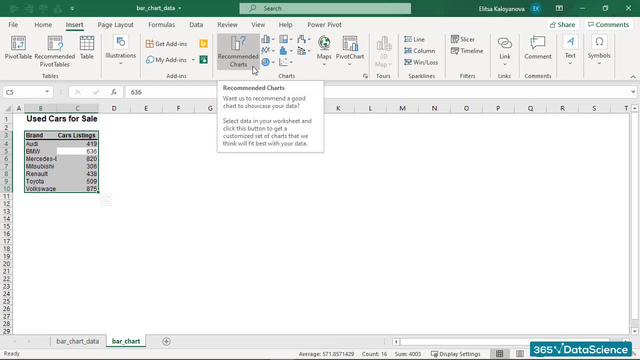 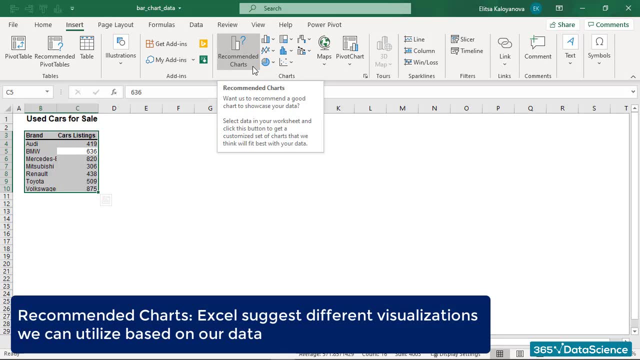 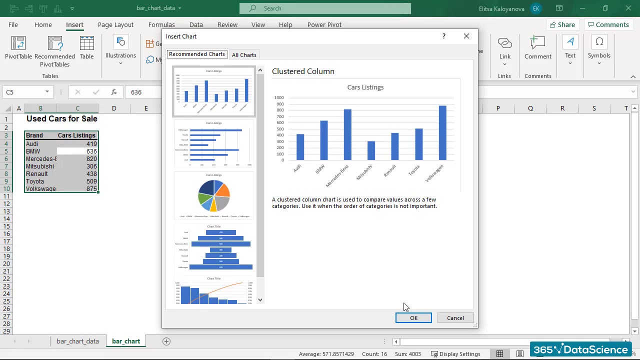 Not only that, but there is also the Recommended Charts section. Through it, Excel suggests different visualizations we can utilize based on our data. Let's try it out, Alright, Perhaps unsurprisingly, the first option we are presented with is a bar chart. 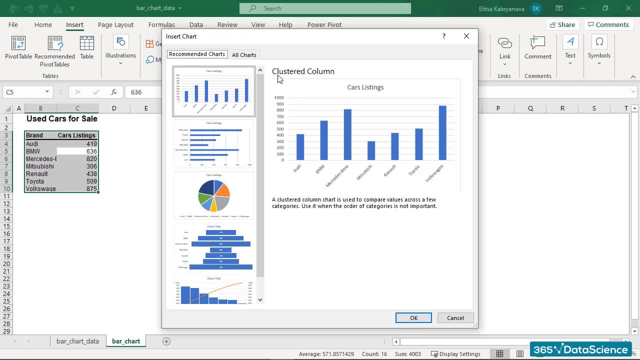 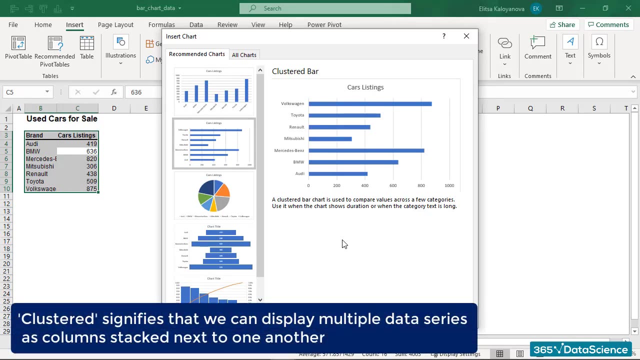 In Excel, this type of chart is referred to as a Clustered Column. The next option is a Horizontal bar chart where the bars are shown horizontally on the Y-axis. In Excel it's Clustered bar. Clustered signifies that we can display multiple data series as columns stacked next to one. 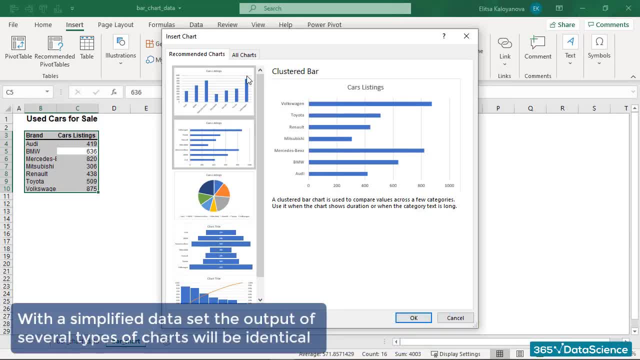 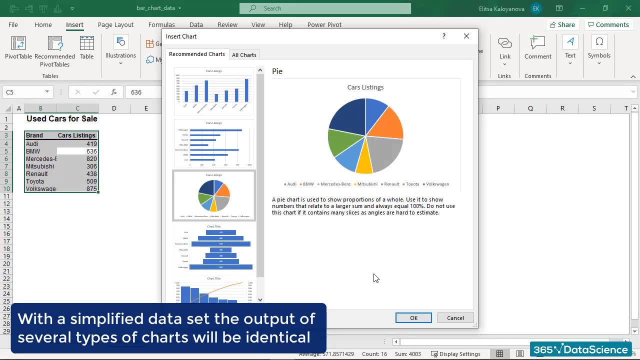 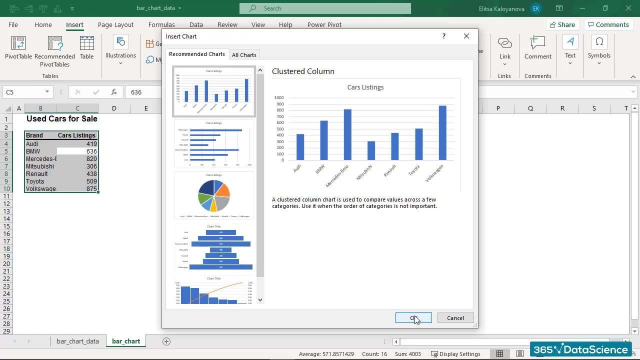 another Note that with a simplified data set such as ours, the output of several different types of charts will be identical. Let's say OK, Either way. for this lecture we'll settle on the basic one, Clustered Column. Then we click OK. 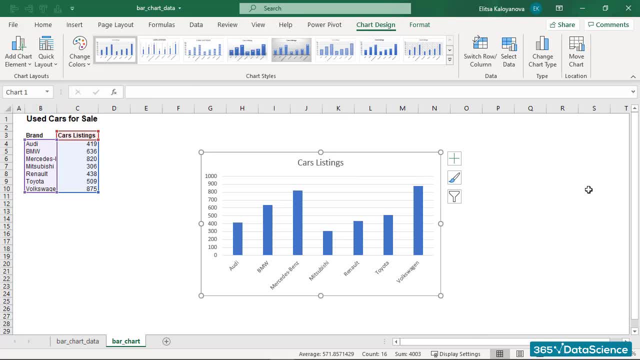 And just with a few clicks we have our chart. It really couldn't be simpler. On the x-axis we have car brands and on the y-axis the number of cars sold. We've got seven columns in total representing the number of used cars sold by each one of. 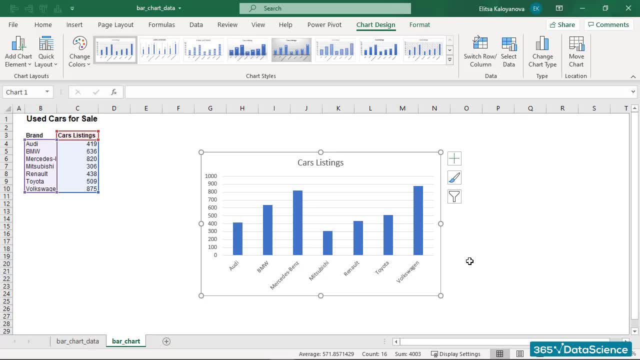 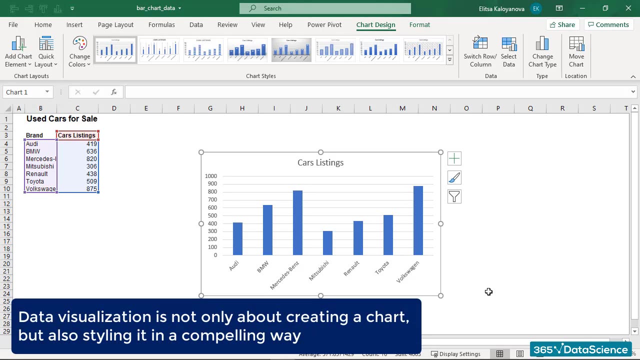 the seven car companies. So far, so good. Now, although this chart is displaying the correct information, we can still improve its appearance. Data visualization is not only about creating a chart, but also styling it in a compelling way. Therefore, let's spend some time on that too. 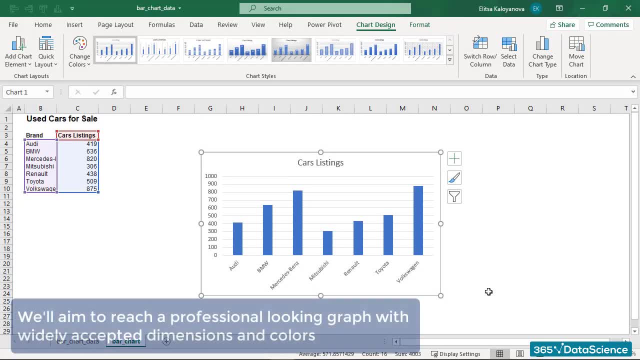 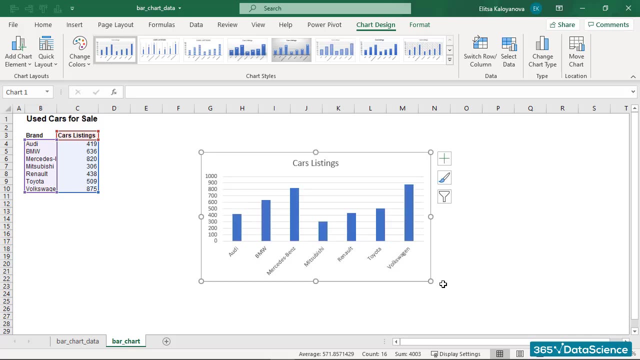 With each visualization we create in this course, we'll aim to reach a professional graph with some widely accepted dimensions and colors. First we'll change the chart size. A chart of this size is optimal for this sheet. The second item on the agenda is to change the font. 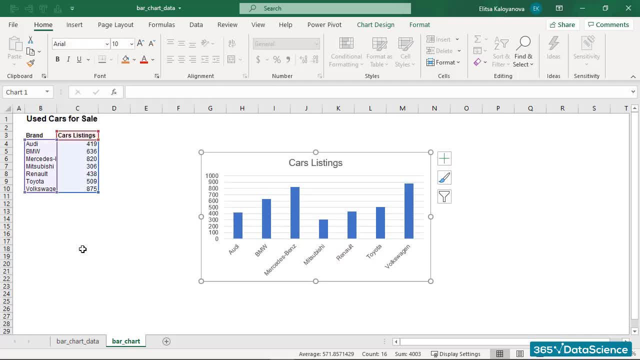 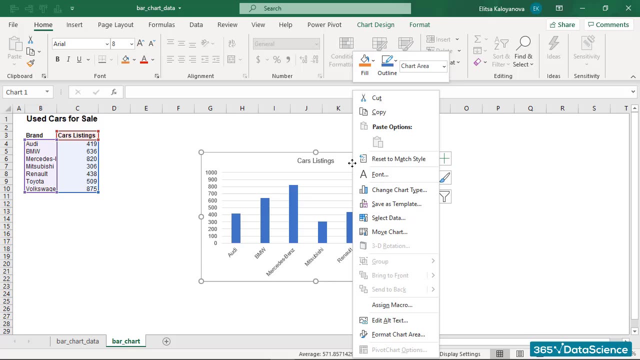 We'll click on the Home button and choose the Arial font. Let's also reduce the font size to 8.. What's next Now? we'd like to remove the fill of the chart and its borderline. Let's left-click on our chart and select Format Chart Area. 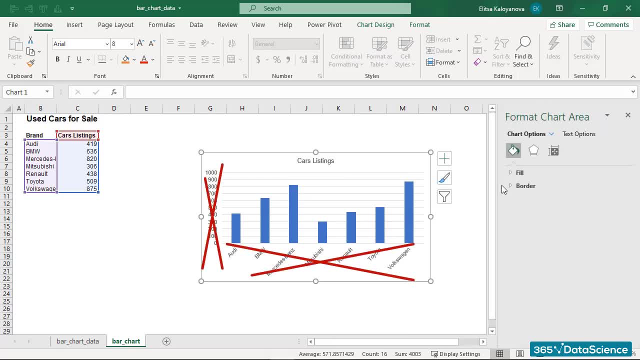 Be careful not to select an element of the charts, such as the plot area or the axis. Okay, From this newly appeared ribbon we can control the fill for the background color or the border for the chart's border. For a professional presentation, clean design works best. 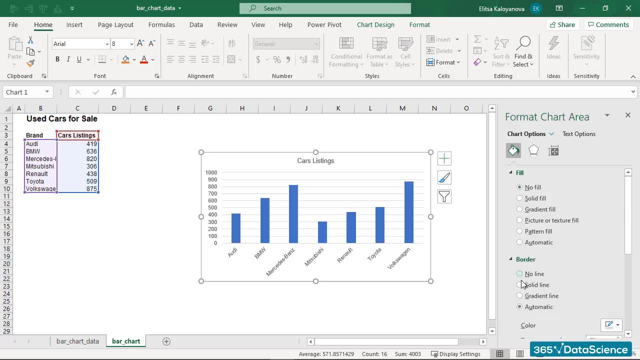 Therefore, our chart will have no fill and no borderline. Alright, We're making great progress. We are now ready to continue with styling specific chart elements. It is only logical we start by focusing on the star of the show, the bars. One idea is to alter their bin size. 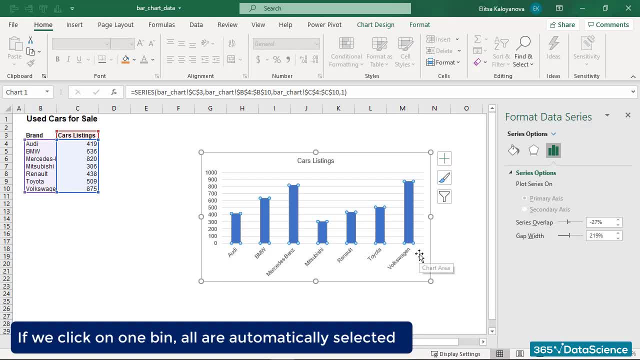 If we click on one of the bins on our chart, it doesn't matter which one- we see that all are automatically selected. Alternatively, if we wish to select only one of the bins in Excel, we need to double-click on it. Okay. 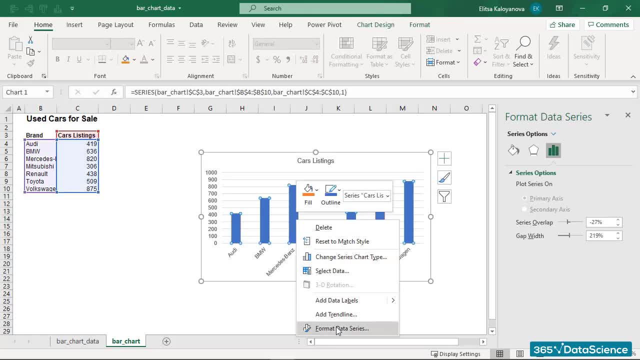 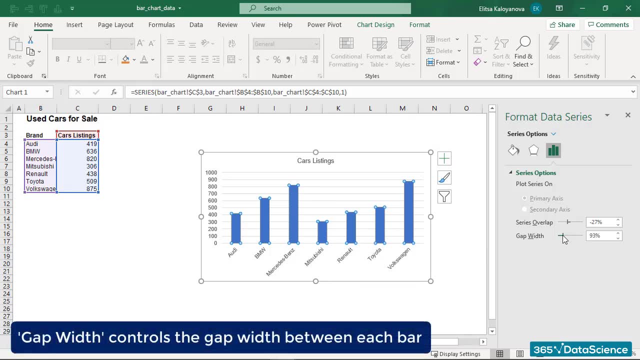 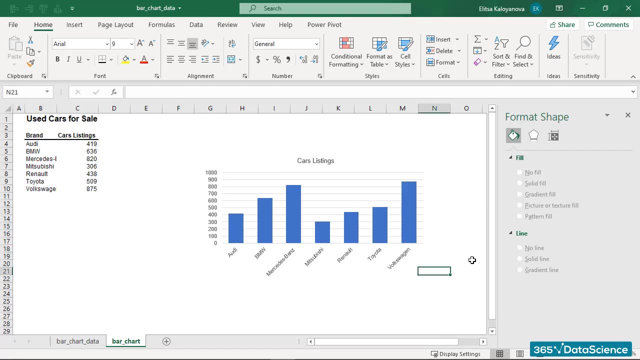 If we right-click on any bin and choose Format Data Series, we'll get a variety of formatting options. Let's reduce the gap between each bar and make it around 95%- Great. What's next? Generally, data visualizations convey insights through shape and color. 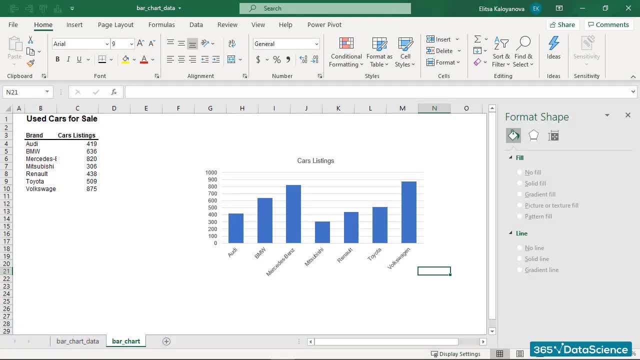 While the shape is somewhat restricted by the nature of the data. the color is up to you. The color is up to us. Choosing a color for our visualizations is of utmost importance and should be thought through carefully. Let's go ahead and pick a nice color for our chart. 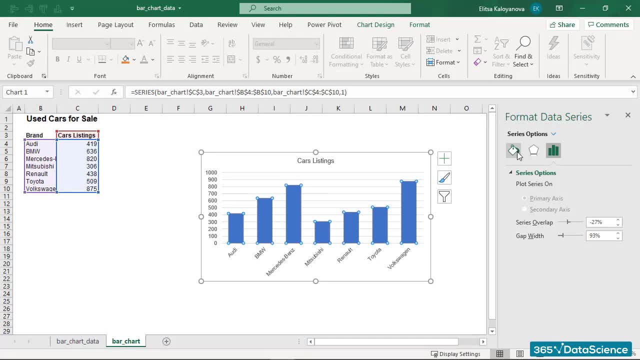 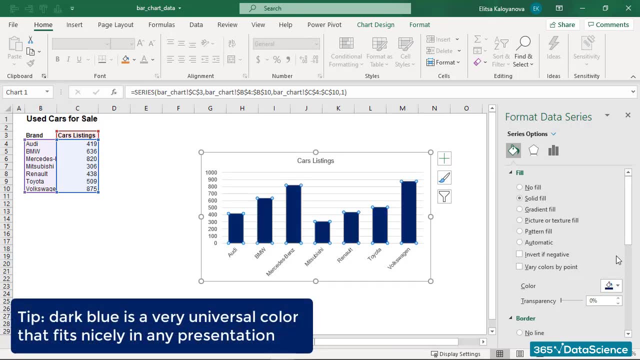 By selecting the first icon in the menu displaying a bucket, we can alter the color to a dark blue. It is a very universal color that fits nicely in any presentation. What else? Currently we can't determine the exact value of each column. 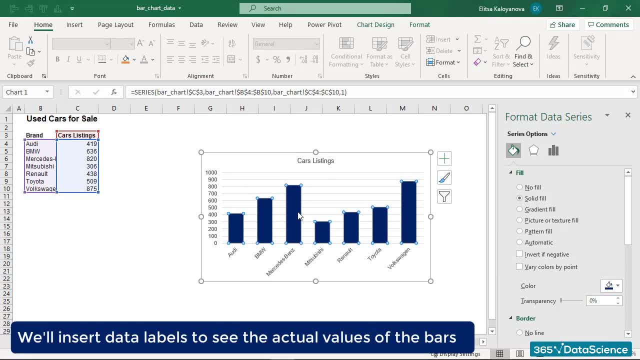 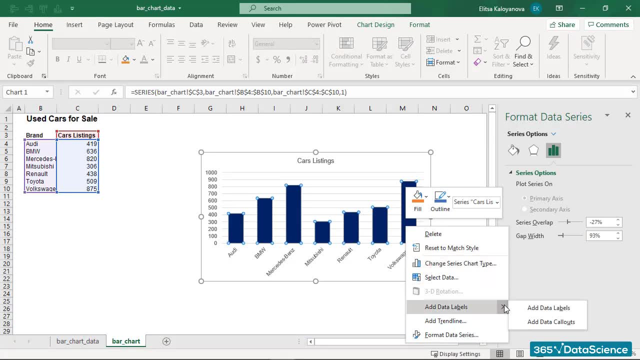 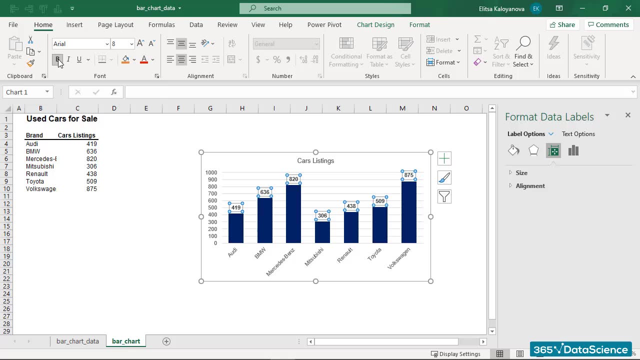 To remedy that, we'll insert data labels. We need to right-click on a series element and opt for Add Data Labels. Let's bold them as well. Cool, We now have the exact amount each company has sold. While we're at it, we should address the Y-axis and add a label there. 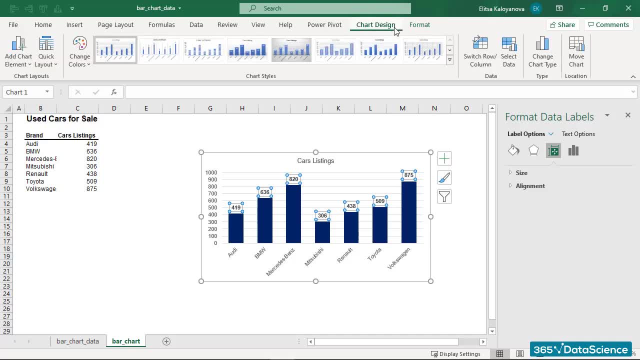 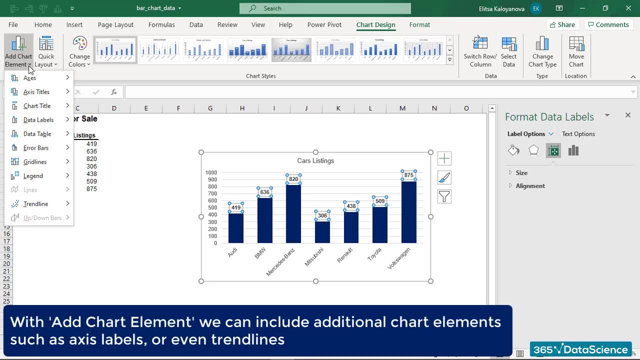 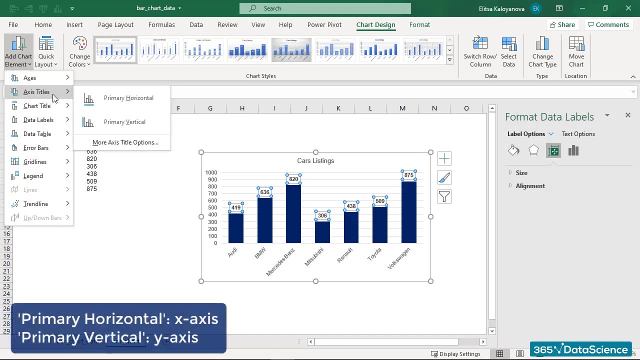 To do so, we select Chart Design from the top Excel ribbon. Here we can select different chart elements. The one we're looking for is a Y-axis label which we add by selecting Axis Title, and then Primary Vertical Horizontal is for the X-axis. 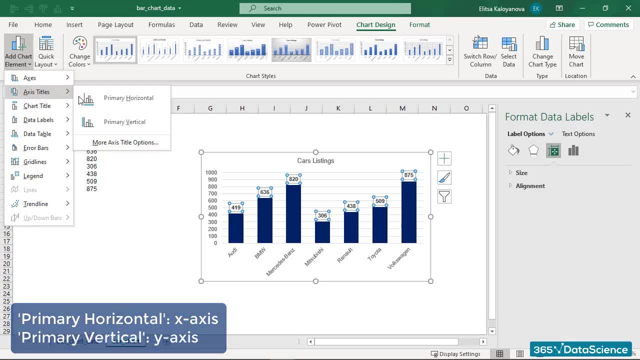 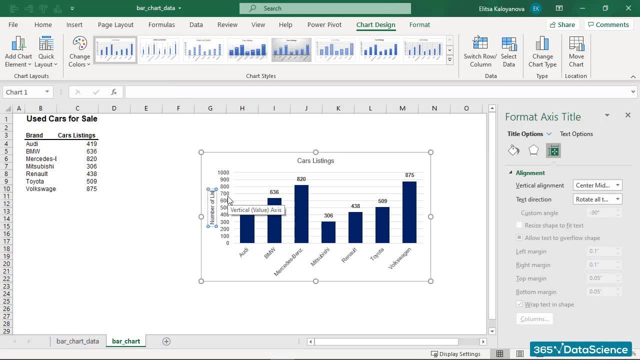 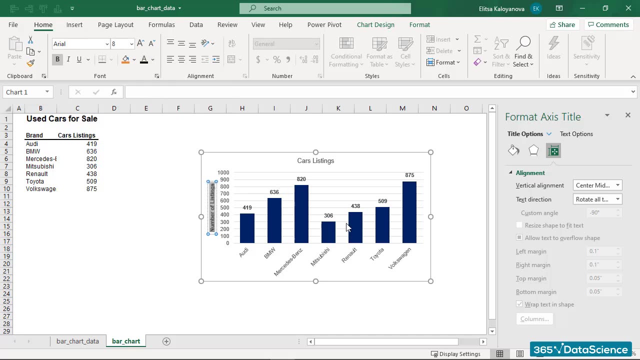 Excellent, Let's name it. Number of Listings and bold it. Make sure the color is actual black. One minor change regarding the Y-axis. The Y-axis ticks are a bit crowded at the moment. Ticks, if you're wondering, refers to the numbers on the axis. 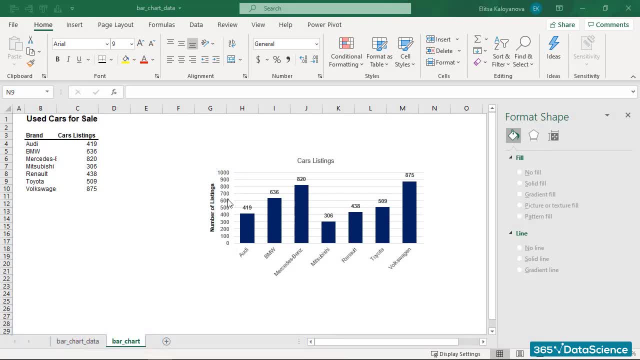 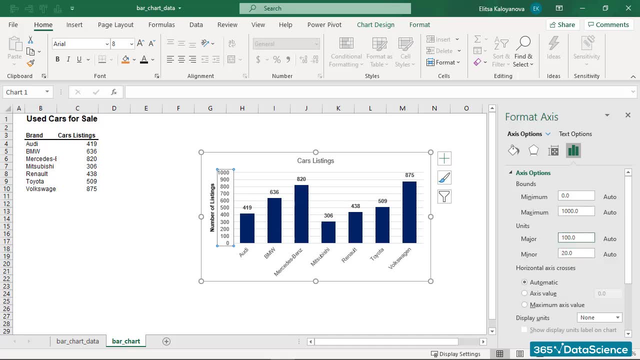 To address the issue. we can add a new label. To address the issue. let's right-click on the axis and select Format Axis. Here, under Units, we can select Major to be 200 instead of 100, thereby halving the number. 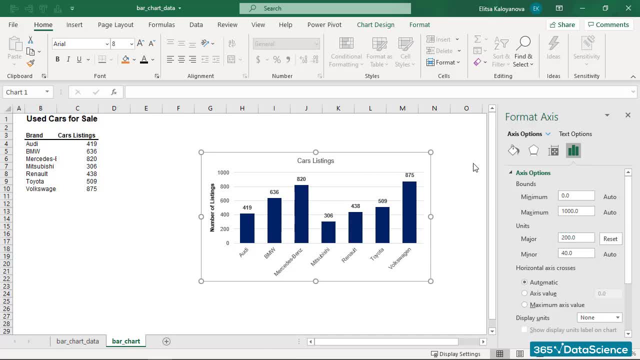 of ticks. Alright, it's time to format the graph's title. Let's double-click on the title area and choose a meaningful title for our chart: Cars Listings by Brand. Again, since this is the title, we want it to stand out, we can select the title we want. 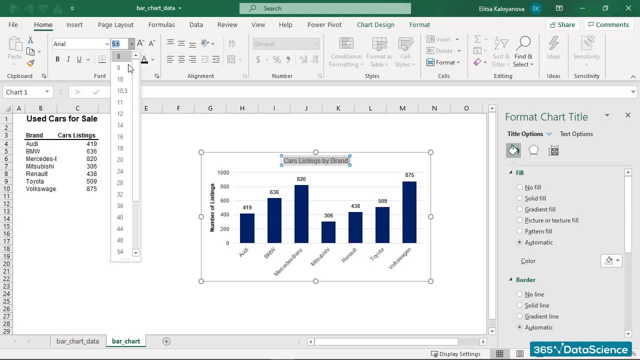 Let's double-click on the title area and choose a meaningful title for our chart Cars Listings by Brand. Here under Units, we can select the title we want it to stand out. On that account, we'll increase the font size to 12 and also have it in bold. 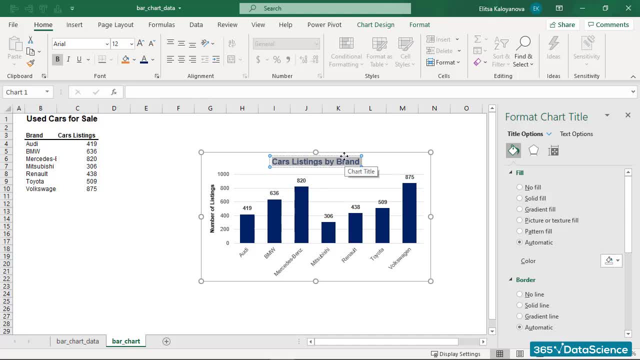 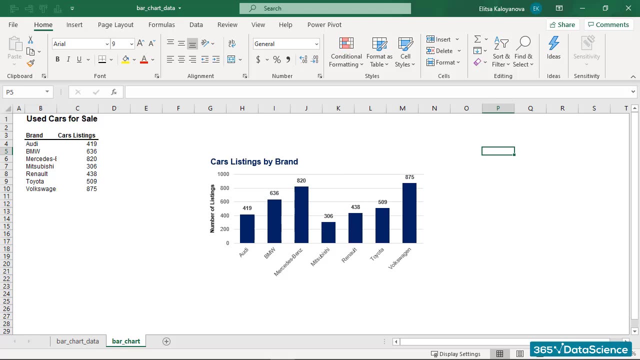 For this particular chart, aligning the title on the left-hand side of the visual is a good option. Great, Now our chart is ready. It not only displays the relevant information, but also looks professional. The last remaining step is to save our work. 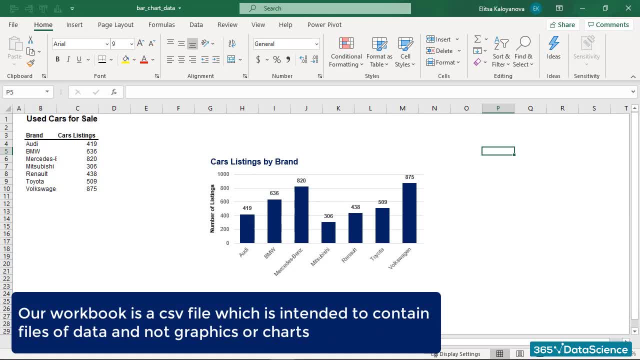 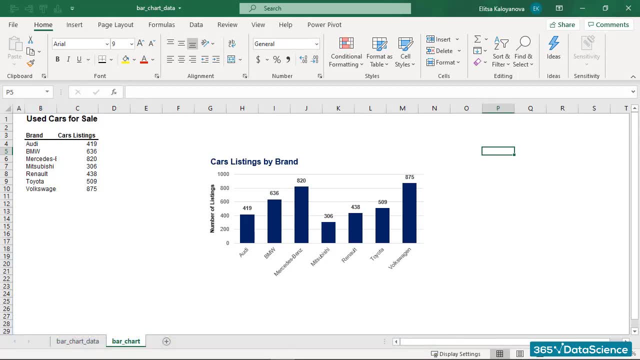 Currently, our workbook is a CSV file. Let's save our workbook CSV file, which is intended to contain files of data and not graphics or charts. If we close Excel right now and reopen it, our chart will disappear and will not be saved. 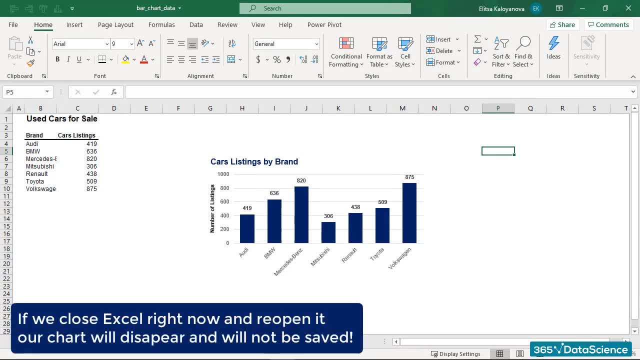 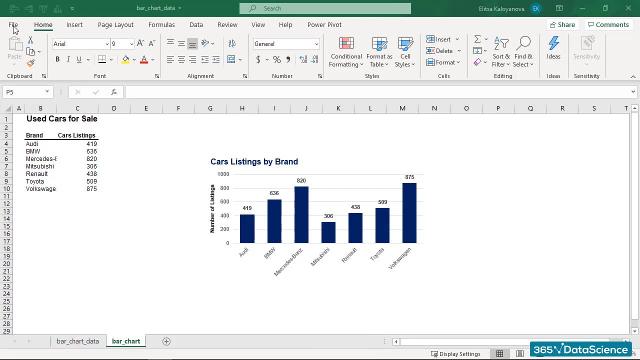 This is extremely important, so I'll repeat that If we close Excel right now and reopen it, our chart will disappear and will not be saved. Therefore, it is crucial to save our file under a different extension. Let's go to File and Save As. 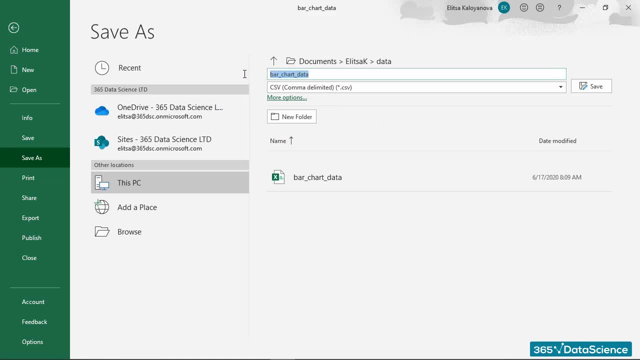 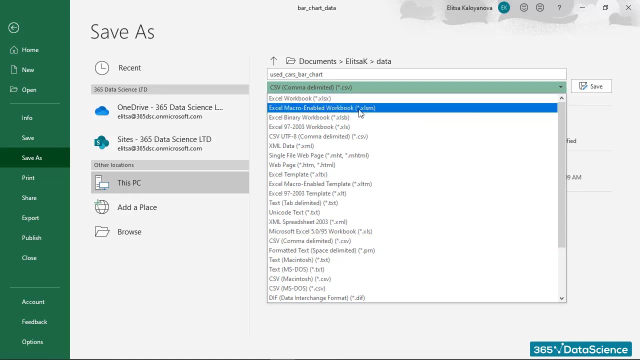 In the first box we'll type in the name of the file. In our case it will be Used Cars Bar Chart. When we select the second box, a drop-down menu appears showing us the different extension files which Excel supports. We'll opt for an Excel workbook under the extension xlsx. 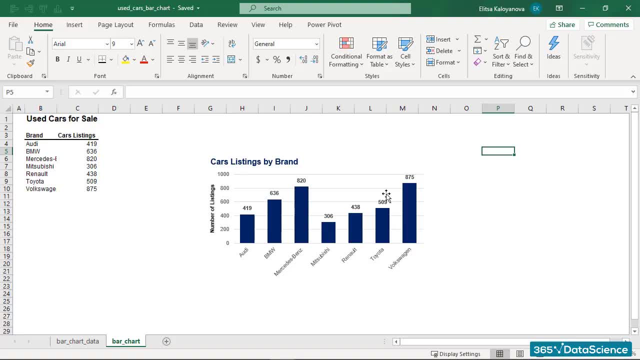 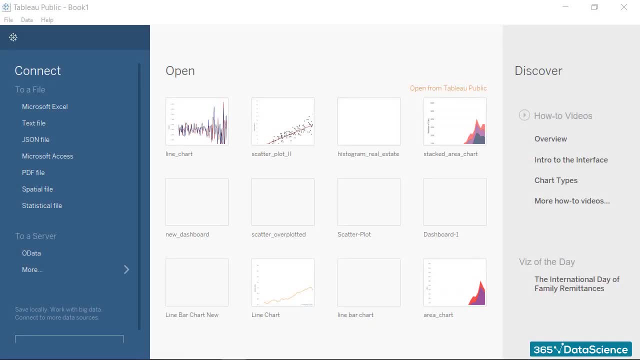 And hit the Save button. Good job everyone. we've successfully created our first bar chart in Excel. Here we'll get familiar with the Tableau interface and use its capabilities to make and style our very own bar chart. Let's get started. The first thing we'll need to do is connect to our data source. 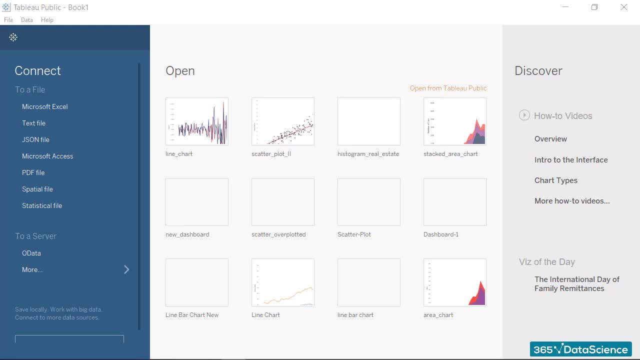 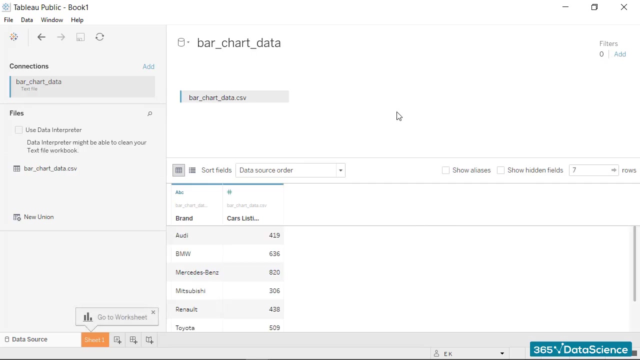 In our case, we have our car data in a text file with the extension csv. Alright, Let's start. Let's select the Connect to a text file option and choose the file: bar chart data, csv. Okay, In this area of Tableau we can explore the data set. 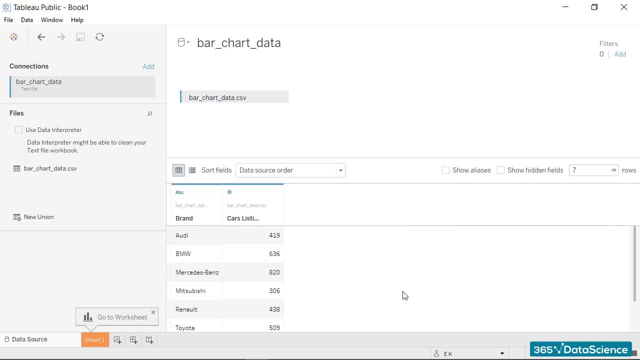 We can join columns together or filter the data, But this data set is really small, so we won't spend a lot of time here. yet Tableau is quite intuitive and beginner friendly, Therefore, we might as well follow its instructions in this pop-up suggesting that we want to. 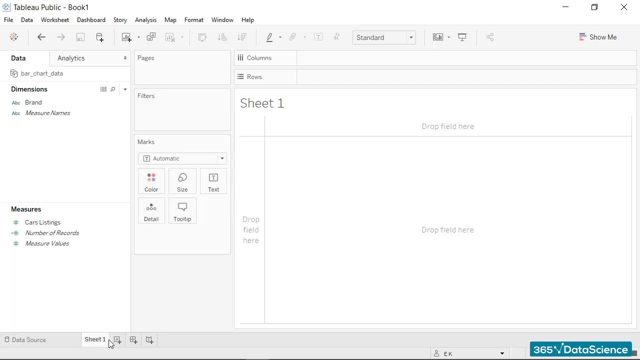 use tableau in the future. As you can see, tableau is one of the most common use cases for a workbook, So we'll be using tableau to organize our workbook. Let's click on tableau And we can see that we have a tableau chart that we've created. 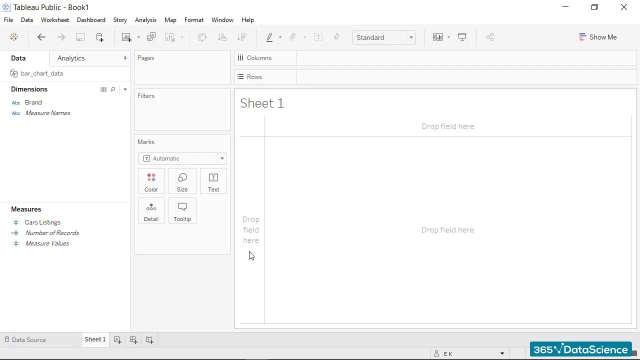 As you can see, we've created a worksheet. Now we can see that tableau is a tableau chart. Let's go to the worksheet. Let's click on sheet 1.. Alright, We blindly followed Tableau's lead and ended up in sheet 1.. 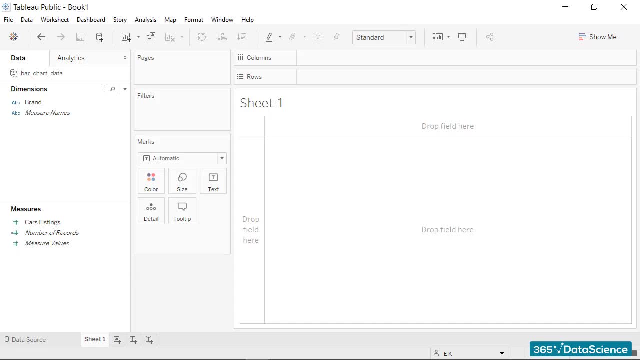 Now, before we go any further, let's spend a second to discuss how Tableau is organized and why it makes sense to be here. Tableau uses a structure with workbooks and sheets. This whole area is known as a workbook. A workbook can contain three different types of sheets. 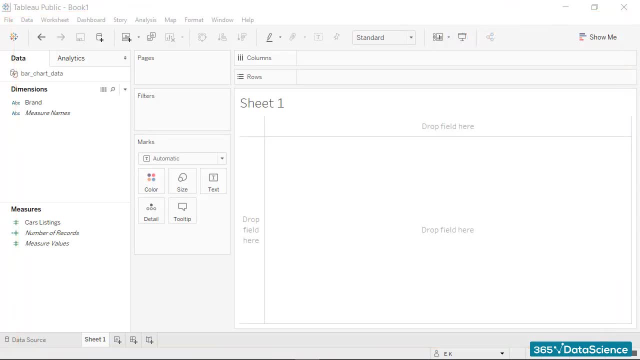 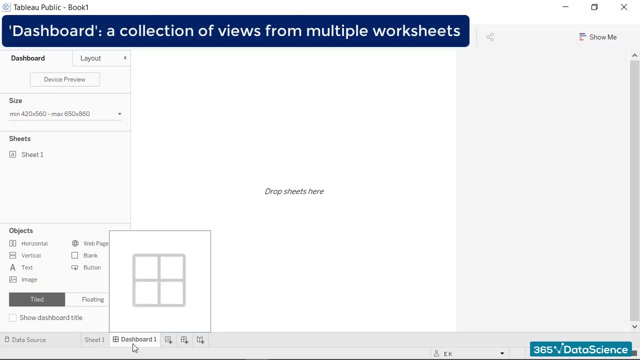 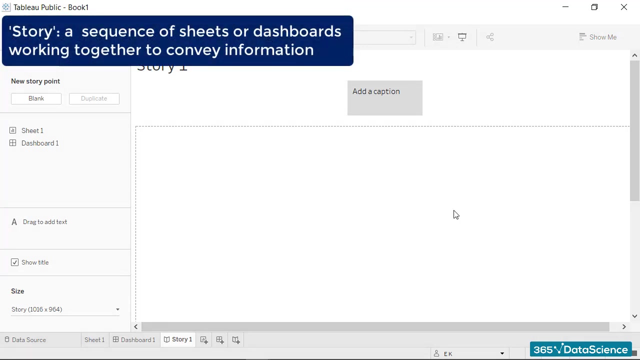 A workbook can contain three different types of sheets. The first type of sheet is a worksheet – a single view containing shelves, cards, legends, data and analytics panels. The second type is a dashboard – a collection of views from multiple worksheets. And, lastly, a sheet can be a story, which is a sequence of worksheets or dashboards. 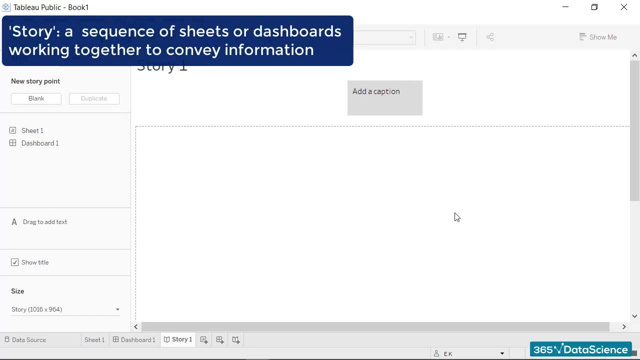 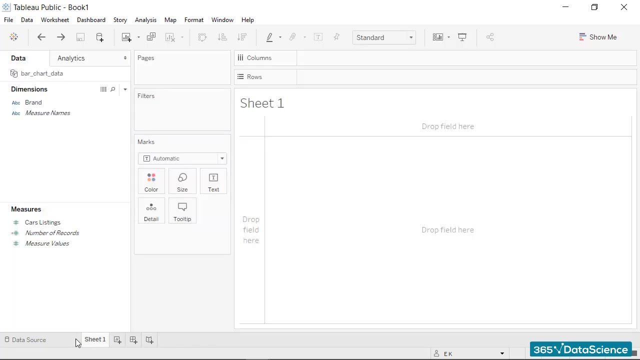 working together to convey information In Tableau. we have easy access to all three through the ribbon at the bottom part of the workbook. For now we'll be creating with a worksheet, but as we progress through the course we'll also learn how to create dashboards. 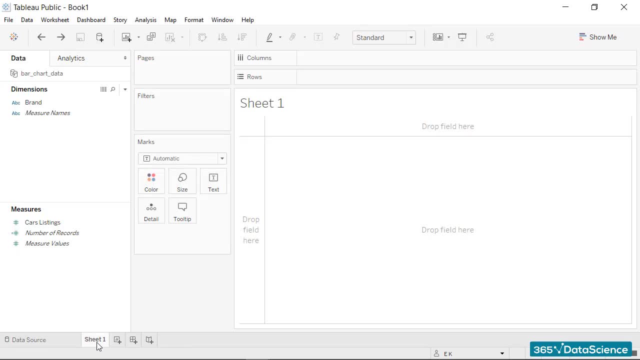 Cool. what else? The panel you see here is a worksheet. Here on the left is the data panel. In Tableau, data is categorized as either a dimension or a measure, So each column in our data will be placed in one of the two categories. 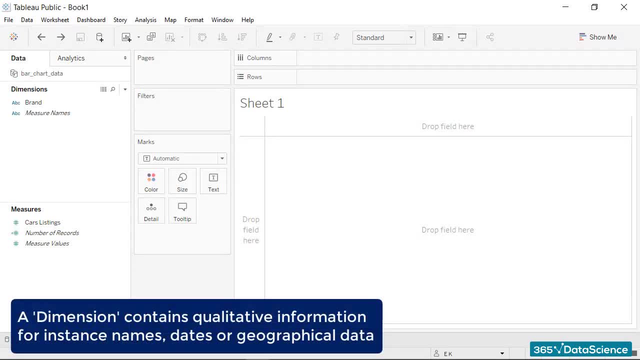 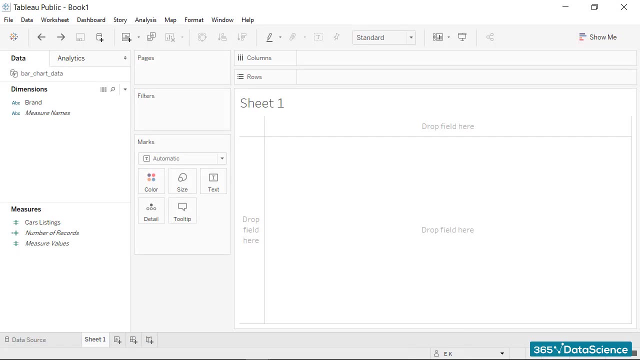 A dimension contains qualitative information – for instance, names, dates or geographical data. A measure, on the other hand, represents quantitative, numeric information. Tableau automatically sorts the variables into the bins and is usually very good at doing so. If we double-click on car listings and then on brand, we see that we get a bar chart straight. 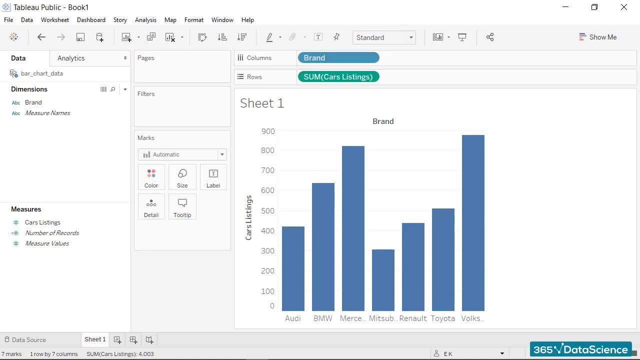 away. Obviously, Tableau has figured out a way to visually represent our data, And this is what is so great about Tableau – it is extremely good at guessing our visualization intentions. That could be the end of the lecture, But things are not always as easy as they seem. 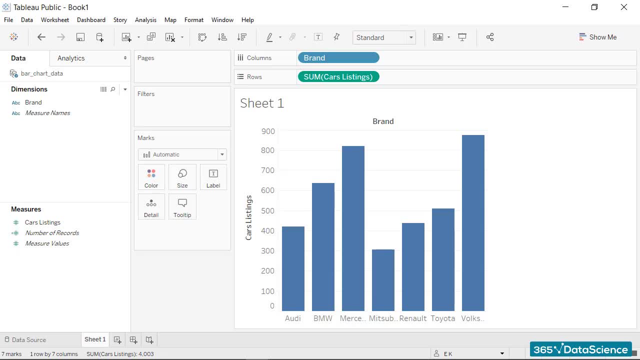 Tableau is a great tool for visualizing. It's that perfect. That's why Tableau also allows us to manually select chart types. There are two ways to do this. The first one is to choose an option from the Marks panel. If we click on Automatic, a drop-down menu with options appears. 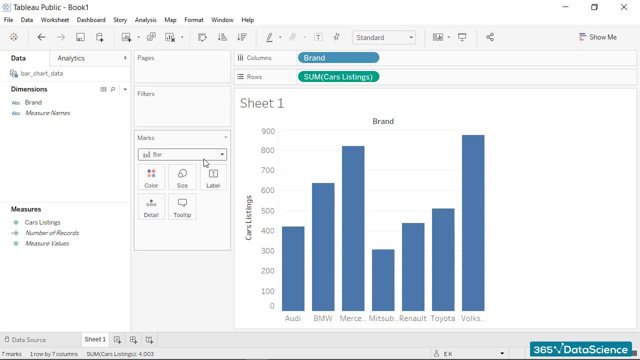 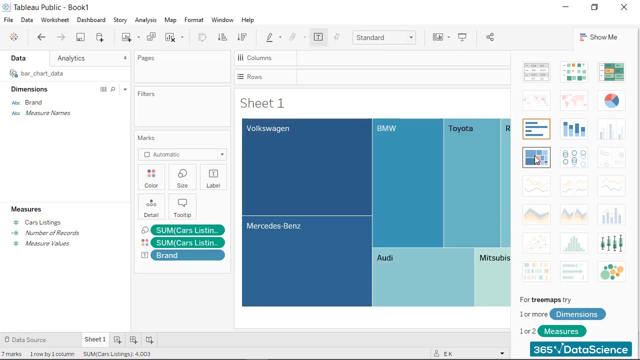 Let's select Bar. Alternatively, on the right-hand side of the worksheet, we have a Show Me field with different visualization options. For example… We can select a pie chart or a tree map. Some of the options are unavailable at the moment because of the nature of our data. 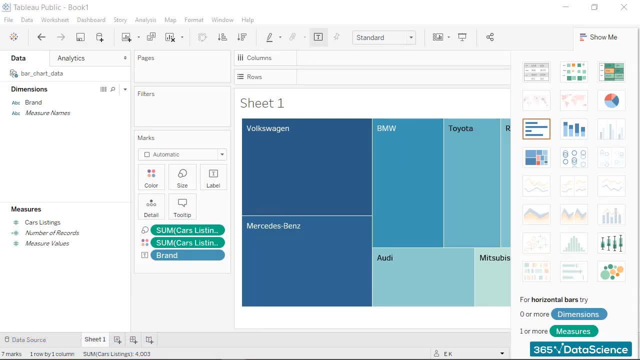 Not all data could be represented with all charts. For instance, if we hover over the map, we see that we need a geographical dimension, which we do not have. Or if we go to Histogram Tableau prompts that a histogram requires precise measurement. 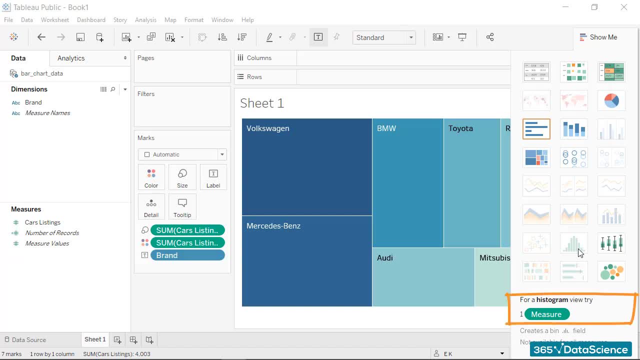 For instance, if we hover over the map, we see that we need a geographical dimension, which we do not have. Or if we hover over the map, we see that we need a geographical dimension which we do not have. Or if we hover over the map, we see that we need a geographical dimension which requires. 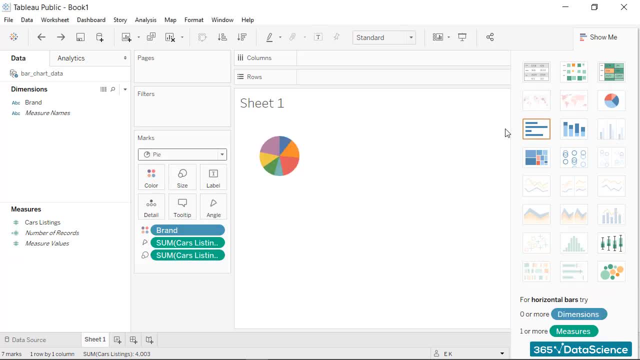 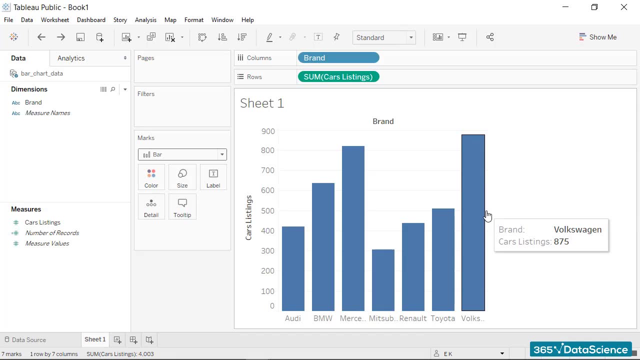 precise measurement. OK, let's stick to a bar chart for now and try out some of Tableau's styling capabilities to improve its appearance. The first thing we'll do is to enlarge the plot to make all the labels on the X-axis visible. 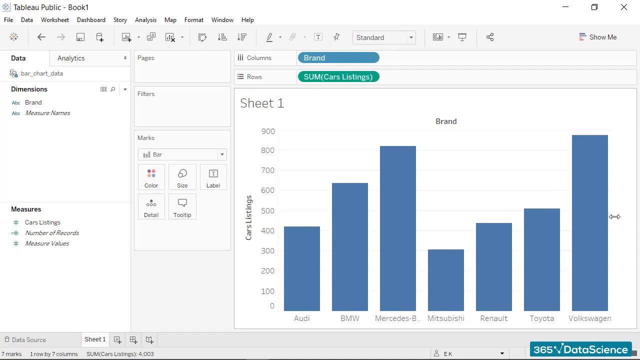 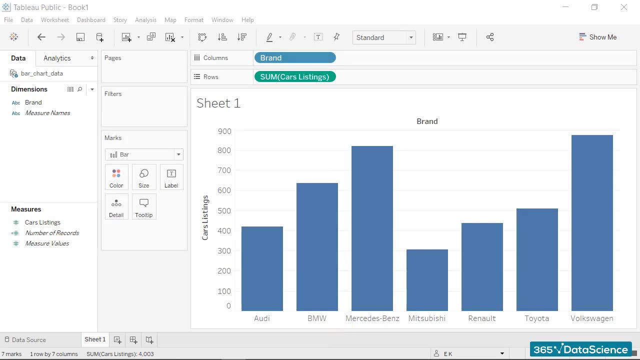 We'll just extend it to the right until we can read the Mercedes-Benz label: What's next? Wow. Generally, data visualizations convey insights through shape and color. While the shape is somewhat restricted by the nature of the data, the color is up to. 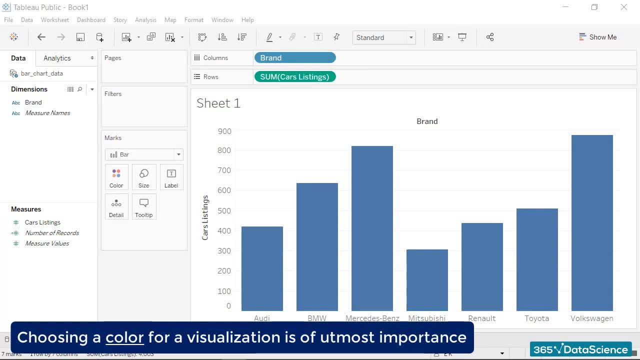 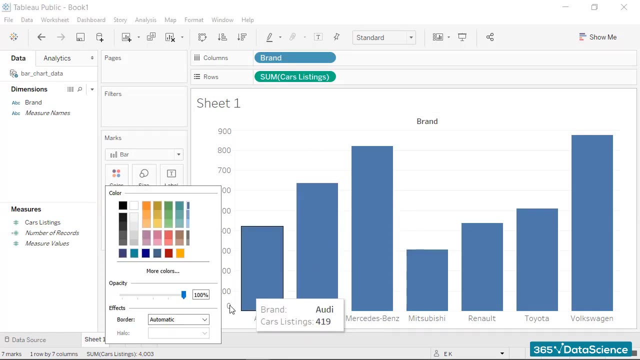 us. Nonetheless, choosing a color for our visualizations is of utmost importance and should be thought through carefully. In Tableau, color can be altered through the color mark. We click on it and a panel appears allowing us to choose a color for our bars and modify. 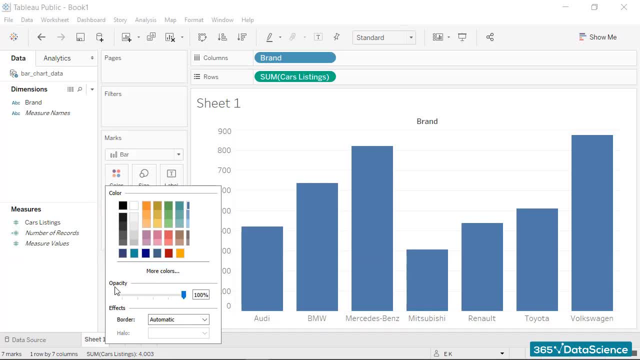 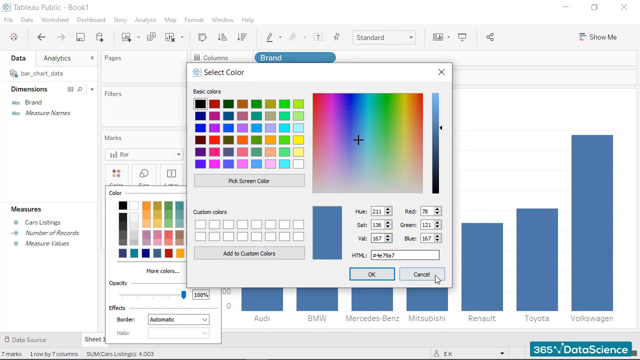 the opacity level. In case you are wondering, opacity controls the transparency of the color elements. Through the More Colors option, we can select a custom color for our chart. So far, so good. The color element is a component of the Marks panel, which in turn, is an integral part of. 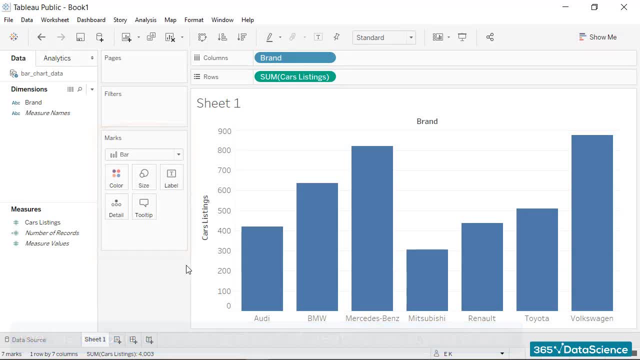 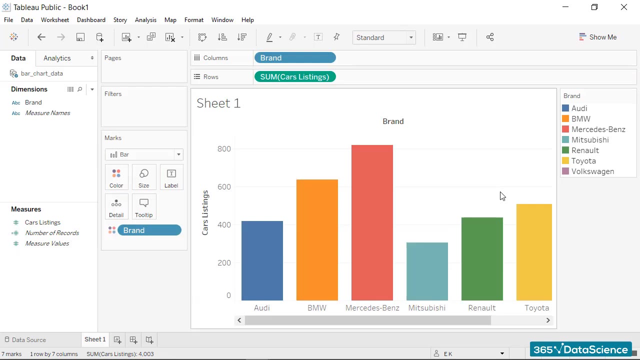 creating and styling charts. Marks allow us to change and add details to our charts. but there is another neat application of Marks. Let's check it out. From the Data pane we'll select Brand and drag it into the color square. See. 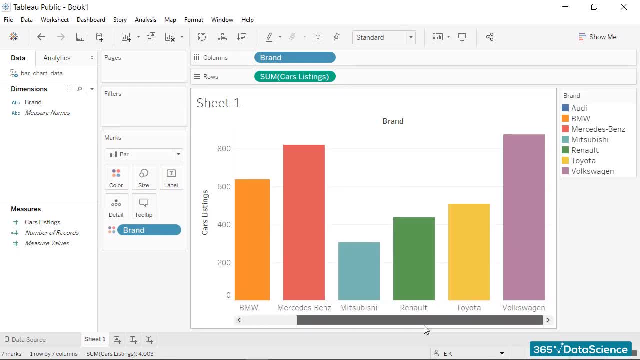 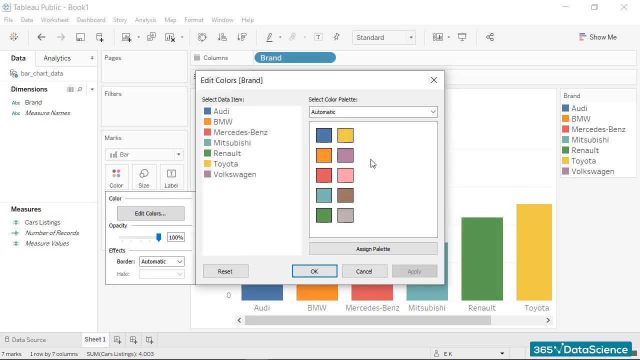 Tableau colors our plot by the individual brand straight away Great. Now, when we left-click on Color and then on Edit Colors instead of individual colors, we are given the option of different color palettes. Let's check it out: Selecting Automatic, we observe 20 or so options. 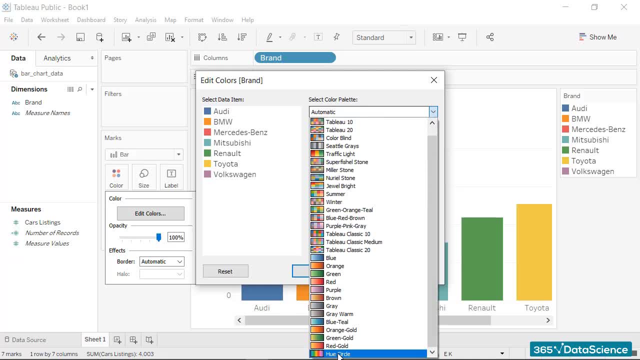 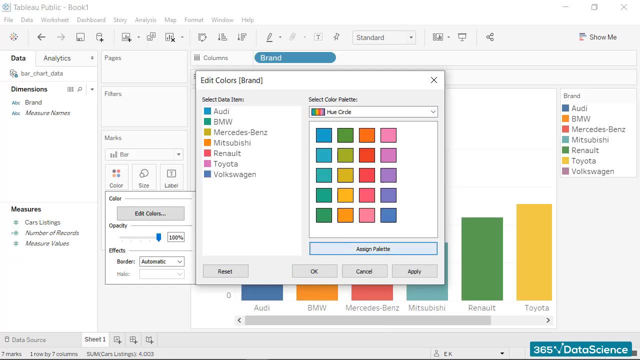 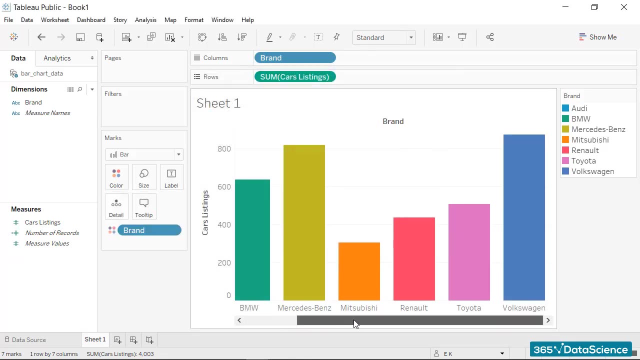 Let's check out Hue Circle, for instance. Once we've landed on a palette, we click on Assign Palette and then on Apply. This sets it as the new color palette for the graph. Feel free to explore the other options on your own after the lecture. 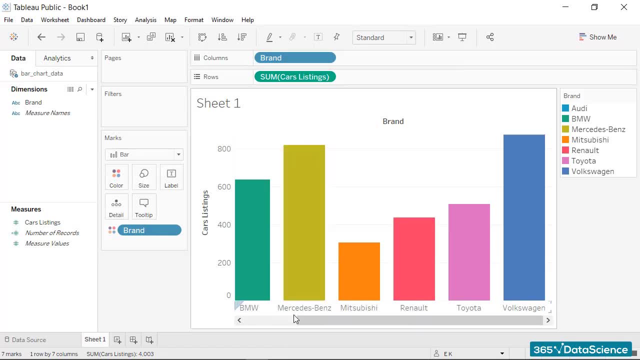 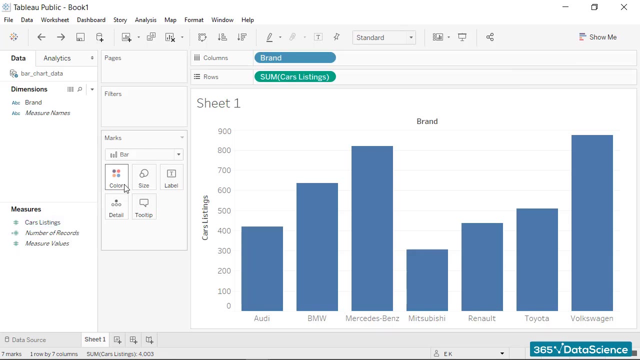 Great. There are tons of styling options available with the Marks panel. We'll be exploring those throughout the course. For our graph, though, let's revert to a single color. with Control-Z To make sure our graph is professional, we can choose a dark blue color. 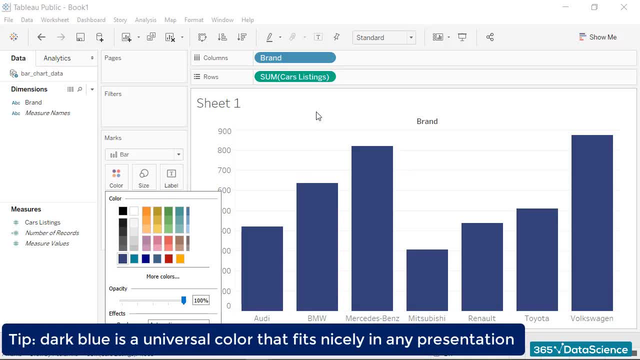 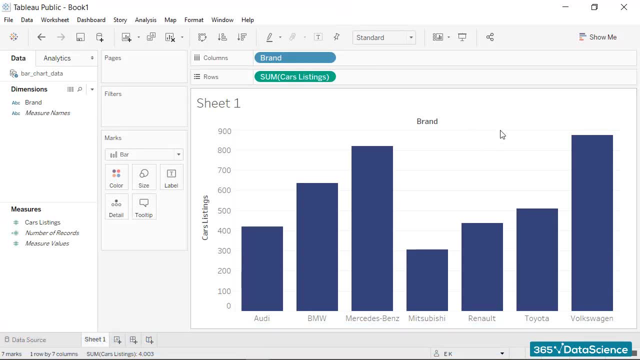 It is a very universal color and would fit nicely in any presentation. Brilliant, We're well on our way to making an awesome chart. Now let's direct our attention to the bars and their height. We can see that the bars and their height are the same. 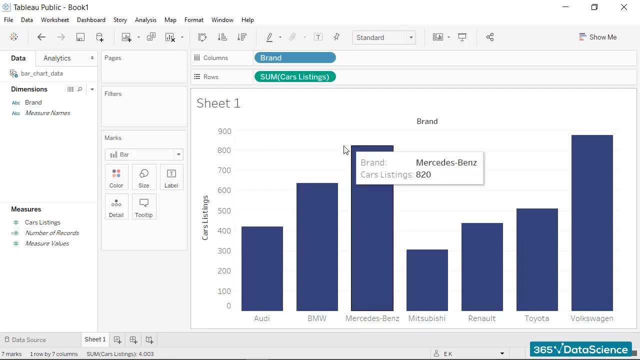 We can see that the bars and their height are the same. The width of the bars and their height are the same, But if we were to scale on the x axis, it isn't very precise In this case. the bar we are just barring makes it hard to adjust this supply. 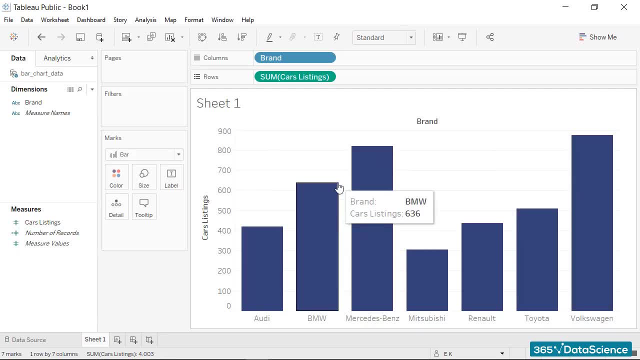 So, then, we relies on this thinner testing bar, which lets us scale on the x axis. That makes gauging the accurate value for each bar difficult. If we were comparing the ads between Audi and Renault, for instance, he has to squint. 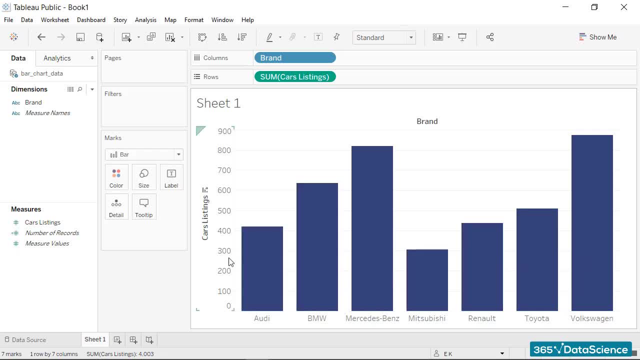 to find out that Renault is ahead of the example. To display the number of car listings of each brand, we'll add labels. And yet another instance where we'll make use of the Marks panel: We'll drag the cars measure into the Labels field. 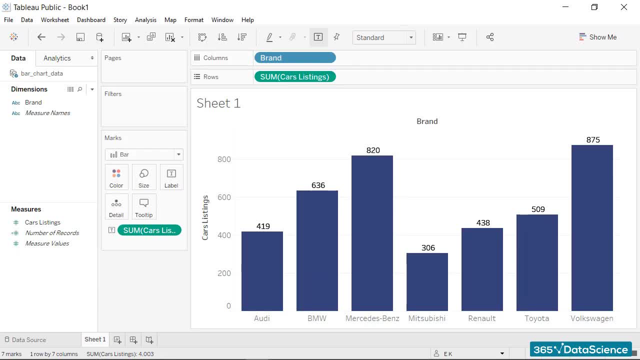 Labels field. and voila, Labels for each bar have appeared Superb. Next we'll focus on the text in our graph. We'll start by changing the font. Tableau allows for font formatting on different levels. We can format a particular axis or individual. 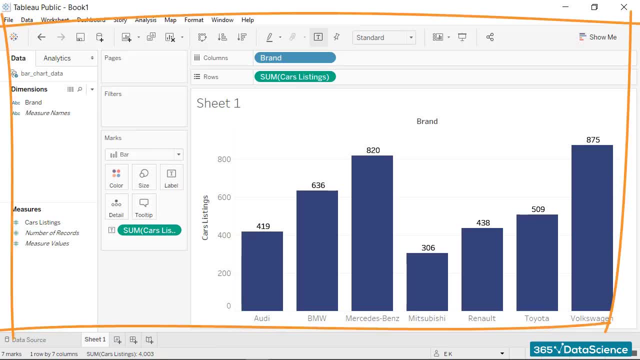 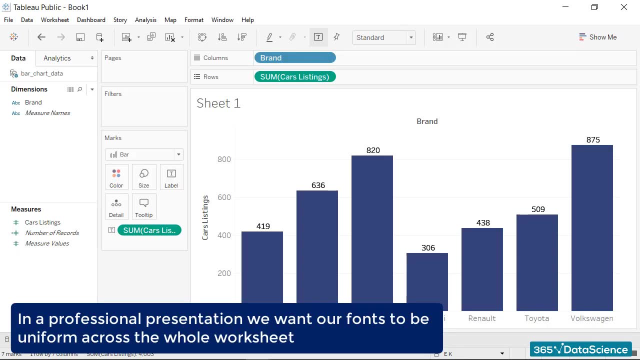 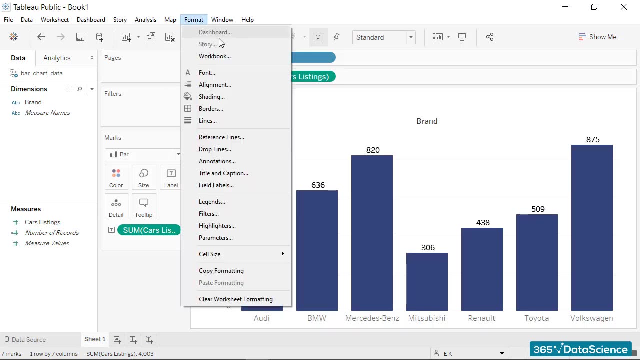 label or generally format the appearance of the entire workbook In a professional presentation. we want our fonts to be uniform across the whole worksheet. Therefore we'll opt for the last option. From the top menu page we'll select Format and then Workbook. Let's go for a pretty standard font like: 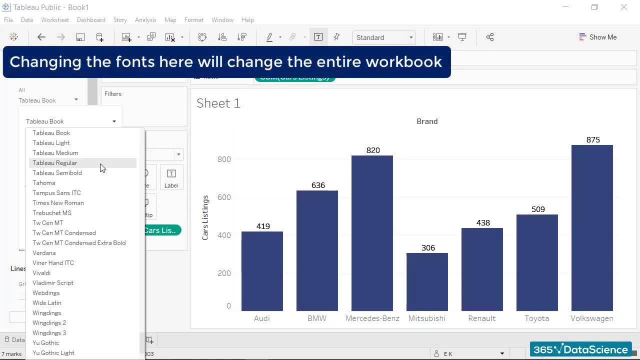 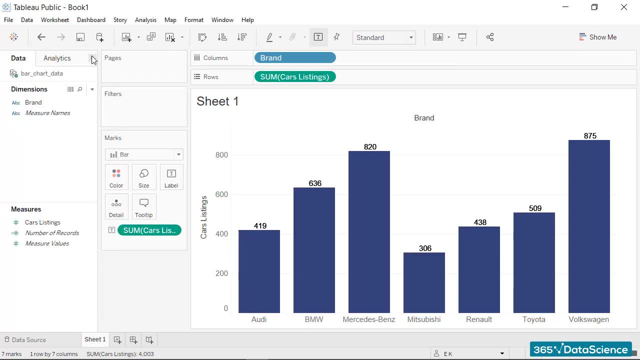 Arial. Once we change it here, we'll effectively change the font for the entire workbook. Excellent, What else? The majority of the work is done, so just a few minor details left. First, we don't require a brand label To. 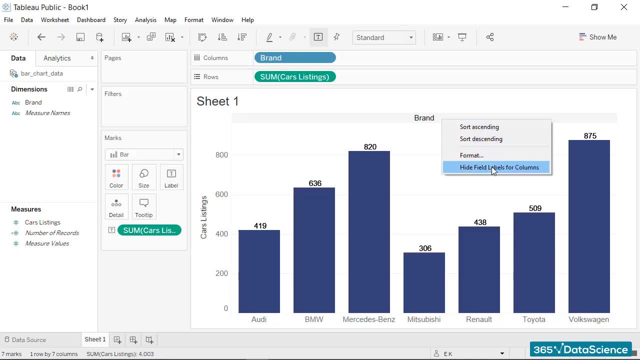 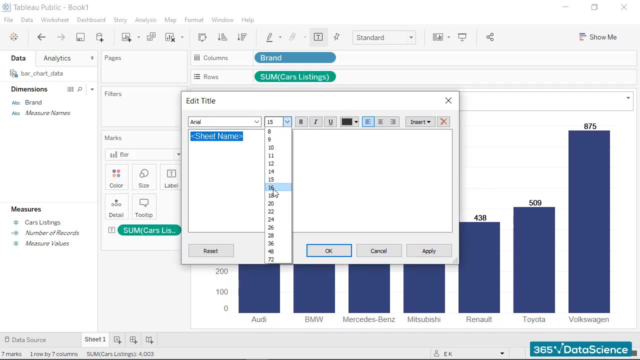 make the visualizations less crowded. we can right-click on it and select Hide Field Labels for Columns. Looks much better. Okay, let's also rename the chart. Then double-click on the field, increase the font size to 16, and bold it for better readability. It's time to type in our new title, which: 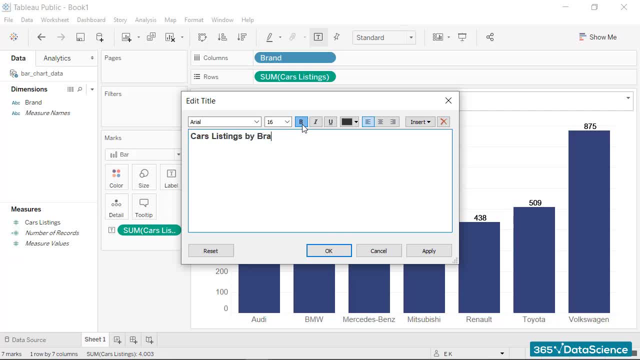 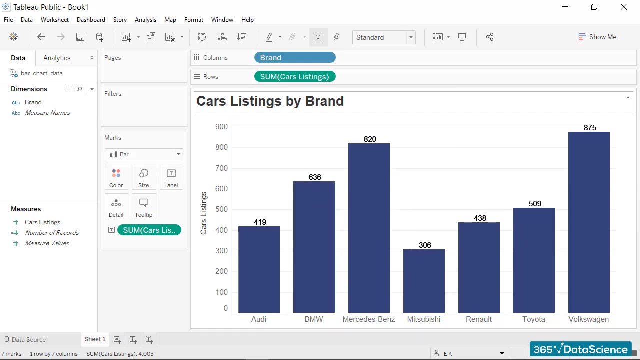 will be Cars Listings by Brand. Remember, having an informative title is an integral part of creating any chart. We'll click Apply and… we have a new title. Excellent, Now, this looks like a presentation-worthy chart. All that's left is to save our work. 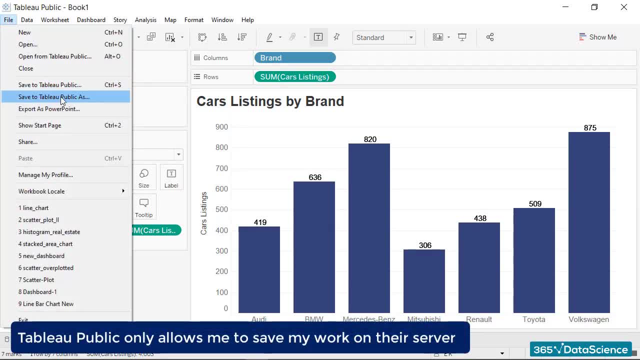 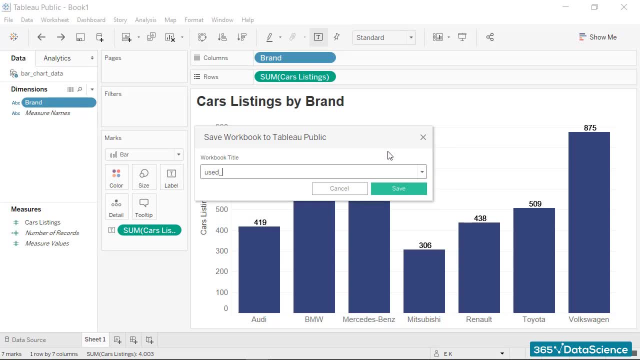 I'm using Tableau Public, which only allows me to save my work on their server. If you already have an account, you can just enter your name and password and save your file on the Tableau server. Alternatively, you will have to complete their registration process. 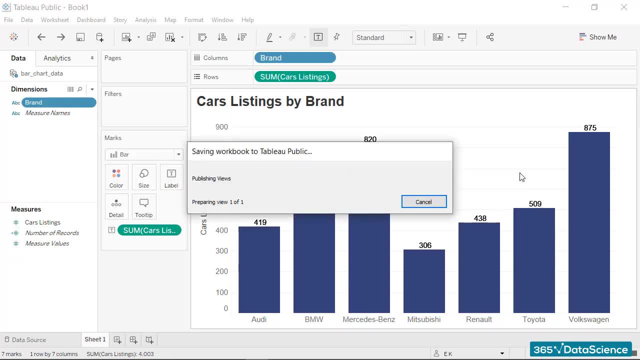 Finally, depending on the size of the file you're uploading, save your file on the Tableau server. Finally, depending on the size of the file you're uploading, save your file on the Tableau server. Finally, depending on the size of the file you're uploading, save your file on the Tableau server. 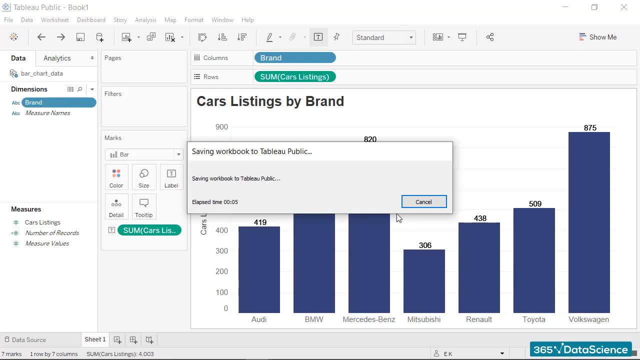 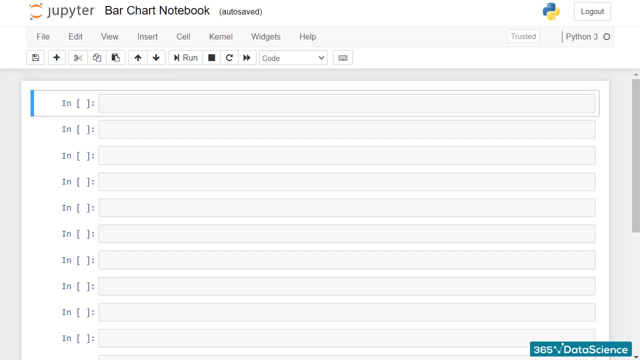 Saving. it might take a little while. Alright, good job everyone. We've successfully created and saved our first bar chart in Tableau: Creating a bar chart with Python. Let's get right to it. The first order of business is to import the libraries we'll need to create our bar chart. 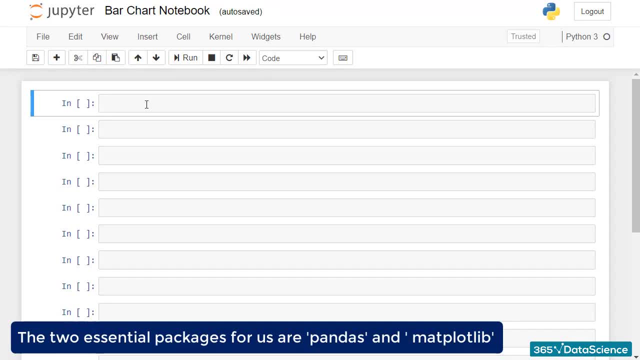 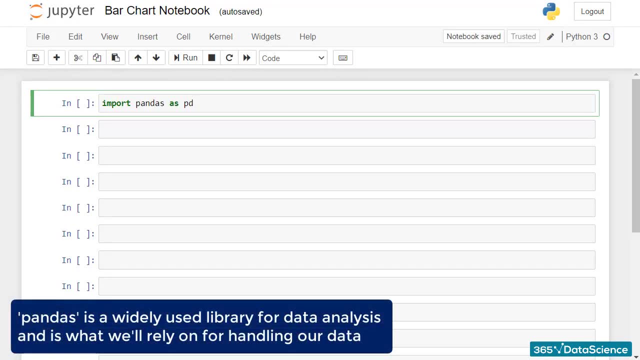 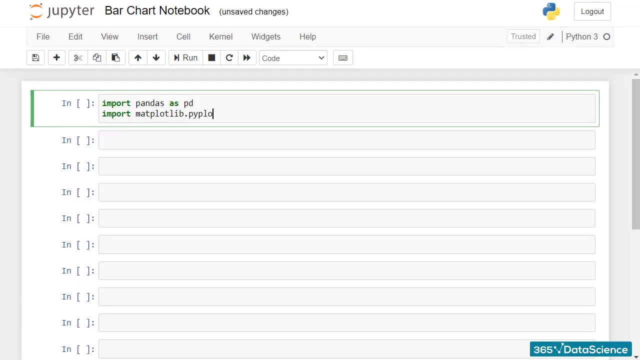 The two essential packages for us are pandas and matplotlib. Let's import pandas as pd. pandas is a widely used library for data analysis and is what we'll rely on for handling our data. Then we will also import matplotlibpyplot as plt. matplotlib is the library we'll be. 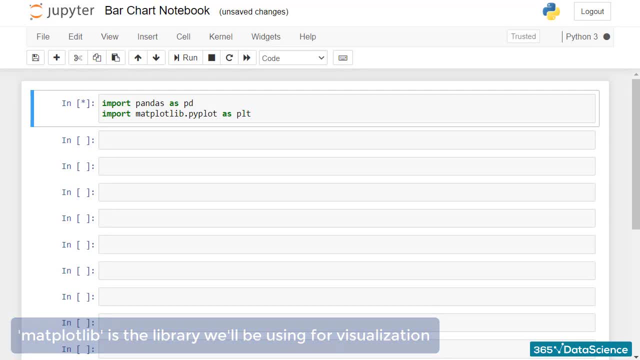 using for visualization. Let's import matplotlibpyplot as plt. matplotlib is the library we'll be using for visualization. Then we will import matplotlibpyplot as plt. matplotlibpyplot is the library we'll be using for visualization. OK, now that we're all set, we can proceed with loading our dataset. 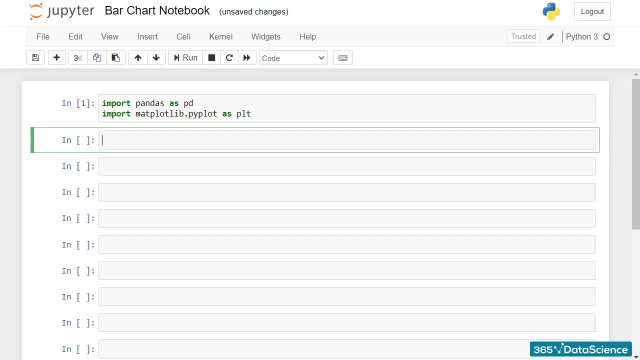 We'll name our first variable df-used-cars and use the pandasreadcsv method to load our CSV file. Our file is called barchartdatacsv. If your dataset isn't in the same directory as your Jupyter Notebook, you'll need to. 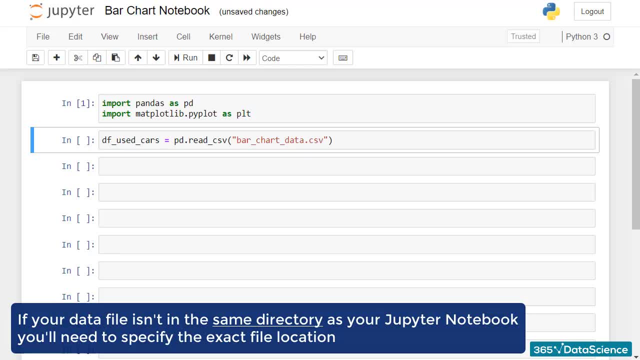 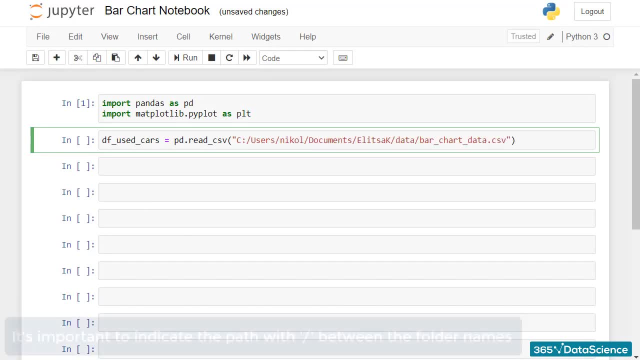 specify the exact file location. For instance, if I were to use the exact path, my code would look like this: Here it is important to indicate the path with forward slashes between the folder names. This is counterintuitive as the path locations in your Windows or Mac. 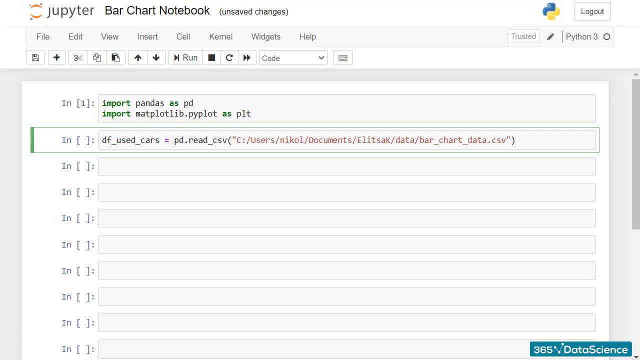 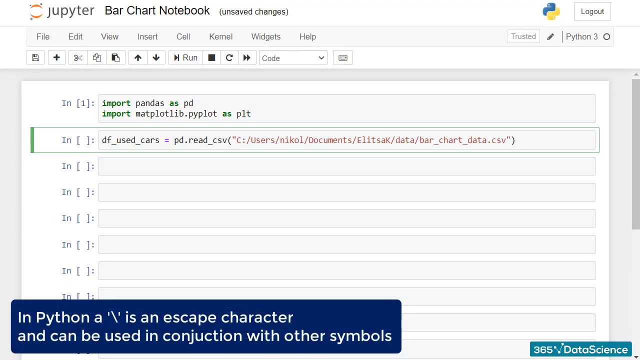 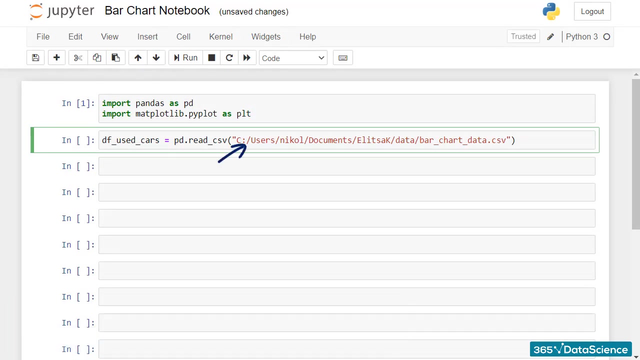 are always specified with backward slashes. However, in Python, a backward slash has a different meaning. It is an escape character and can be used in conjunction with other symbols. Therefore, always remember to use only forward slashes when specifying a path to a file. Good, After we've loaded the CSV file, we can 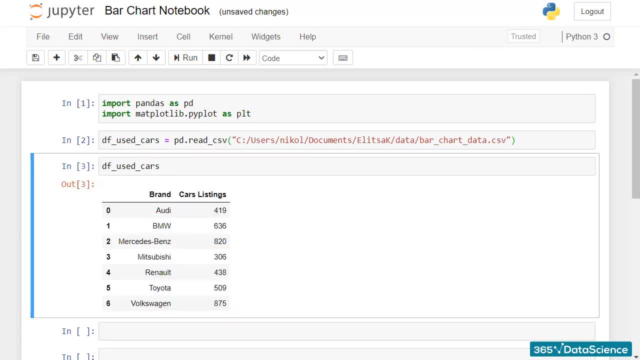 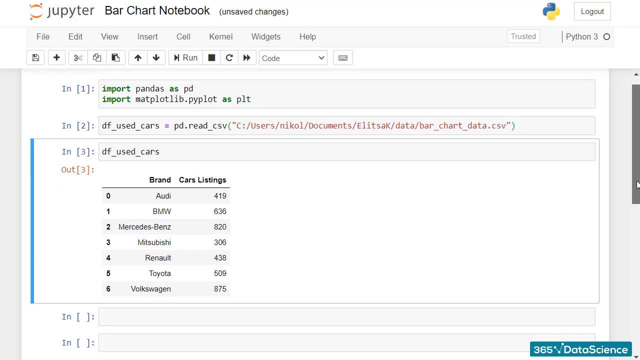 check what the data frame of used cars contains. It looks identical to the dataset we have already examined. Now let's see how we can translate this information into Python. First, we need to create a function in the form of a bar chart- Luckily, the pyplot module. 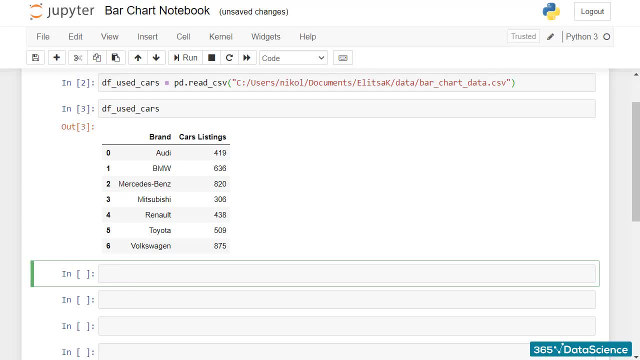 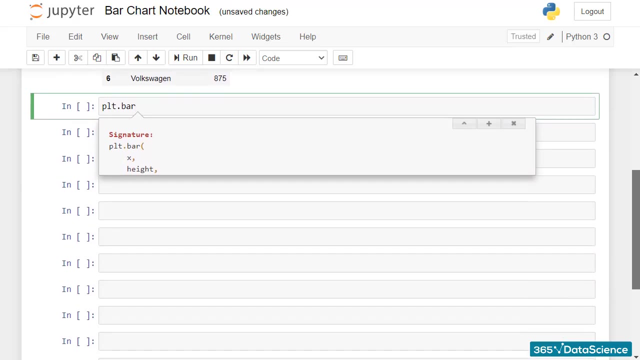 from matplotlib has a readily available barplot function. We'll need to type pltbar Before we go any further. let's hold shift and press the tab button. A window appears allowing us to explore the different parameters of the function. Unsurprisingly, 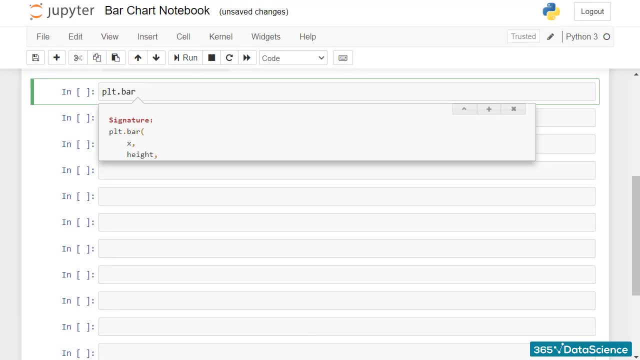 the first parameter is the x-axis, The second called height, The second called height is the y-axis, and so on. We can expand the window with the plus sign and scroll through. Alternatively, we can access a detailed description of functions and parameters through matplotlib's online. 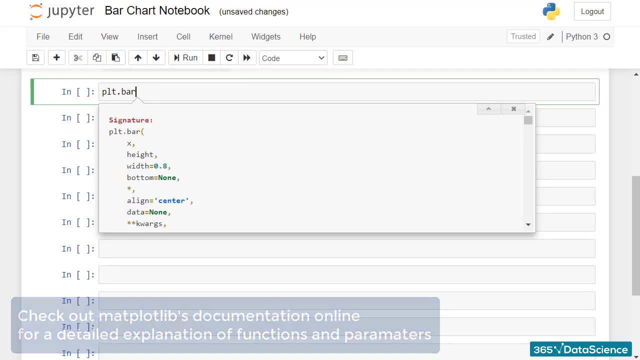 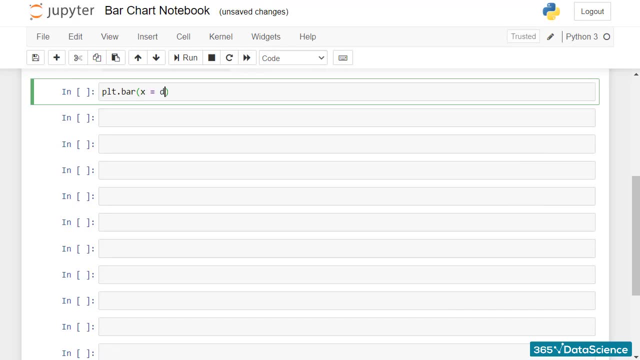 documentation For our bar chart. we'd like to plot the number of car listings by brand. Therefore, for the x-axis, we should select the brand column from the cars listing dialog. We see here we'll have a number of car listings by brand. Therefore, for the x-axis, we should 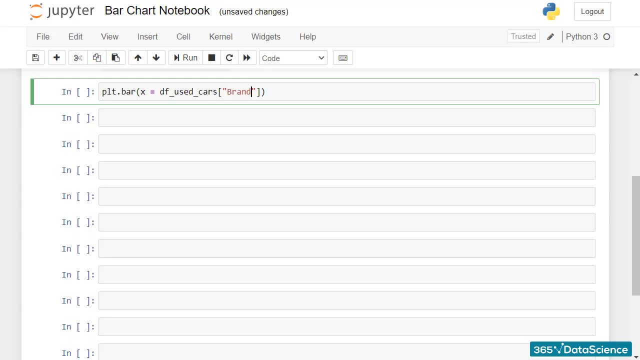 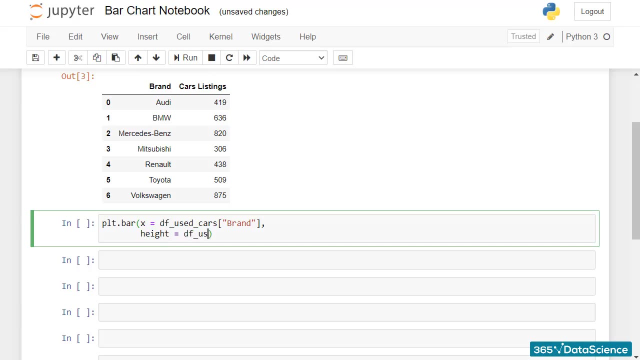 from the cars listing variable On the y-axis, which is the height, we'll need the number of cars sold. Hence from our used cars data frame, we'll take the second column, cars listings, Also as the last line we ought to include. 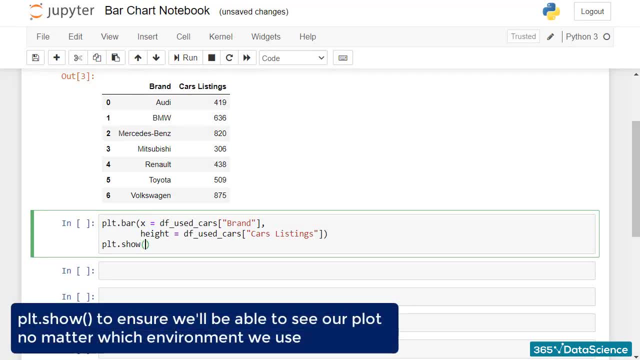 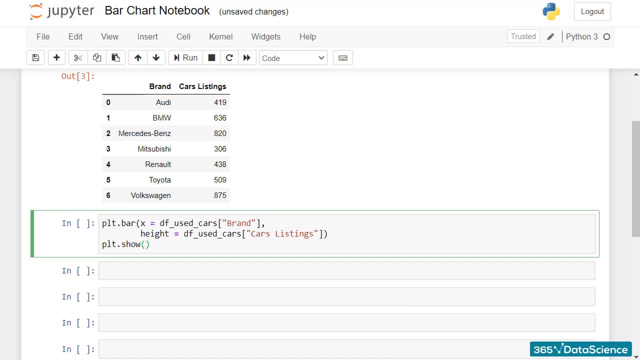 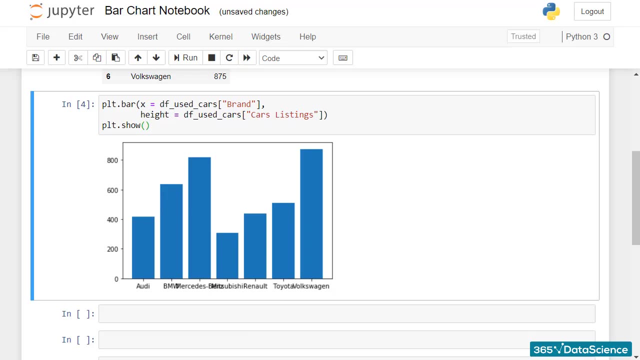 pltshow to ensure we're able to see our plot no matter which environment we use. Alright, let's run the cell and check the result. Look at that. only a line or so of code is all that's required to create a bar chart. Good job. 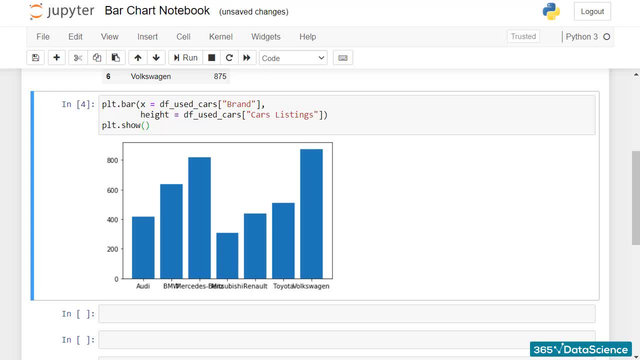 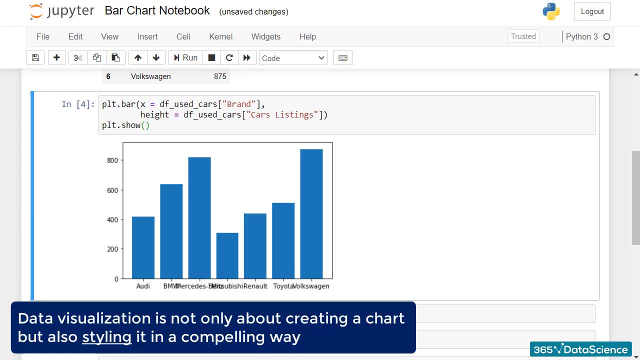 Now, although this chart is displaying the correct information, we can still improve its appearance. Data visualization is not only about creating a chart, but also styling it in a compelling way. Therefore, let's spend some time on that too. With each result, we'll be able to see how many cars we've sold and how many cars we've sold. 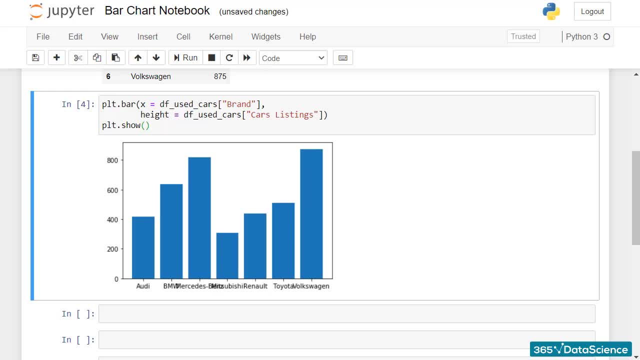 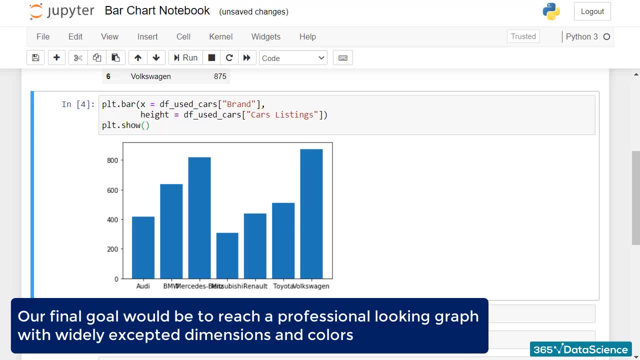 With each result we'll be able to see how many cars we've sold and how many cars we've sold With each visualization we create in this course, our final goal would be to reach a professional graph with some widely accepted dimensions and colors. 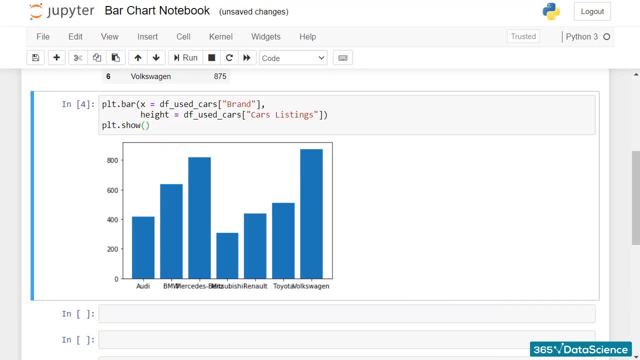 So let's get straight to it. First things first. we want to be able to read all the labels on our x-axis and at the moment they are overlapping. We can resolve the issue by increasing the size of the plot. The default size is 6.4. 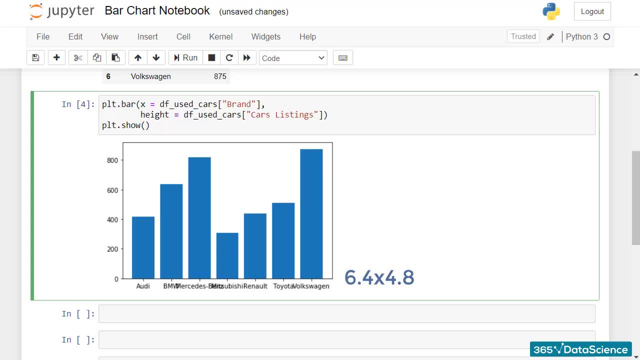 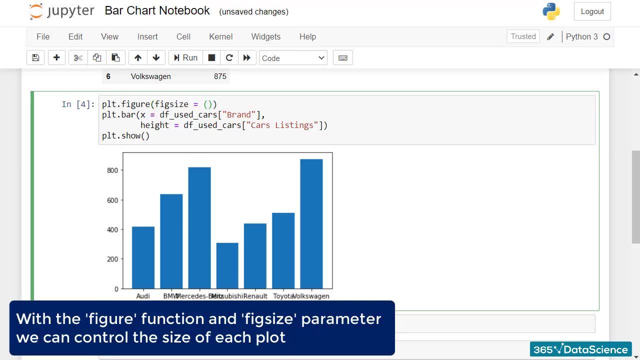 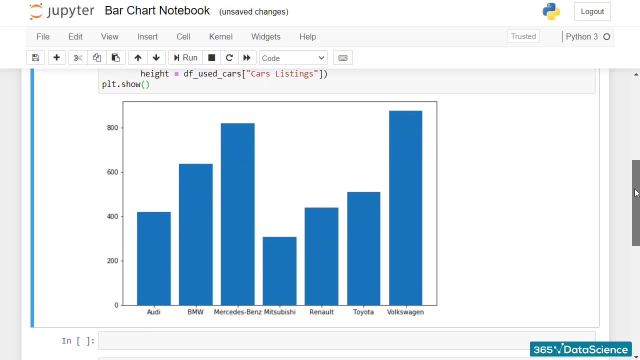 point, 8 inches. We could increase it by specifying the size through the fig size parameter. From my experience, a 9 by 6 figure will be appropriate for most visualizations. Excellent. But there is another way as well. We can avoid overlapping labels by rotating. 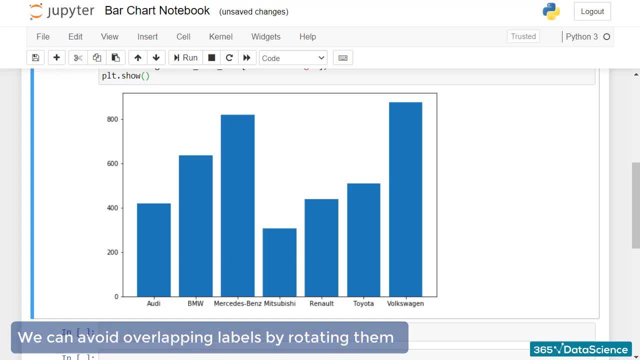 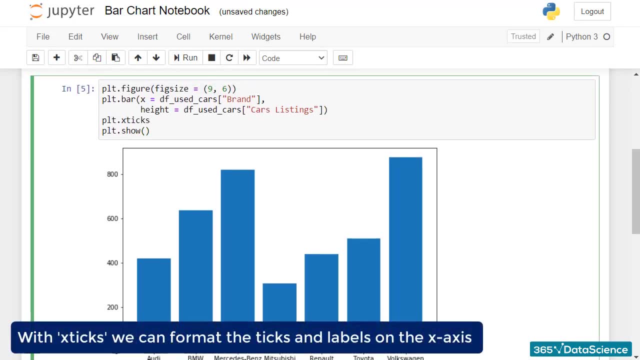 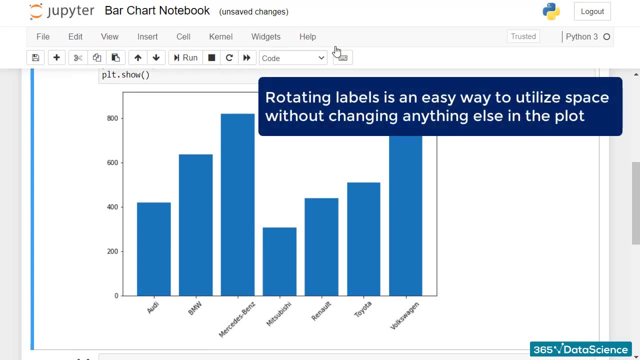 them. Let's try it out, shall we? We'll just introduce an additional line of code, which is a x tix with a rotation angle of 45 degrees, And here's the result. Rotating labels is an easy way to utilize space without changing. 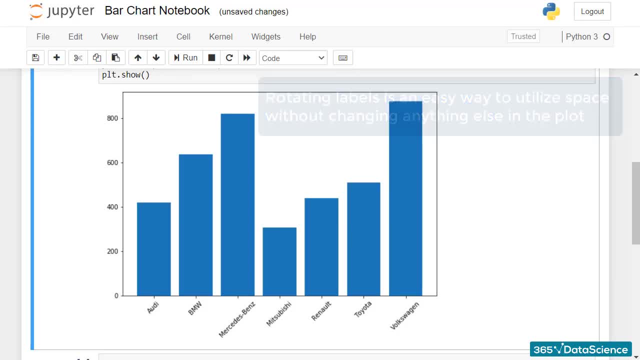 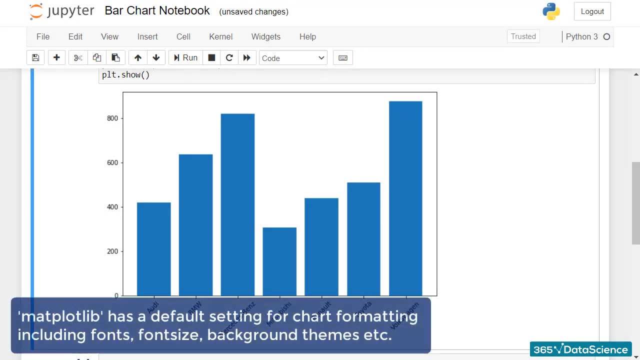 anything else in the plot. Now that that's out of the way, let's enhance our chart a bit more. So far we've been working with matplotlib which, as a visualization library, has a default setting for chart formatting, including font. 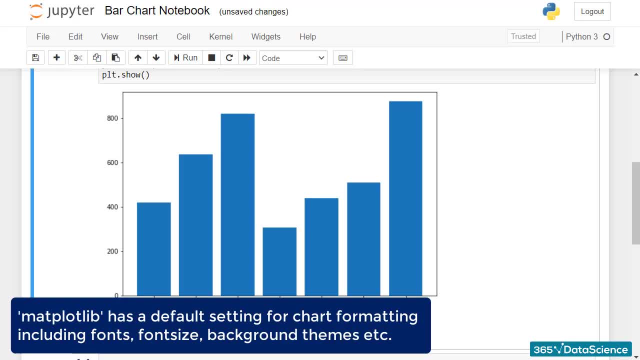 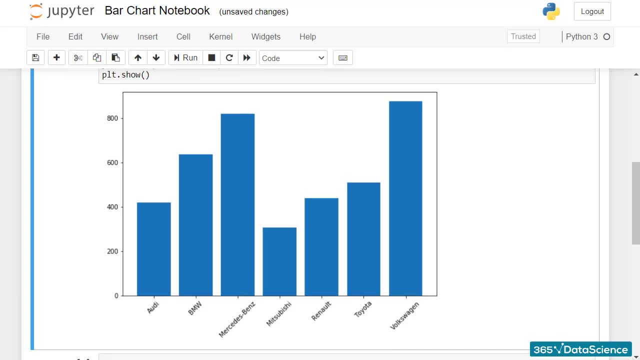 font size, background themes, etc. Sadly, this particular look isn't everyone's cup of tea. Not long ago, a new visualization library called Seaborn has emerged and has become the preferred choice for many programmers, especially in the field of data science. Seaborn- 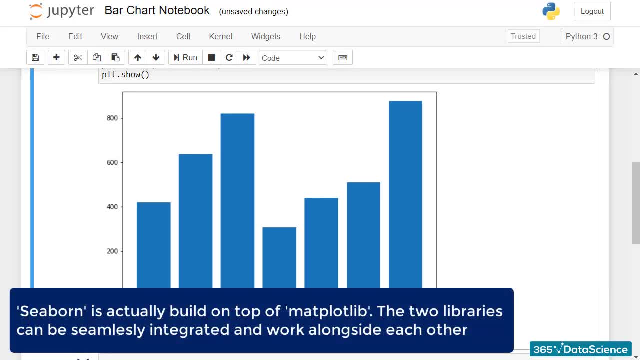 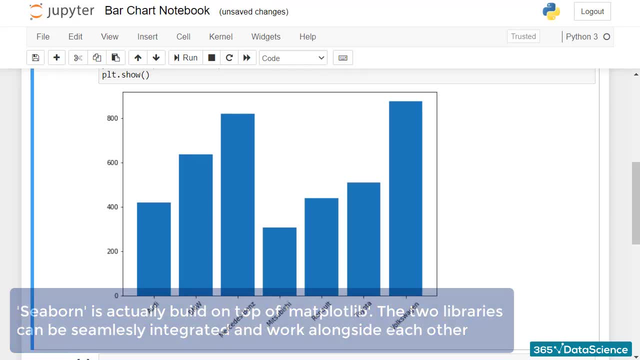 is actually built on top of matplotlib. As such, the two libraries can be seamlessly integrated and work alongside each other, which is great news for us. To be more precise, we can import Seaborn and set its look to overwrite the default one in matplotlib. Let's scroll back to the top of our code. 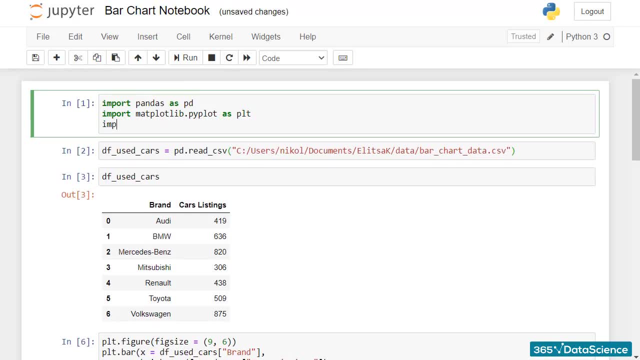 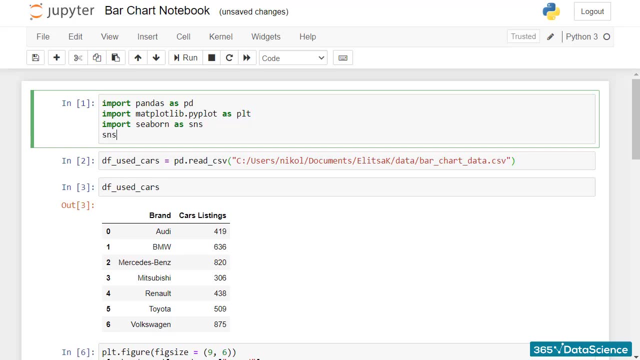 and try it out. First, we'll import Seaborn as sns and secondly, we'll overwrite the matplotlib look with snsset to take advantage of the Seaborn styling. In essence, this will allow us to code the graphs in matplotlib, but they will be displayed. 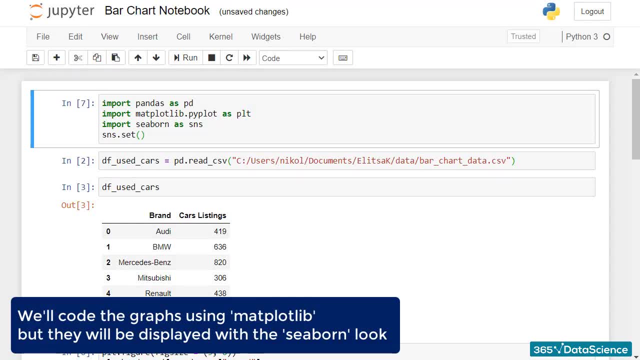 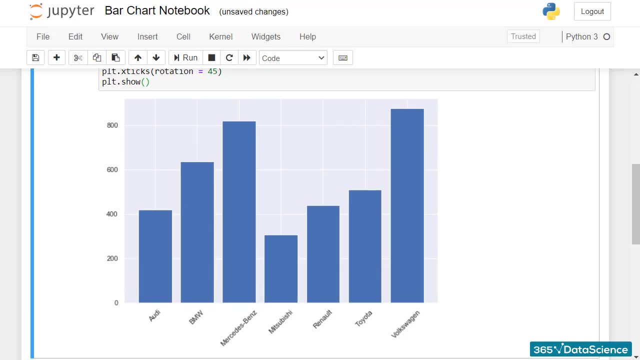 with what some call the much superior Seaborn look. Alright, it's time to put it to test by re-running the last cell of code. Tremendous, Moving forward. we'll be sticking with the Seaborn visuals in the majority of cases. 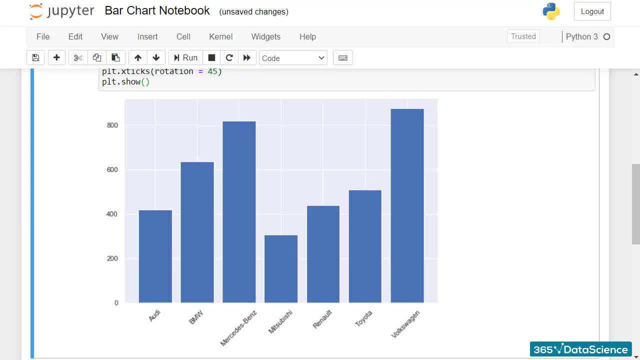 What's next on the agenda? Generally, data visualizations convey insights through shape and color, While the shape is somewhat restricted by the nature of the data. the color is up to us. Let's take a look at the data visualizations. Generally, data visualizations convey insights through shape and color, While the shape is somewhat restricted by the nature of the data. the color is up to us. 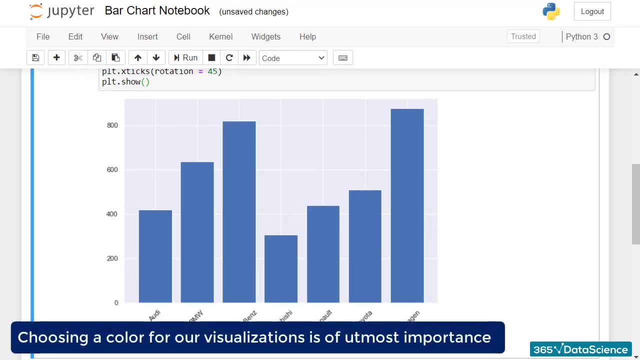 Let's take a look at the data visualizations. Generally, data visualizations convey insights through shape and color. While the shape is somewhat restricted by the nature of the data, the color is up to us. Nonetheless, choosing a color for our visualizations is of utmost importance and should be thought. 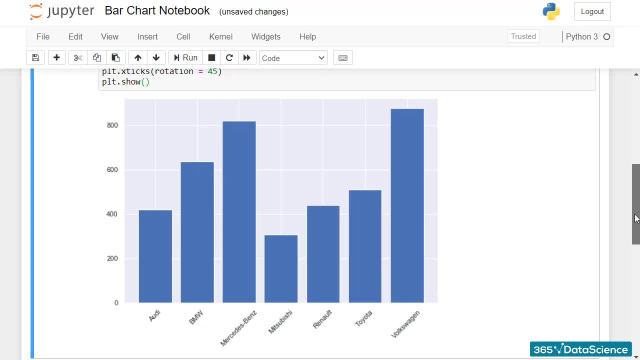 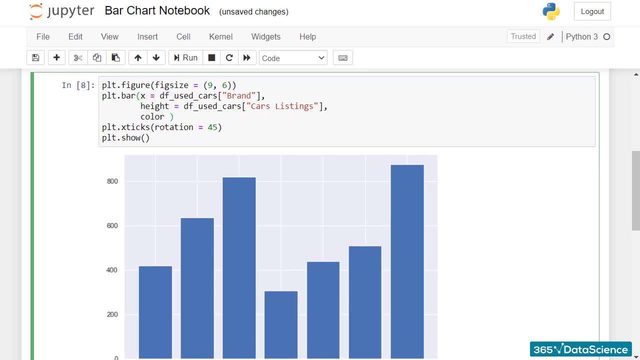 through carefully. In matplotlib, we can change the colors of our plot by adding a color argument. Furthermore, we can choose a color name from a predefined color list available in the Seaborn library. Seaborn recognizes over a hundred color names, starting from the basic ones. 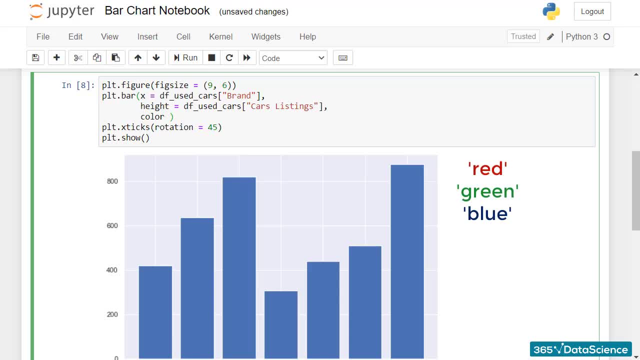 such as red, blue and blue. Seaborn is also named after the colors Oldweb, Clued, Green or Blue, which we can refer to by their initials, RGB respectively. If you're feeling more adventurous, you can. 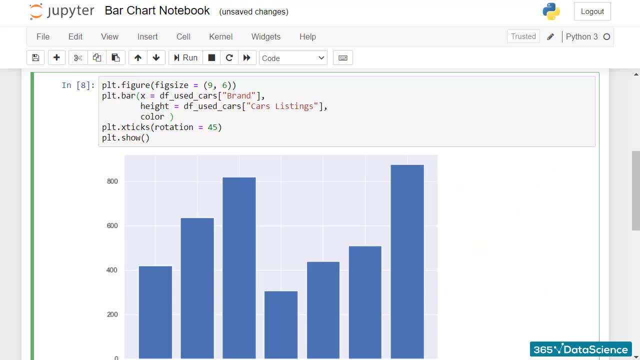 also choose colors such as Linen Honeydew or Dark Orchid. In fact, you can assign an individual color for each of the bars. Let's see how. We have seven columns and will assign each their own color. We can type in a string with the following seven letters: 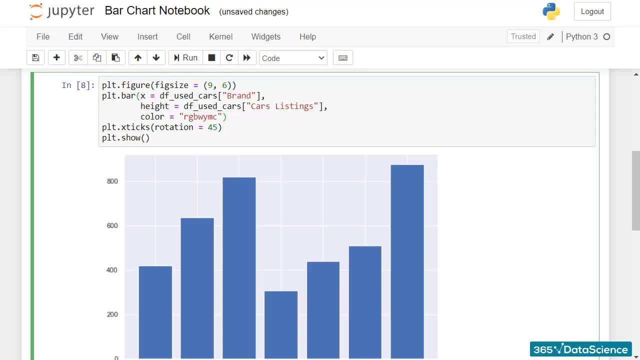 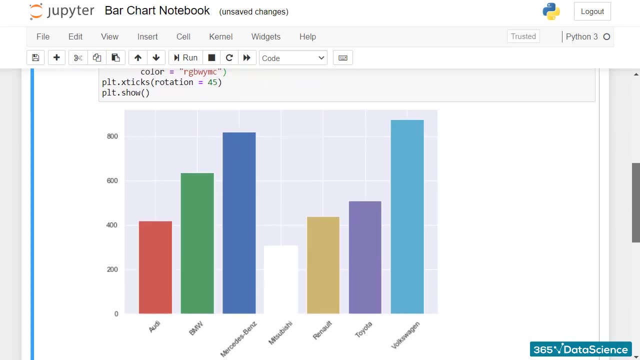 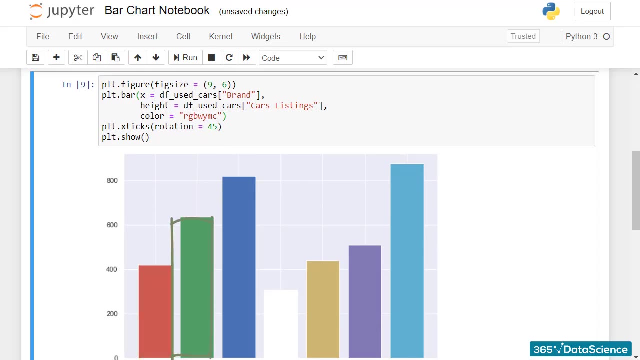 RGBWYMC. You can type in anything along those lines. Each of these letters is an abbreviation for a frequently used color. Here's what we get Cool. Each column has been assigned an individual color. We have… R for red, G for green. 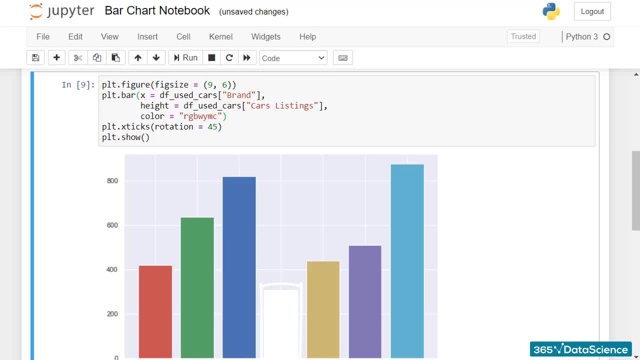 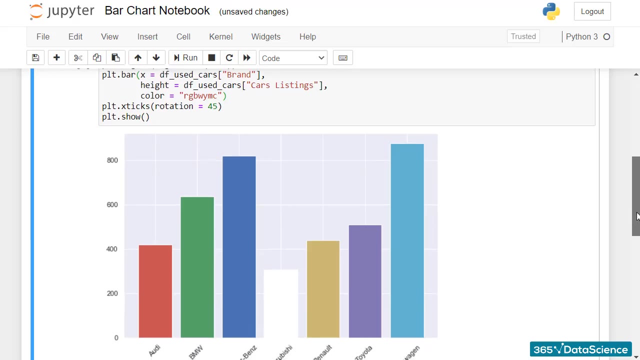 B for blue, W for white, Y for yellow, M for magenta And lastly, C is for cyan. This shows how versatile plotting in Python is. We can specify a color for as many bars as we have in this manner. 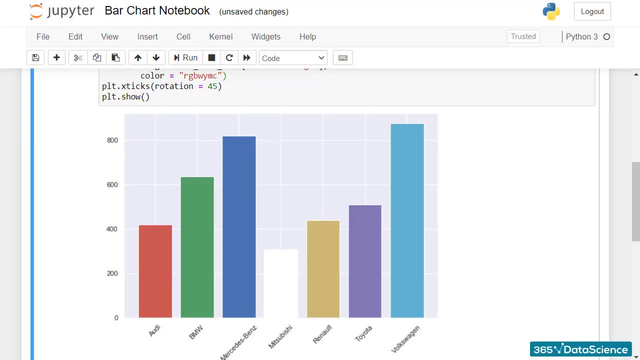 Just bear in mind: the color abbreviations aren't limitless. Therefore, at some point you might have repeats. However, in a professional presentation, we want our color to be uniform across the whole worksheet. Therefore, let's choose dark blue or midnight blue. 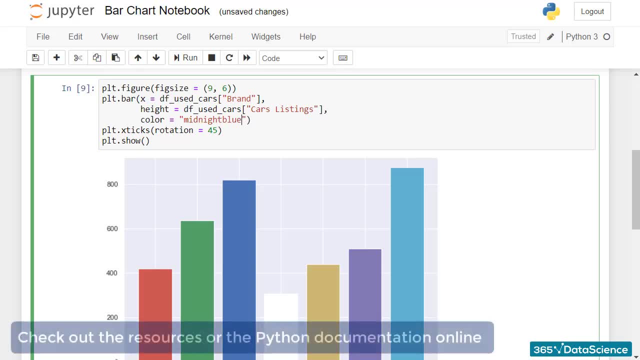 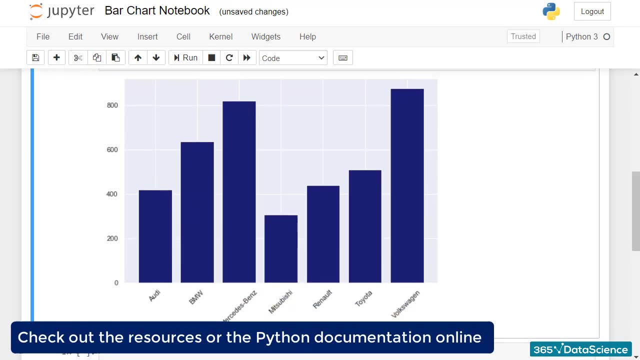 as the color we want. This is the only color of our bar chart. You can find the full list of colors in this lecture's resources or check the Python documentation online. Okay, What's left? Well, every plot needs a title. To integrate a title, we type plttitle. 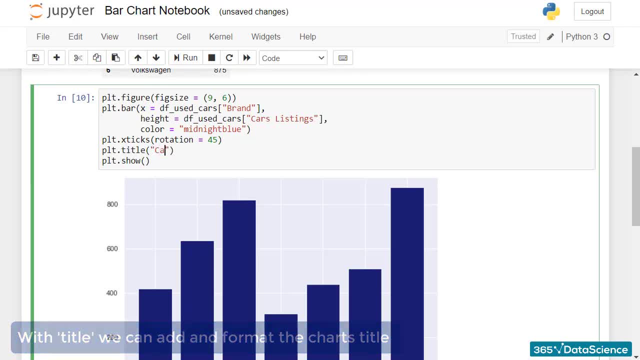 and in brackets, specify the desired title. Cars listings by brand has a nice ring to it. Note that you need to put that in quotation marks So that Python knows that it is a string. Let's examine the result While we've successfully placed a title on top. 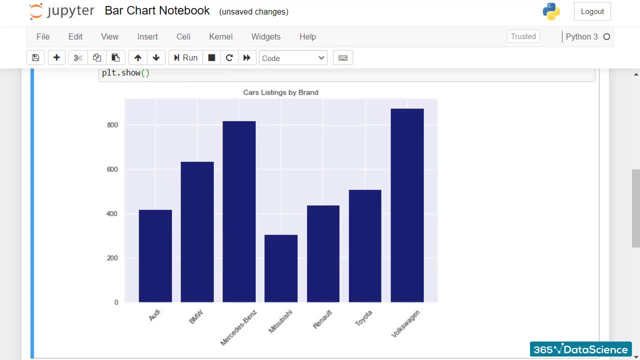 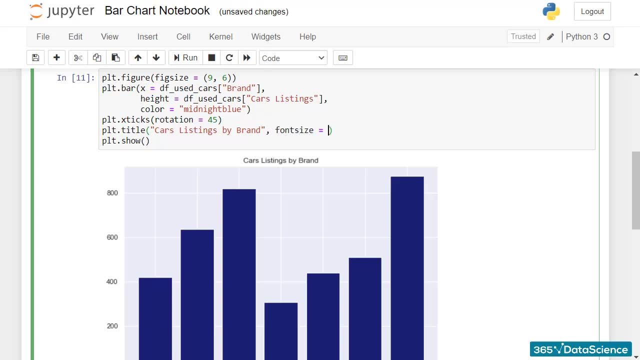 it is a bit small compared to the rest of the graph, But no worries, Everything in Python is customizable. We can increase the font size by adding an extra argument and then specify a font size of 16.. We could also add a font weight argument and set it to bold. 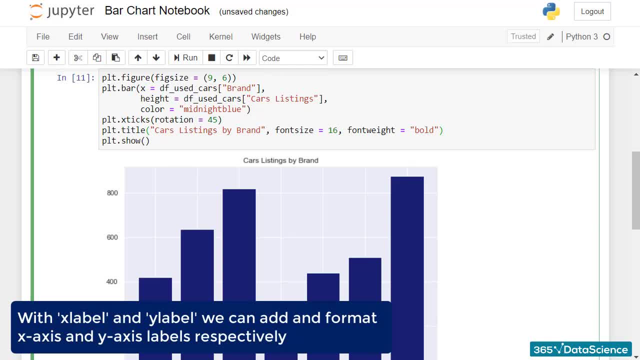 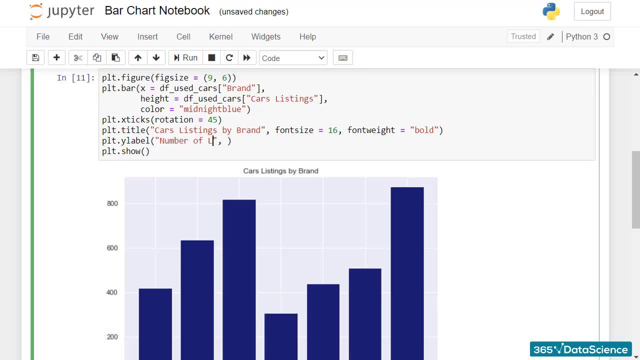 Here we could also do weight. We could also do with a y-axis label. To add one, we just write pltylabel and in the brackets specify the name as a string. I know for a fact the axis label appear a bit smaller. 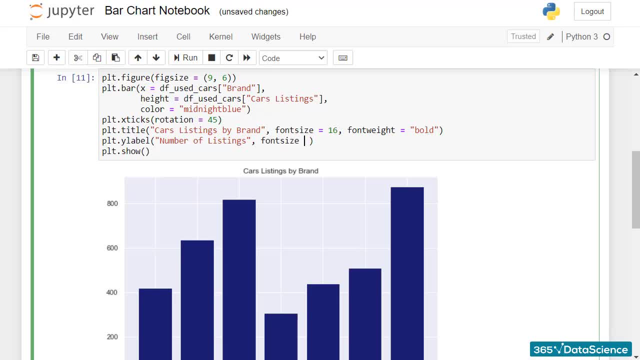 So let's increase their size to a 13 with the font size parameter. In fact, let's also format the other text elements a little bit so they look more pronounced. Increase the font size to 13 for the x and y-axis labels. 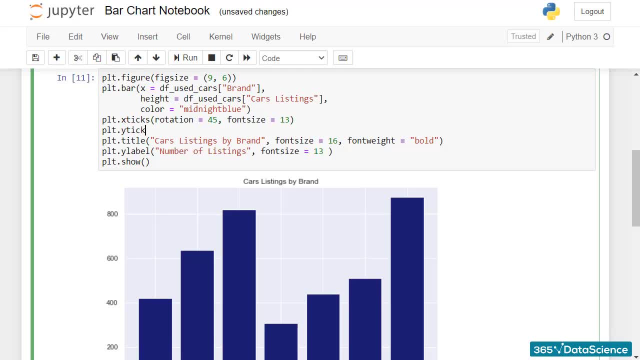 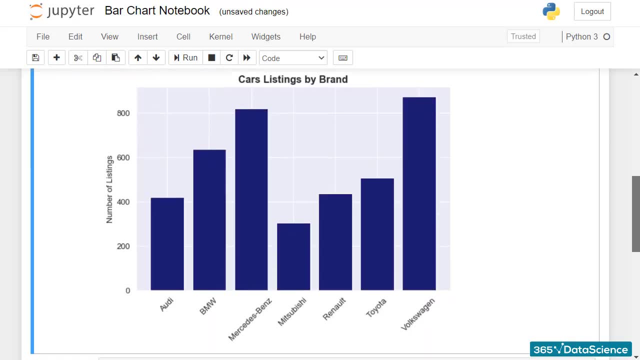 and then set the y-ticks font size to be equal to 13 as well. Marvelous, Our bar chart looks presentation ready. A quick side note: Not all people are comfortable with coding in Python. In fact, you may often need to use your plot outside a Jupyter notebook. 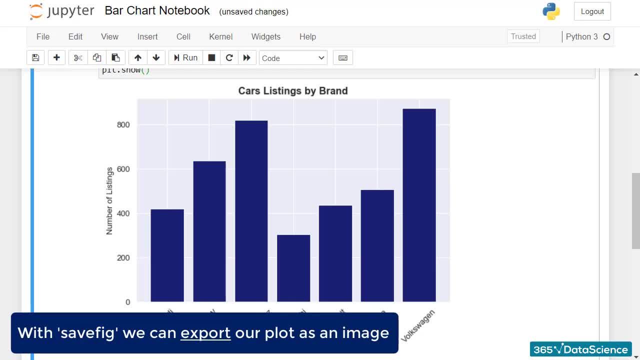 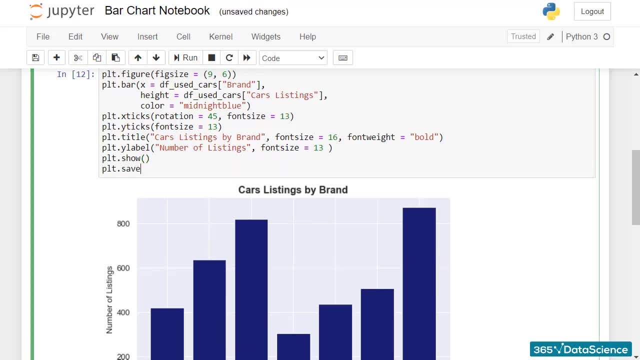 To achieve that, you can export your plot as an image. This is achieved with the saveFig method. In the brackets we need to specify the name and file format. In our case it will be a PNG, So we'll have usedCarsBarpng. 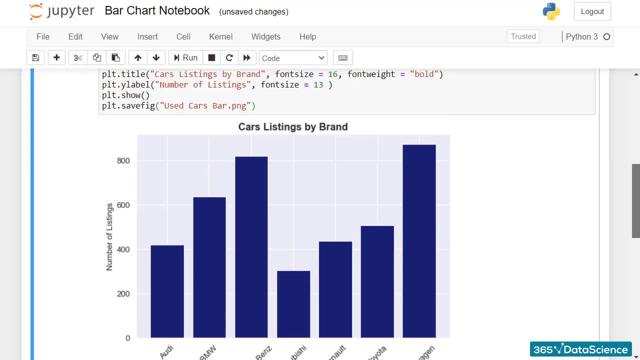 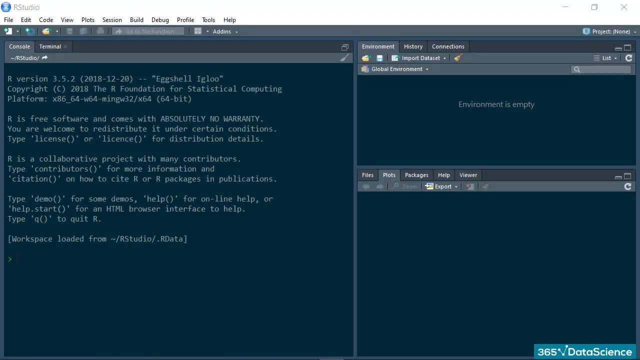 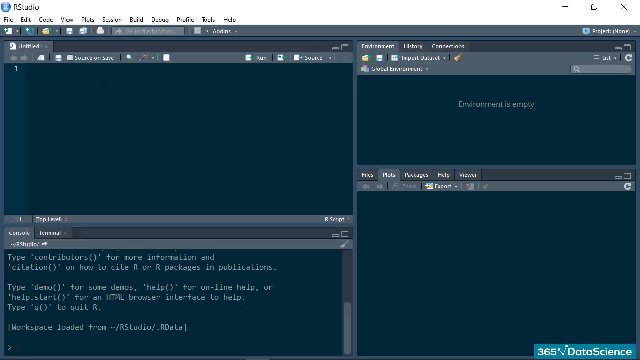 And that's it. Great job everyone. Creating a bar chart with R. So let's jump straight into RStudio and start writing some quality code. The first thing we need to do is open up a new script. It is a good idea to begin by saving it under an indicative name. 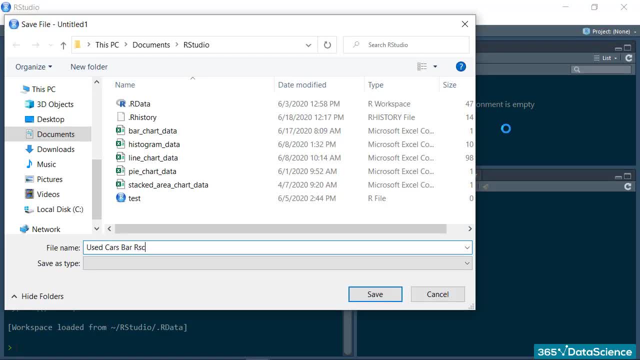 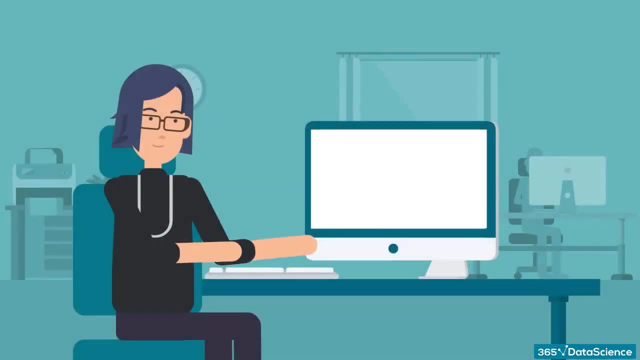 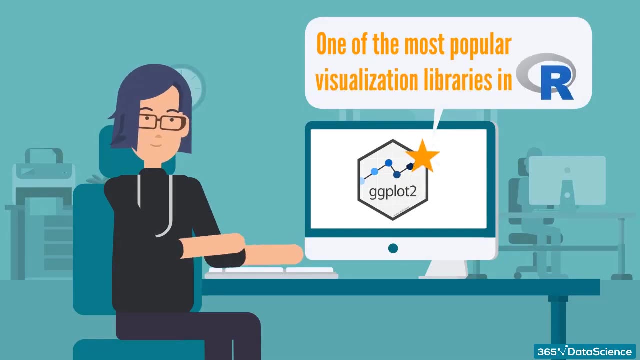 such as usedCarsBarRscript. So far, so good. We'll be using ggplot2.. It's one of the most popular visualization libraries in R and a favorite among the community. This is the library we'll be using for the majority of our visuals. 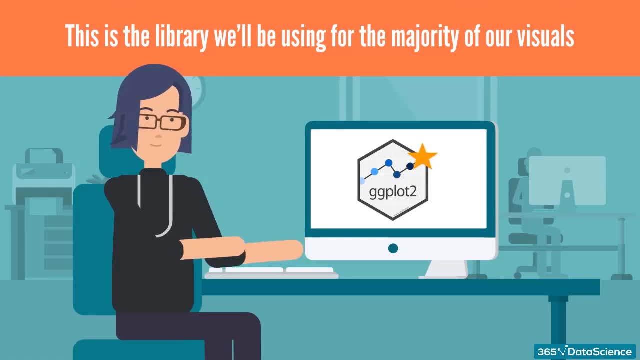 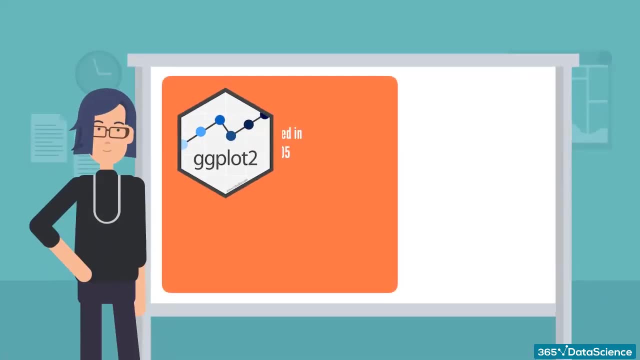 so it's worthwhile to take a second and see what ggplot is all about. We're ready to start talking about ggplot2.. ggplot2 was developed in 2005 by Hadley Wickham. It relies on a concept known as the grammar of graphics. 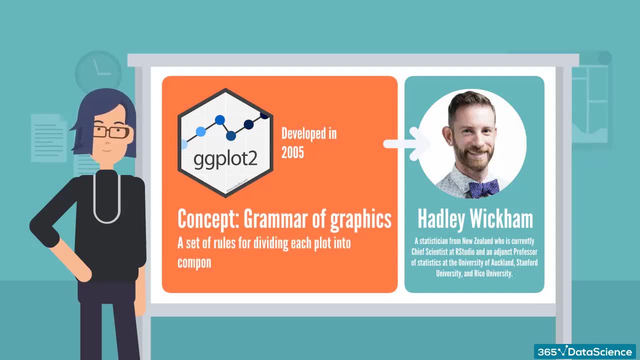 which is a set of rules for dividing each plot into components or layers. It is also the basis of how each ggplot is created, which is why it pays off to explore the grammar of graphics in more detail Without further ado…. Introducing the grammar of graphics. 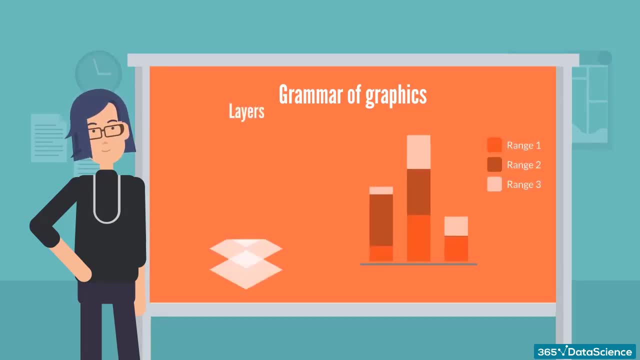 You can think of it as a way of dividing each plot into layers, where each layer is responsible for a specific element of the chart. There are seven layers we can use when creating a ggplot, and, as we delve into different visualization topics, we'll talk about them in a bit. So let's get started. 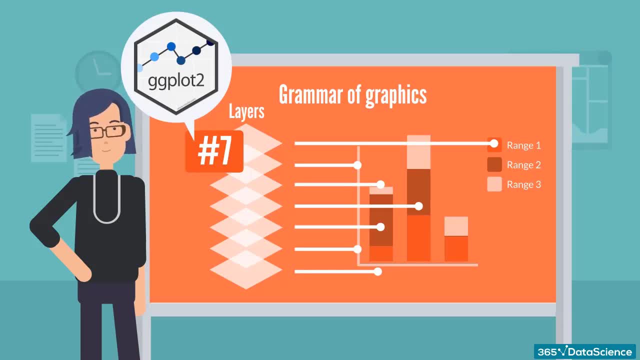 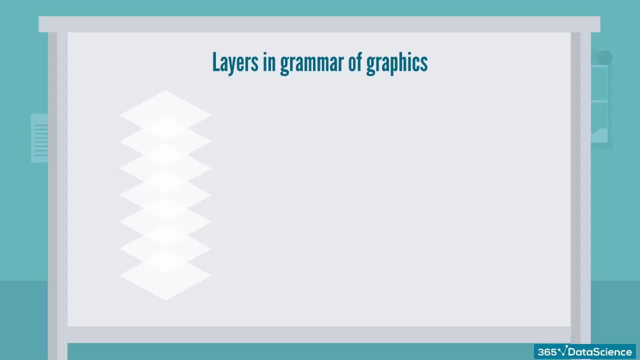 We'll get a chance to explore each in detail. For now, let me give you a quick overview of each of these seven layers, which constitute the grammar of graphics. The first three layers are mandatory, while the remaining four are optional. Let's start with the first layer, also known as the data layer. 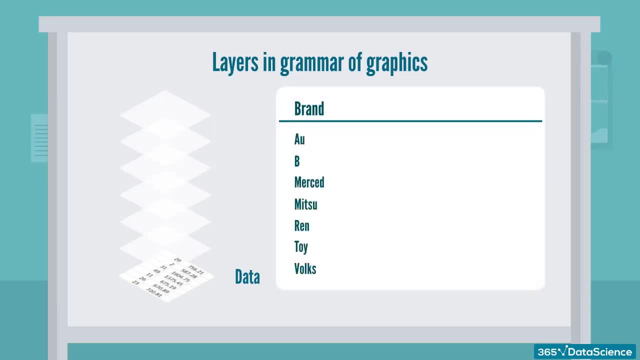 Creating a chart naturally means we require some data, otherwise our chart would be empty. Therefore, it is only logical to use the data layer. It is only logical that this is the first and most important layer. Alright, What else? We must also decide how the data will be visually organized onto different axes. 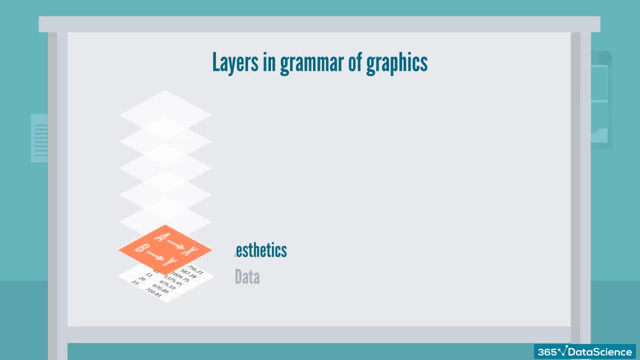 This is where the second layer comes in. It is called the aesthetics layer. Here we specify the mapping to the X and Y axes. Good, The last required layer is the geometry layer. Through geometry, we specify what shape our data will take. In other words, will the points take the form of bars, circles, dots, etc. 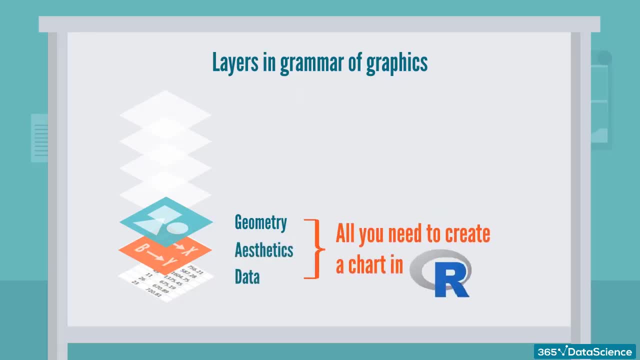 These three layers alone are all it takes to create a chart in R. The remaining four layers are optional. However, since we want to be proficient at visualizing data in R, we'll master them too. An important distinction between the mandatory and optional layers concerns 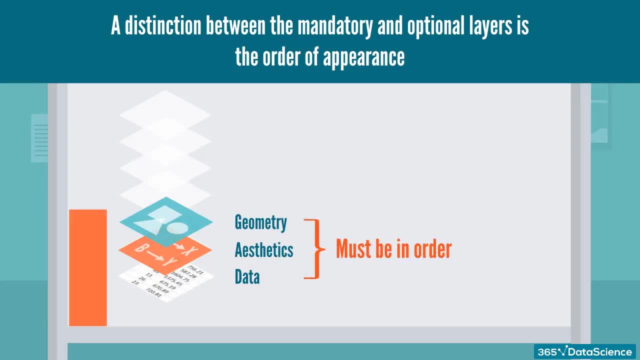 the order in which they appear. For the first three layers, we must start with data, continue with aesthetics and, as a third step, determine the geometries. The remaining four layers don't need to appear in strict order. In fact, we don't have to include any of them in our plot. hence the optional part. 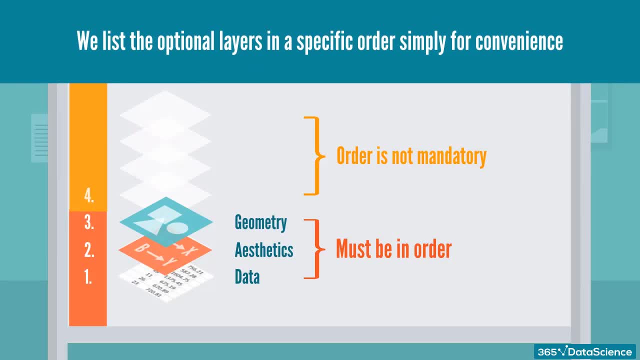 In this lecture, we list the optional layers in a specific order simply for convenience, but it is not necessarily the order in which they should appear in a GG plot. With that in mind, let's continue with the fourth layer, the facets layer. 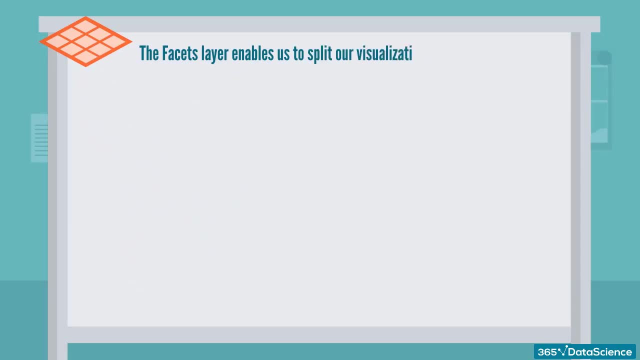 The facets layer enables us to split our visualization into subplots according to a categorical variable or variables. Subsequently, each subplot corresponds to a subset of categories of the variables. For instance, say, we have an engine type variable in our data containing diesel, petrol and electric engine cars. Using the facets layer, 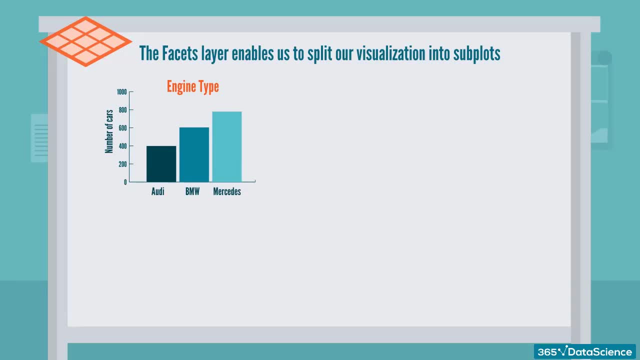 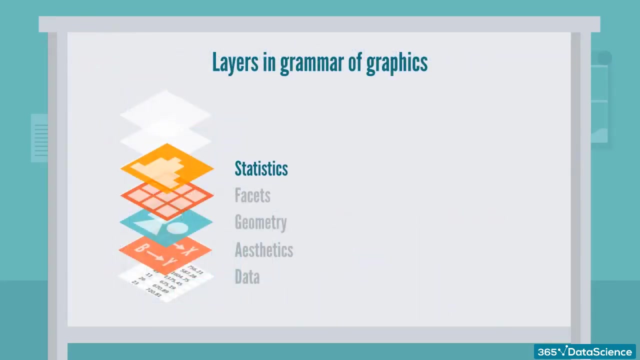 would allow us to divide our dataset into three plots, each containing one of the three categories: Diesel, petrol and electric cars. So far, so good. Moving on to the fifth layer, which is statistics, This layer represents the statistical transformations we might perform on our data. It can be used for various purposes. 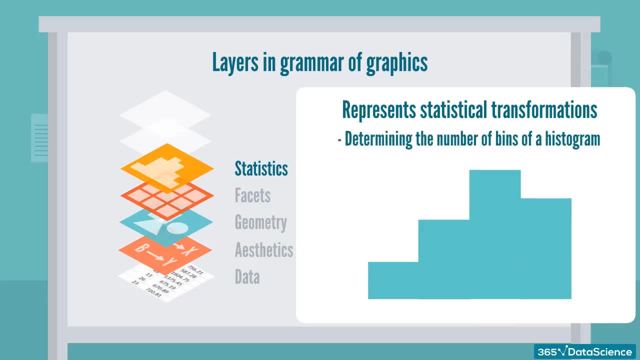 such as determining the number of bins when plotting a histogram or smoothing lines when drawing a regression line Cool. The sixth layer is the cohort. This layer is the coordinates layer. The coordinates layer, as the name suggests, is connected to the coordinates or boundaries of our graphs. This layer can be used to zoom in. 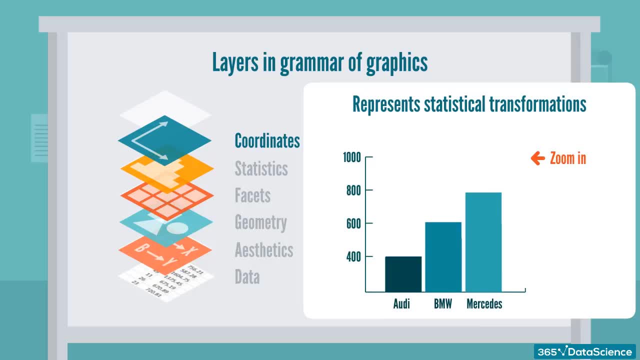 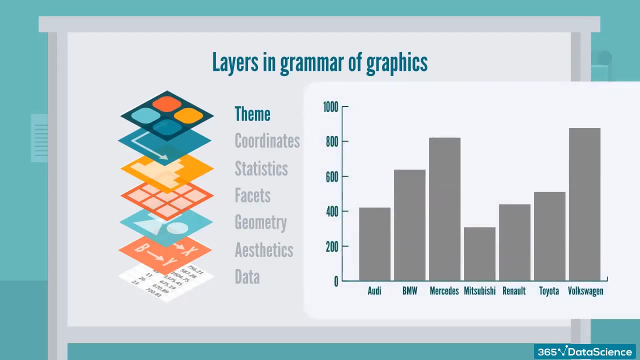 or out of a plot. Apart from this, it could be used to perform transformations on the coordinate system, For instance switch to polar coordinates. Finally, we arrive at the seventh layer: themes. The themes layer has a sole purpose: to polish the appearance of our plot. 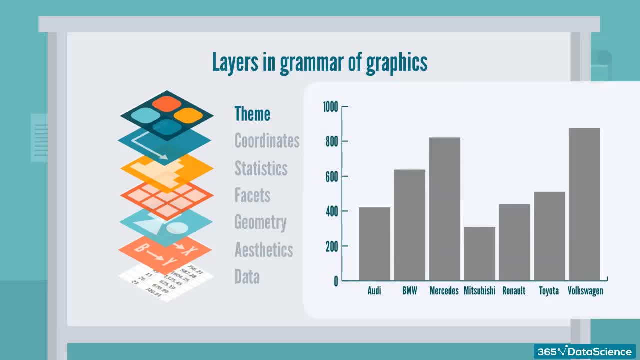 This is the place that controls the overall style of our graph. For instance, we can choose from darker or lighter themes. Not only that: with the aid of the themes layer, we can use predefined templates or recreate the visuals and style of well-known publications such as the BBC. 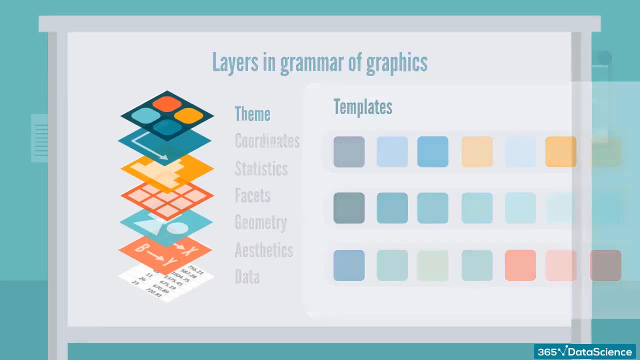 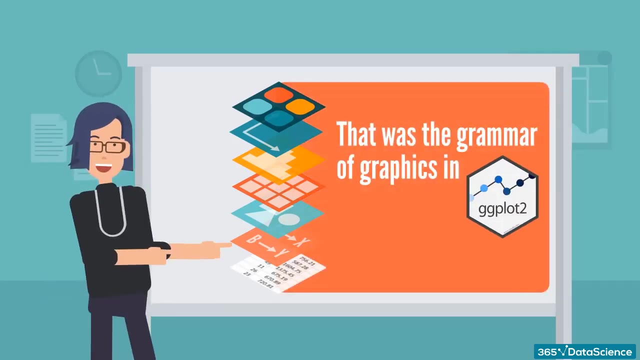 or The Economist, among others. All right, Phew. This is what the grammar of graphics in ggplot2 is all about. You can revisit this lecture if you ever need a refresher, or check out the course notes, Or you can just learn by doing Speaking. 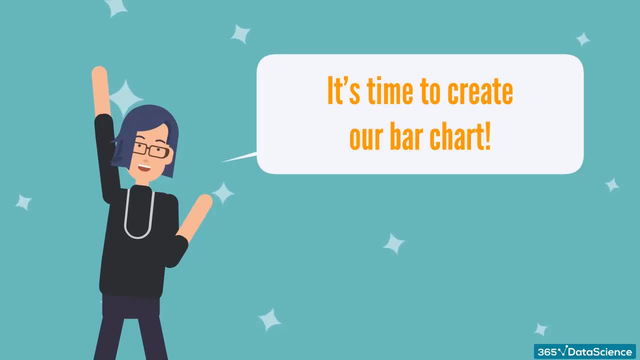 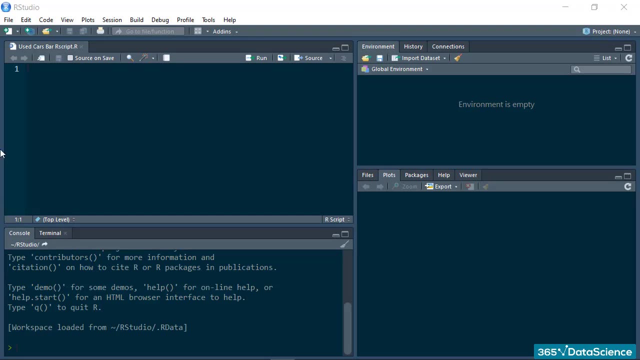 of which it's time to create our bar chart. The first step towards a successful visualization is obtaining the necessary data. Therefore, let's load our data file in a new variable called usedCars and apply the readCSV function As an argument. we need to pass the file to be read. 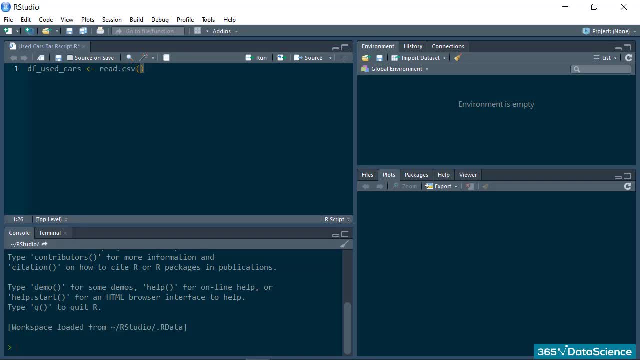 Let's enter our var file in this order. Our file is called barChartDatacsv. If your file isn't in the default r files library, you need to specify the path or directories leading to it. This is counterintuitive, as the path locations in your windows or mac. 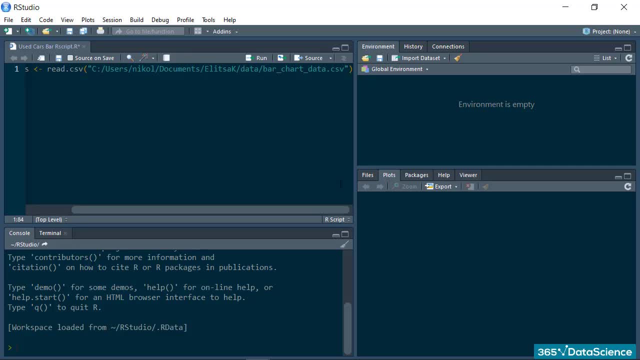 are always specified with backward slashes. However, in R, a backward slash has a different meaning. It has a different meaning when you specify a password slash in your database. It is an escape character and can be used in conjunction with other symbols. Therefore, always remember. 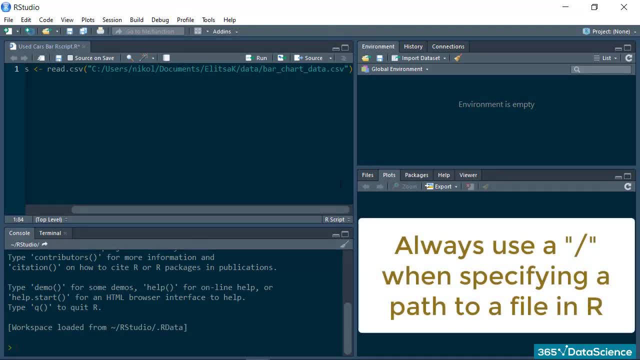 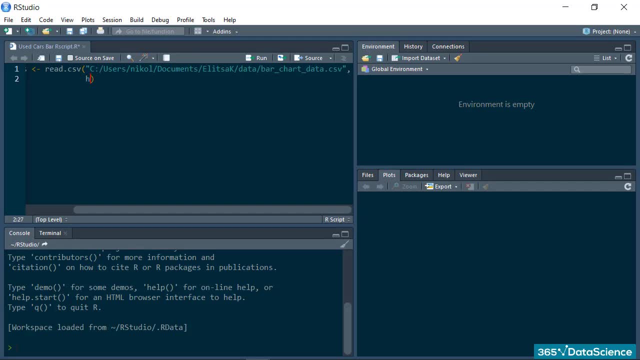 to use only forward slashes when specifying a path to a file. Okay, We specify the header as true, which means that the first row of our data will be used as columns' names. Lastly, we'll indicate that the separator is a comma. 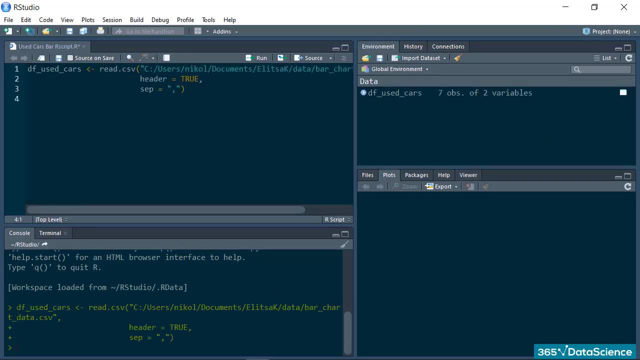 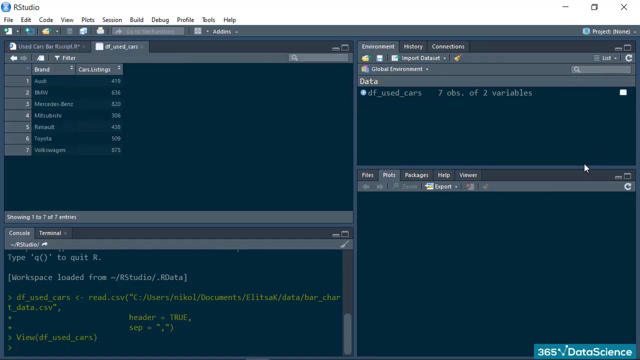 After running the cell, the new variable appears in the top right of window. RStudio. Next to it is a summary indicating used cars- contains two variables with seven observations. Not only that, if we click on used cars, we'll be privy to the entire data set. A great feature. 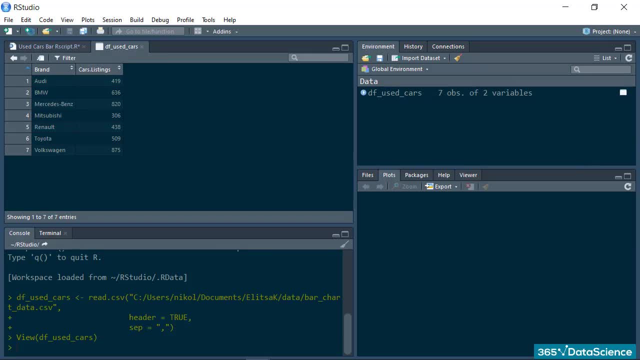 of RStudio, granting us easy access to each variable we create. And now on to creating our first chart. We'll begin by creating our first chart. We'll be relying on the ggplot2 library, which means we ought to include the library. 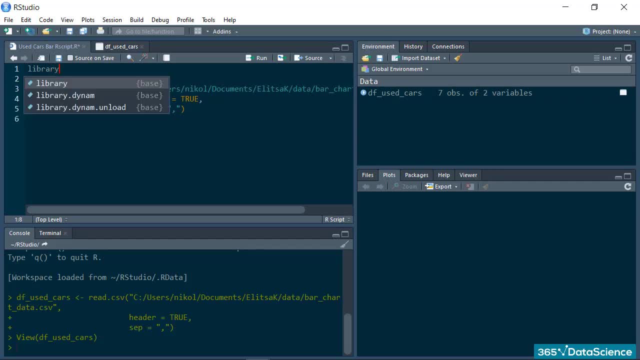 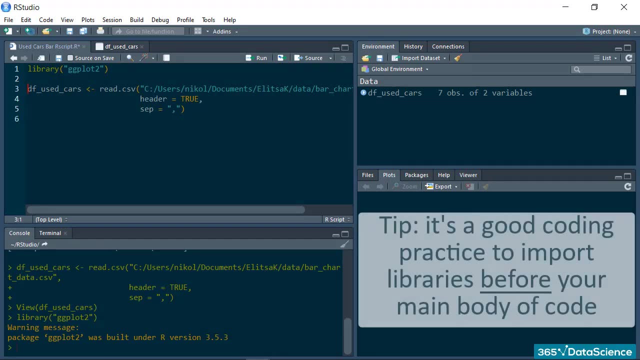 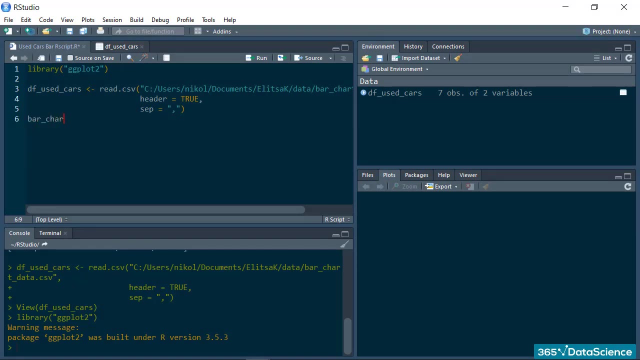 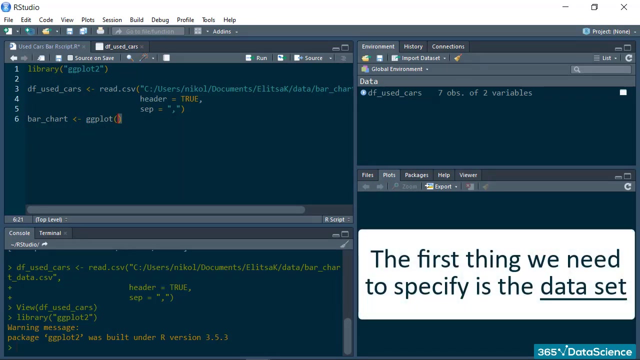 in our script. We achieve it by writing library, When in the round brackets include the name of library, in our case, ggplot2.. Great, Now let's create a new variable which will be a ggplot object. Now, as discussed, according to the ggplot philosophy, the first thing we'll need to specify is: 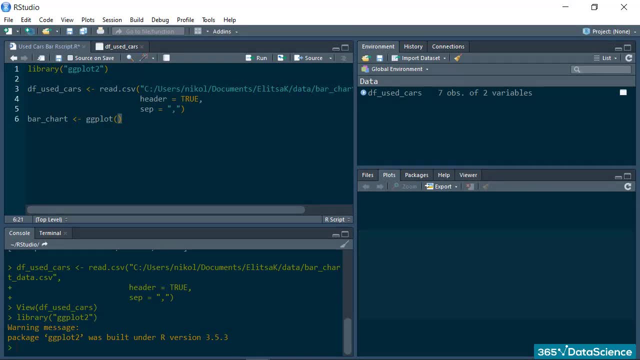 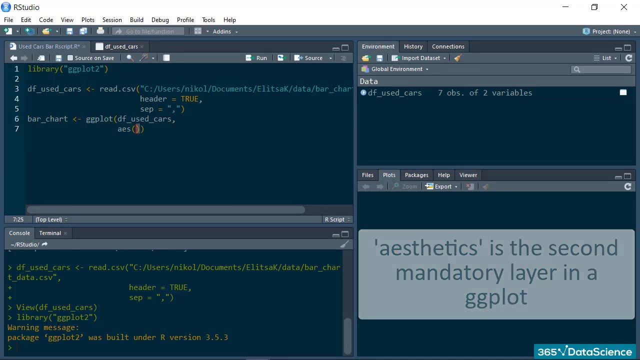 the data set. We'll be plotting our automobile data. hence the first parameter to include is the used cars data frame. Good, The next step is to specify the aesthetics, the second mandatory layer of each ggplot. Here we need to specify which columns we'll map on the x and y axis. 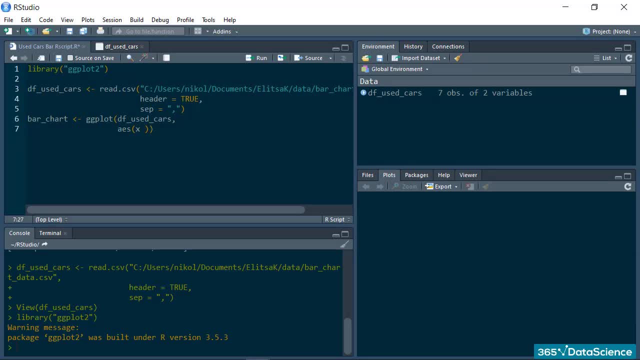 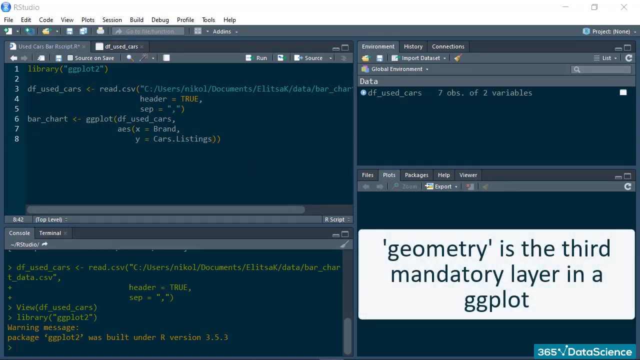 We want to display the number of car advertisements by brand. Therefore, on the x-axis we'll have brand and on the y-axis we'll select cars listings. The last mandatory step for completing the plot is to specify the geometry. The geometry shows the shape in which we'll be displaying our data. 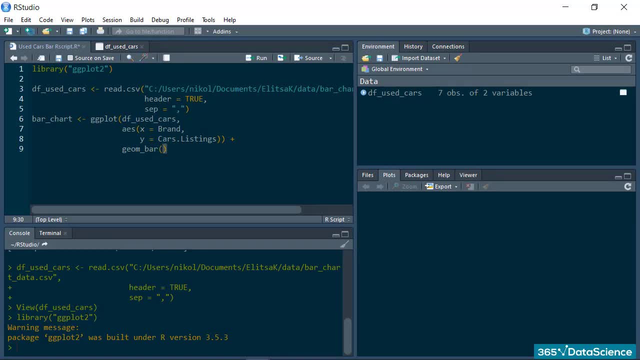 We'll be creating a bar chart. Therefore, we'll opt for the geomeBar. Inside the brackets we'll need to indicate a y aesthetic. We'll use stat equals identity specifying. we want the actual y values plotted. The reason here is that geometry bars are 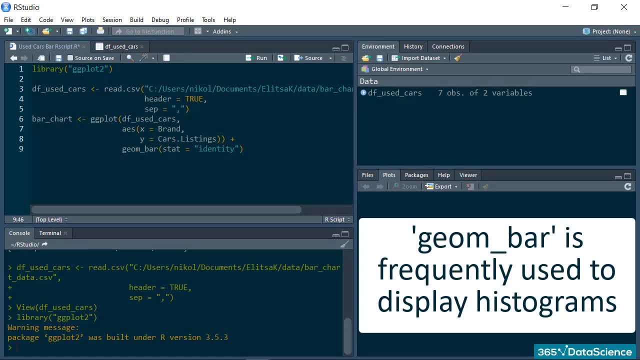 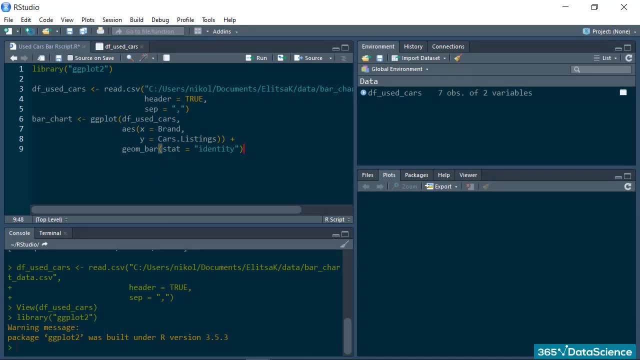 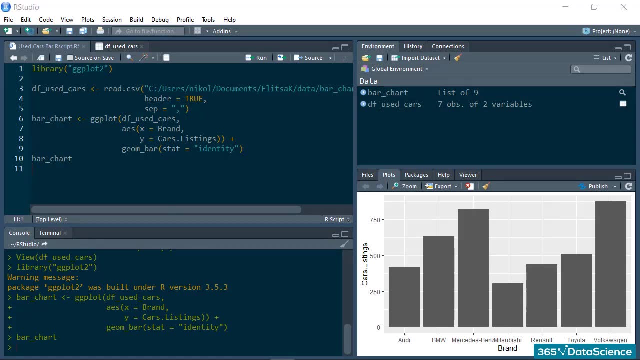 frequently used to display histograms which map the distribution of a certain variable. That's why we require the extra parameter. Okay, let's run the code and examine the result. There you have it, our first bar plot. On the x-axis we have the brand, while on 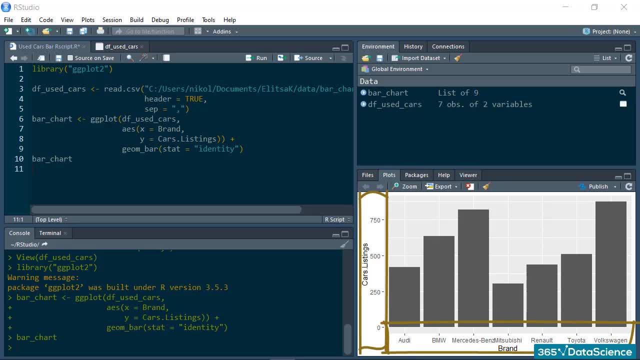 the y-axis the number of cars sold, And that's all you need to create a bar chart. But don't go packing up just yet. we still have work to do. For the remainder of the lecture, we'll concentrate on formatting our chart and improving. 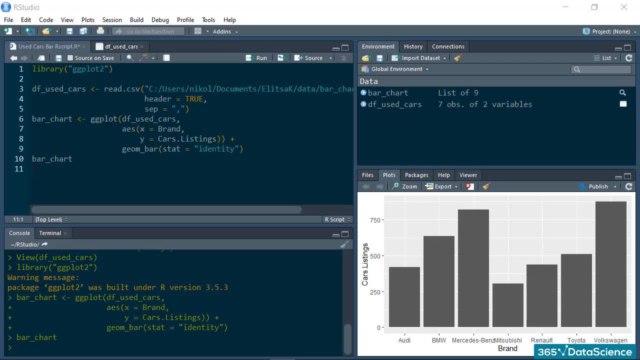 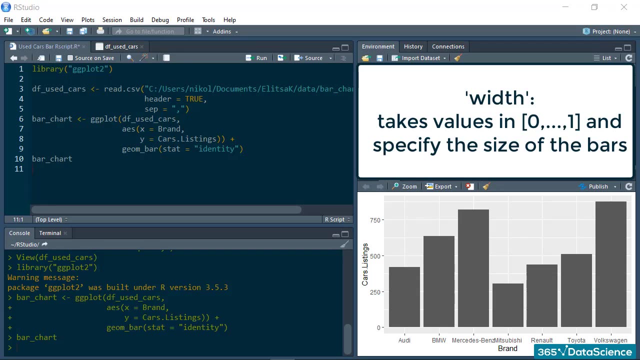 its appearance. It will also give us the chance to get better acquainted with some of the remaining ggplot layers. First, we can decide on the size of the bars themselves. The size is specified using width. for the width of each column, It can take values from 0 to 1.. If we select 1, there 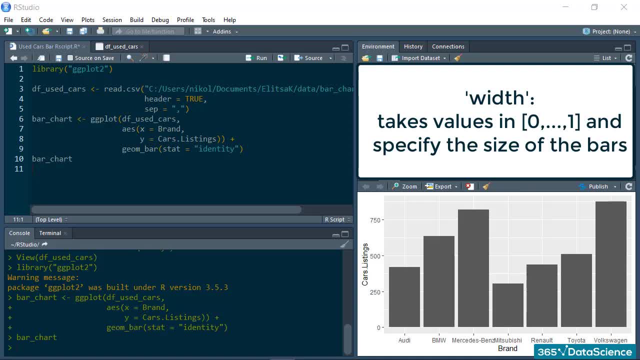 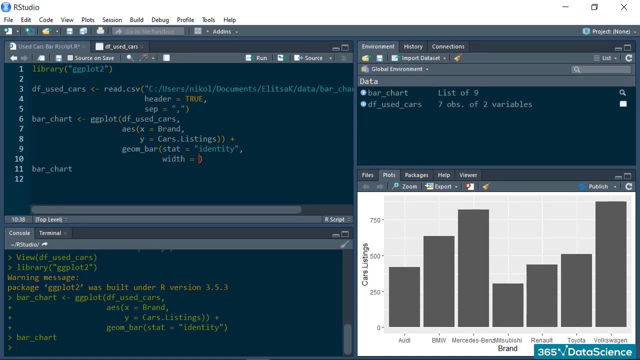 will be no space left between the bars, making it look like a histogram. We're creating a bar chart right now, so let's select 0.8, leaving us with some space between the individual bars, without spacing them out too much. 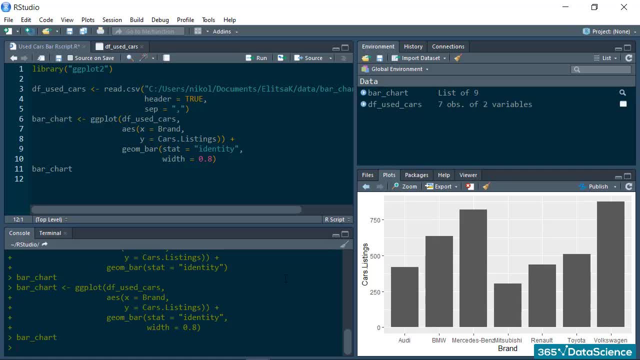 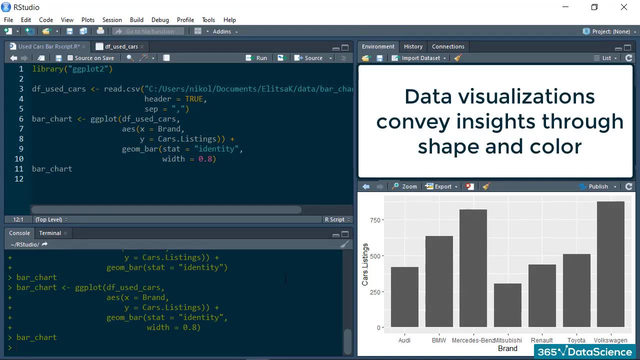 Okay, what comes next? Generally, data visualizations convey insights through shape and color. However, While the shape is somewhat restricted by the nature of the data, the color is up to us. Nonetheless, choosing a color for our visualizations is of utmost importance and should be thought through carefully. 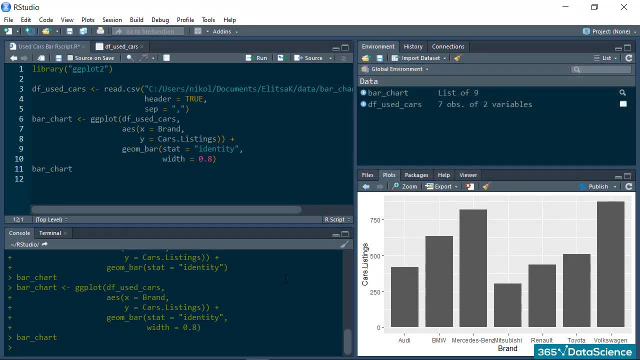 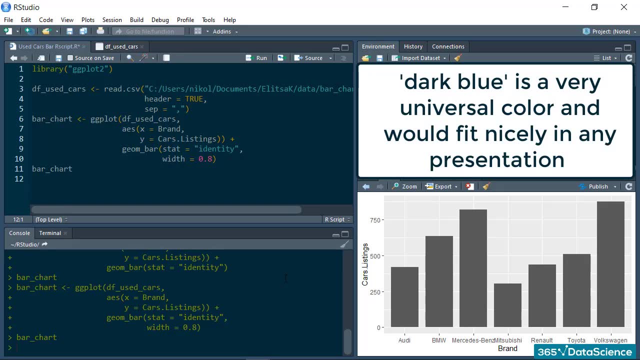 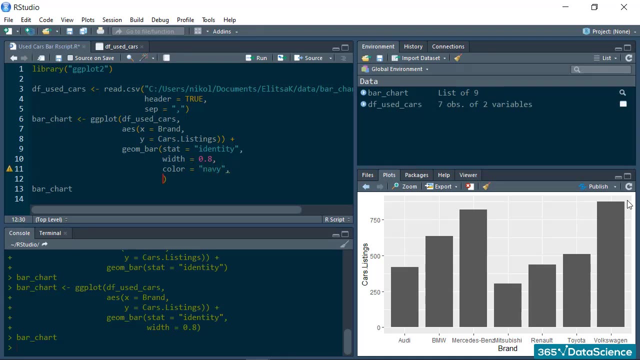 So let's go ahead and choose a nice color for our bars. For this chart, we'll settle on a dark blue color. It is a very universal color and would fit nicely in any presentation. We'll include it as a string for both the fill and border of our bars. 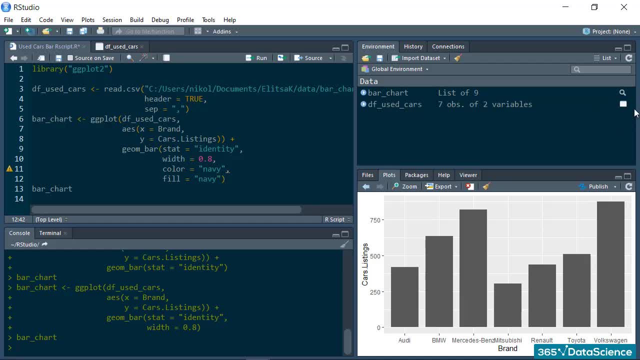 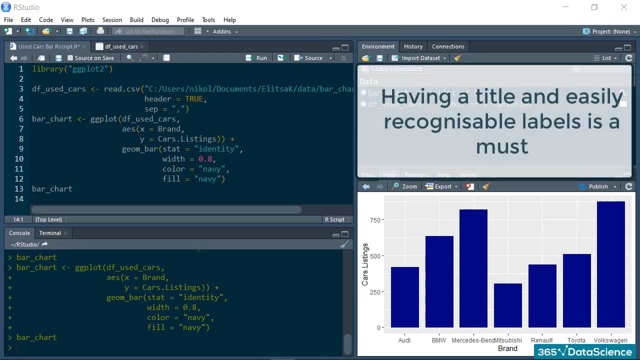 You can find a list of available options with the resources in this lecture or online. While colors are very important, having a title and easily recognizable labels is arguably even more important. For the title, we'll add another element called ggtitle. As I start typing it out, 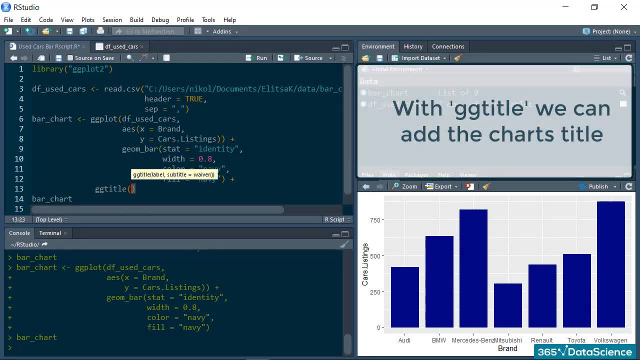 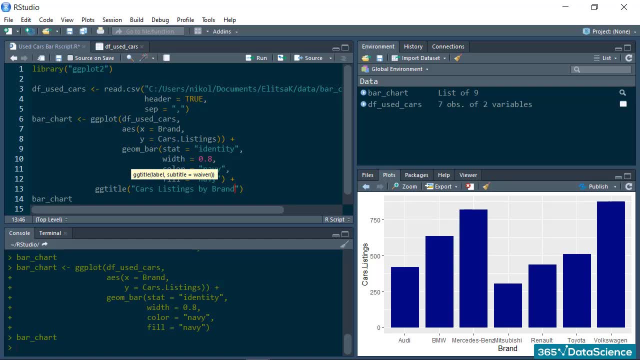 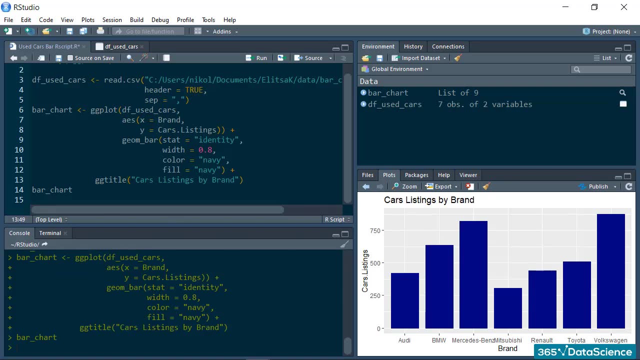 RStudio is already there. It's already suggesting it. What would be a good title- Cars Listings by Brand- has a nice ring to it, doesn't it? Good job, Alright. what's next? Well, since we changed the color of our bars, the gray background isn't as fitting any longer. 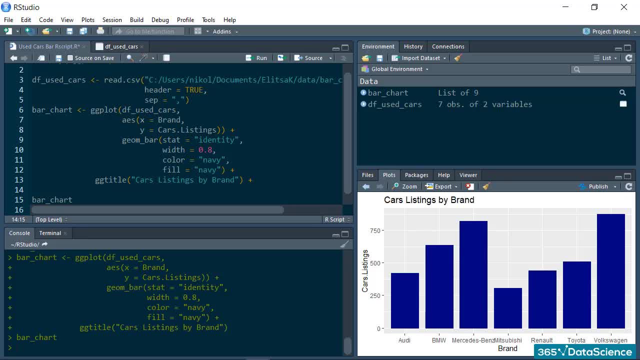 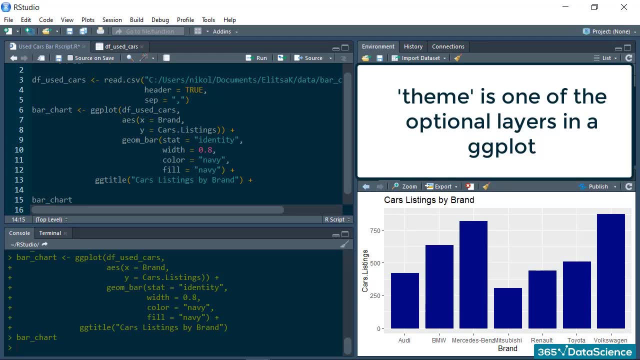 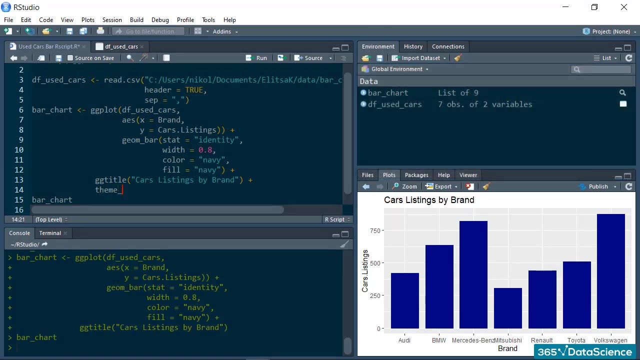 No worries, we can fix this by assigning a different theme. Recall that Theme was one of the optional layers in a ggplot. Though optional, we'll be using it often because the appearance and style of our charts matter. So let's add a theme element to our chart and select a classic theme which has a white background. 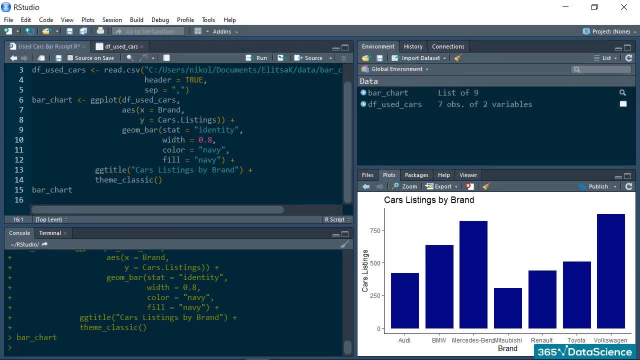 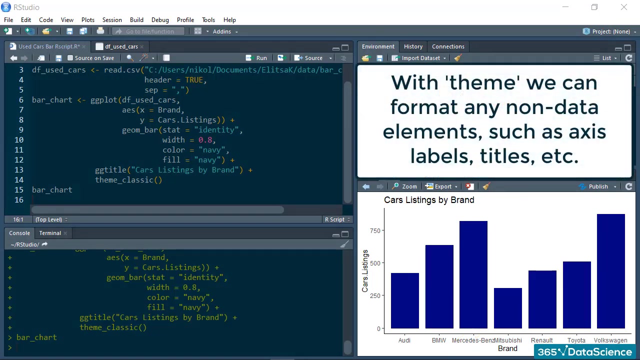 Very nice. The next item on the list is formatting the axis. Currently, the labels on the x-axis are overlapping in parts, which, of course, isn't ideal. However, we can amend it and increase space by rotating the labels. As with any styling choice, this is part of the theme department. 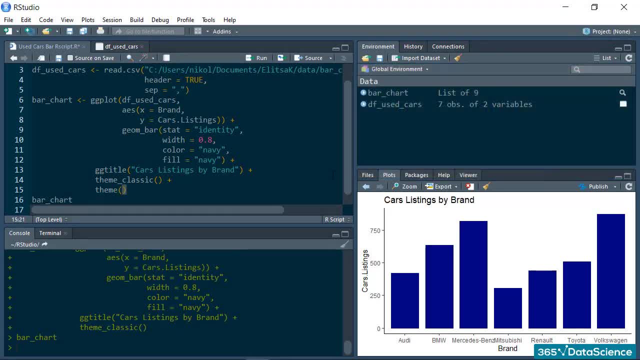 Let's add a theme element where we'll include a text parameter for the x-axis. We'll give it the text labels with element text and in brackets, specify a rotation angle of 45.. Lastly, we also add a height justification of 1,. 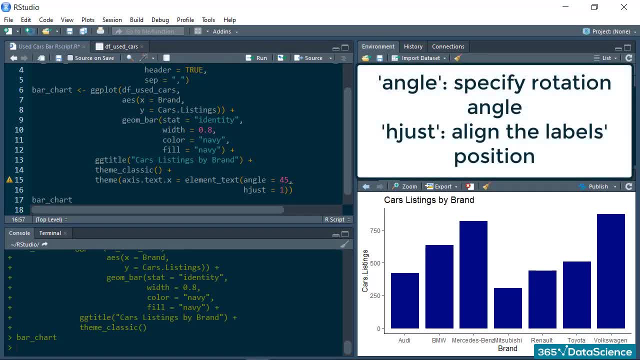 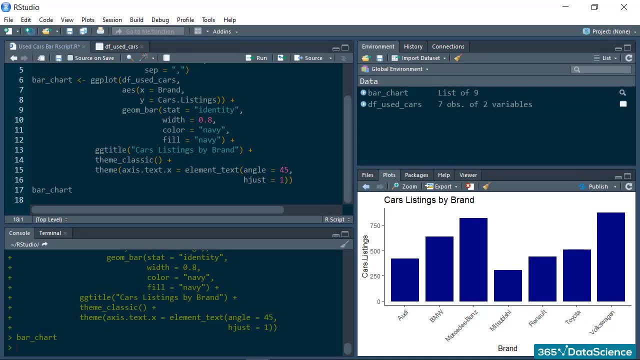 just so the labels don't shift after the rotation. I'm excited to see the result: Superb. All labels can be clearly distinguished. Lastly, we don't need the label on the x-axis for this graph, as it is evident from our labels that we are displaying car brands. 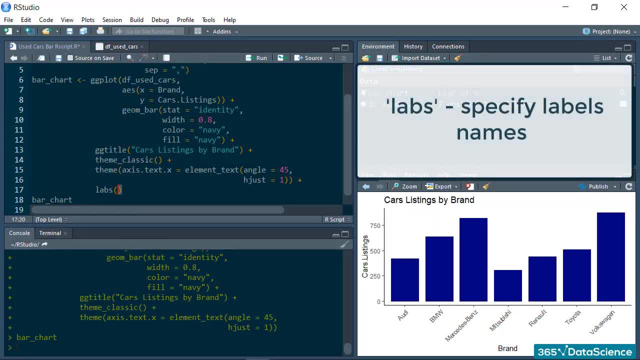 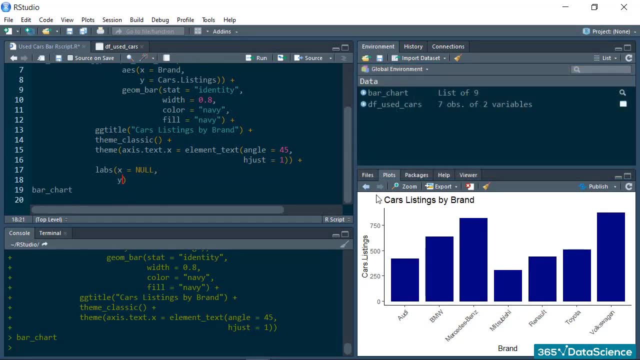 We'll add a labs function, short for labels, and say that x is null, which will remove the label on the x-axis. As for y, let's set the label to Number of Listing. Okay, amazing, We have successfully made our first bar plot in R. 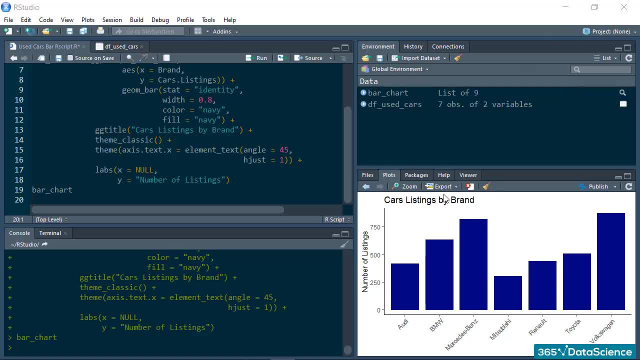 A great feature of RStudio allows you to export the generated image. You just click on Export and select Image or PDF. Or you could directly copy this image to your clipboard and paste it in a dictionary. And paste it in a different document, like a PowerPoint presentation, for instance. 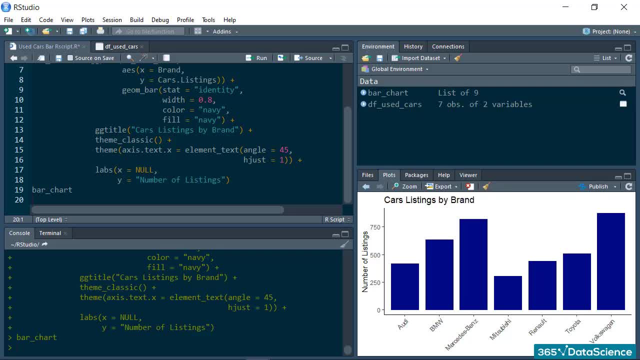 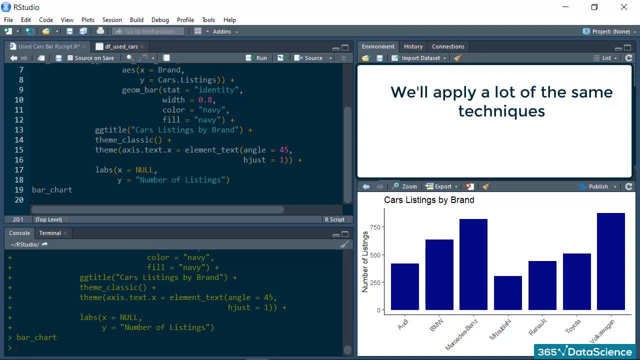 Alright. This concludes our lecture on bar charts in R. Moving forward, we'll apply a lot of the techniques we saw here in this introductory lecture, But we'll also learn some new tricks for making quality charts, And I for one can't wait. 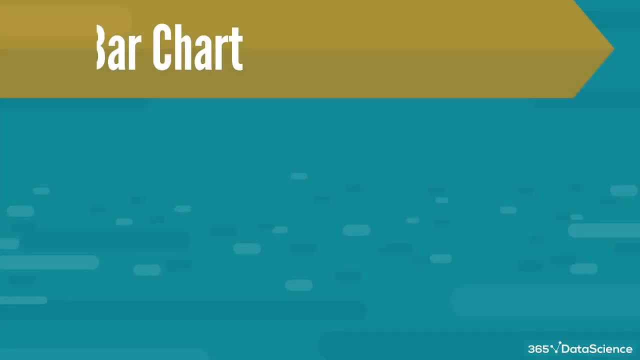 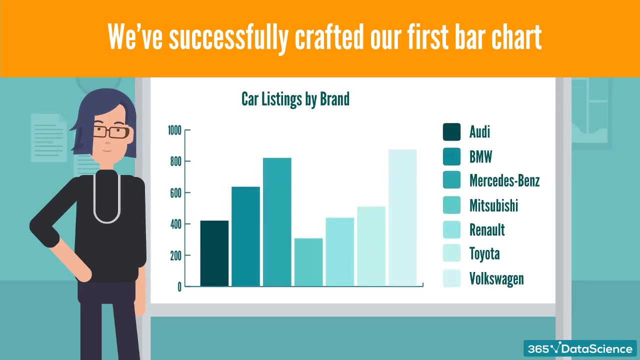 We've successfully crafted our first bar chart and are confident it would serve us well during a presentation. After all, we've done all the necessary steps to ensure it is as professional as possible. On top of that, your audience can easily tell: the most widespread brand for used cars is Volkswagen. 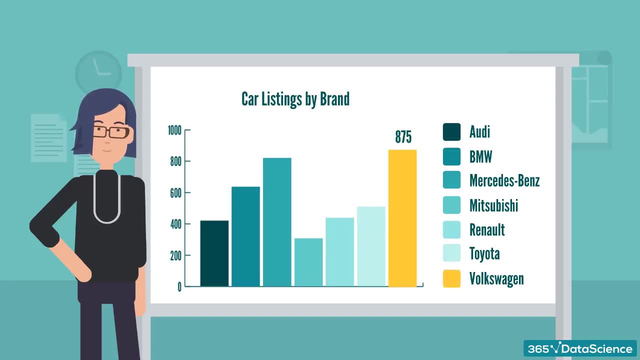 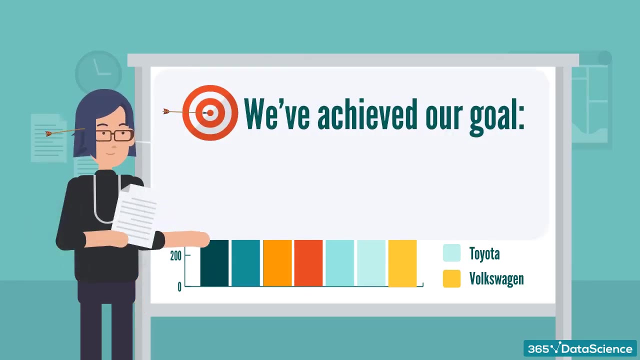 There is a total of 875 units from Volkswagen, followed closely by Mercedes with 820.. Mitsubishi was the least popular, with approximately a third of the listings of the frontrunner. Excellent, We've achieved what we set out to do: Tell the story of this dataset with the aid of a bar chart. 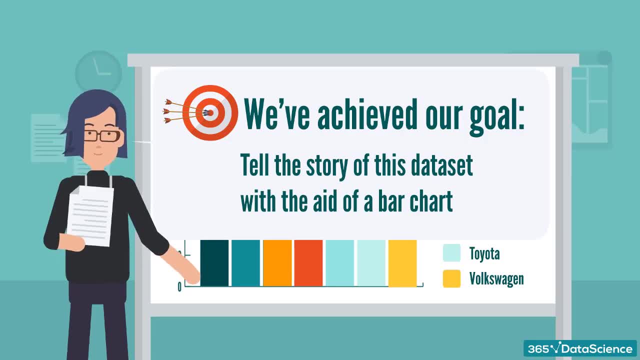 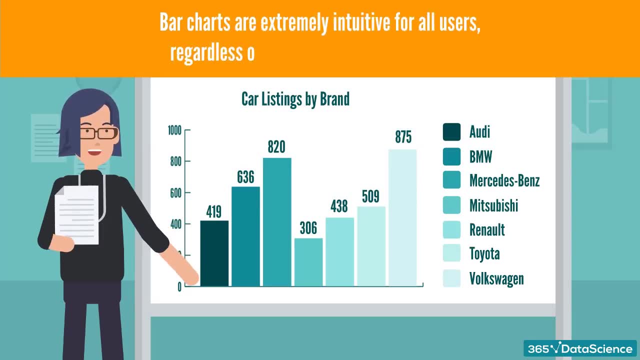 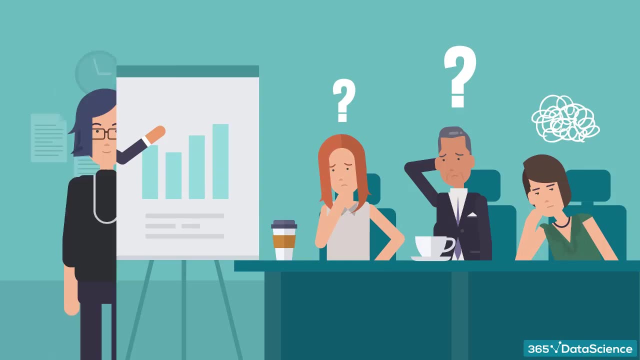 There isn't much left for us to comment on this visualization. That is one of the greatest strengths of a bar chart: It is extremely intuitive for all users, regardless of their professional background. But not all bar charts are created equal, So it's worth taking a second to explore what can go wrong when making a bar chart. Let's look at the following chart depicting the average house prices in pounds for the years 1998 and 1999.. Visually it appears from the year 1998 to 1999, there has been a threefold increase in house prices.